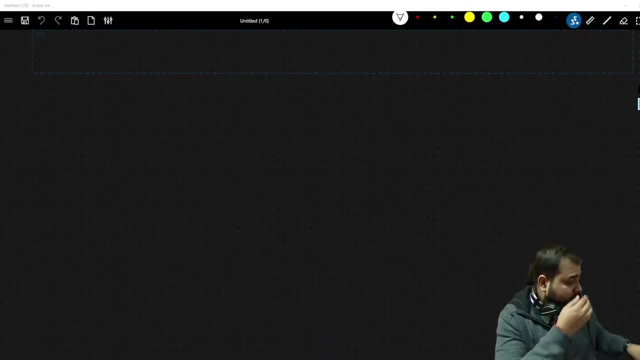 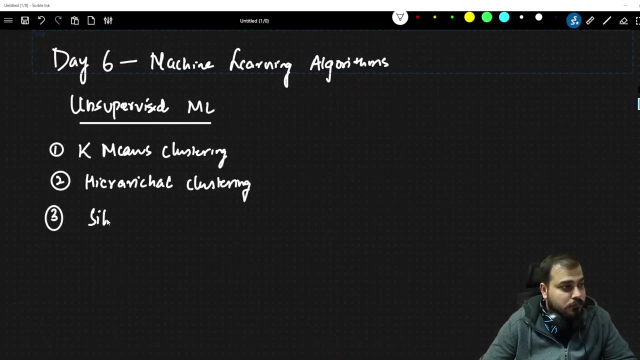 Thank you, Hello guys, I hope everybody is able to hear me out. Hello guys, I hope everybody is able to hear me out. Hello guys, I hope everybody is able to hear me out. So till now, we have discussed about lot of supervised machine learning algorithms and in those specific algorithms we have already discussed about different, different algorithms like linear logistic. then we discussed about KNN- KN nearest neighbor. we discussed about decision tree, AdaBoost. you know XGBoost. I told you to basically check it from my one of my YouTube videos because, again, I am trying to cover it within one and a half hours. so, whatever is possible, I will definitely try to cover it up. 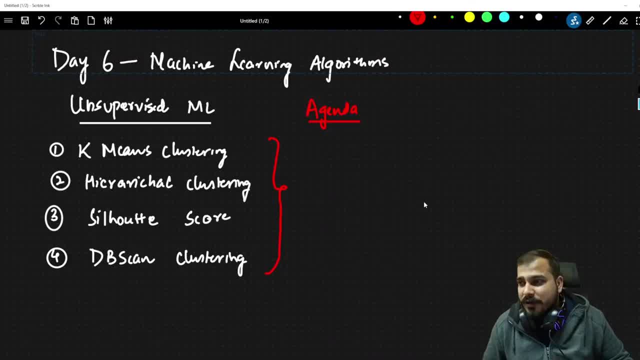 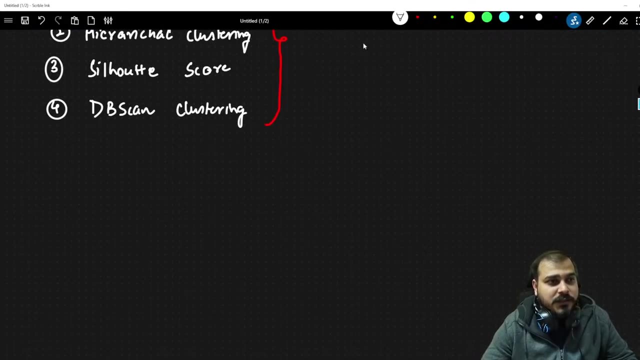 Okay, SVM, SVR. I have already uploaded in one of my video there, because I don't know whether we will be able to cover everything or not, but tomorrow's whatever is missed, I will try to cover those things also. Okay, so let's start. the first algorithm that we are probably going to discuss today is something called as K means clustering. 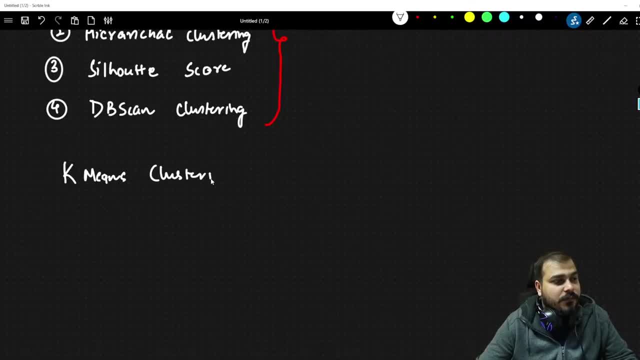 K means clustering, and this is a kind of unsupervised machine learning. Okay, Now, always remember, Remember, unsupervised machine learning basically means that the one and the most important thing is that in unsupervised machine learning, in unsupervised ML, you don't have any specific output. 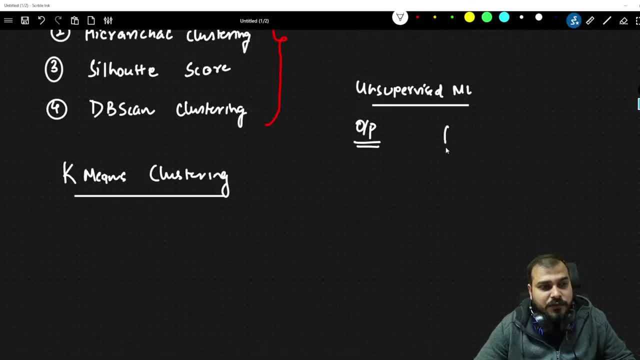 Okay, so you don't have any specific output. So suppose you have feature one and feature two, and suppose you have data's different, different data, you know, and based on this data, what we do, we basically try to create clusters. Okay, So this cluster basically says: what are the similar kind of data? 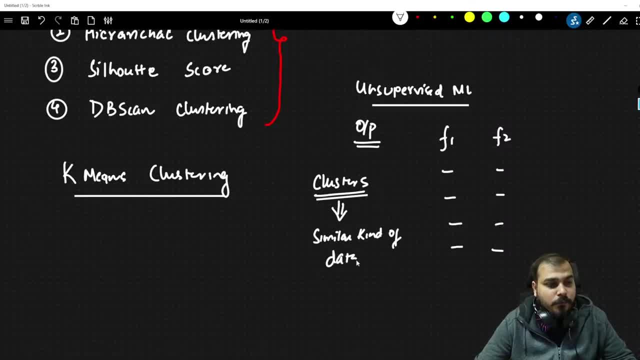 Okay, Similar kind of data. So this is what we basically do from clustering and there are various techniques, like K means. it is hierarchical clustering and all. So first of all, we try to understand about K means and how does it specifically work. It's simple. 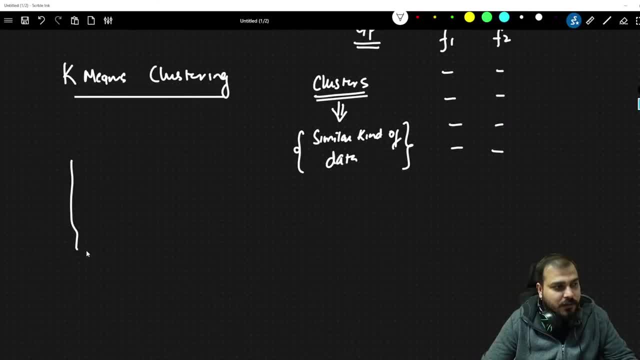 Suppose you have a data points like this. Let's say that you have a data points. Suppose you have Some data points like this: Okay, let's say that this is your F1 feature, F2 feature and based on this- in two dimensional probably, I will be plotting this points and suppose this is my another points. 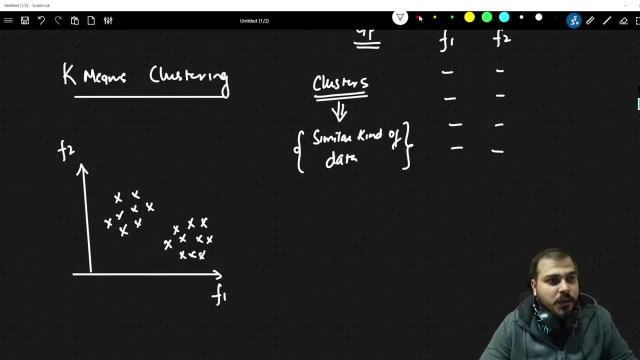 So our main purpose is basically to cluster together in different, different groups. Okay, so this will be my one group and probably the other group will be this group. right, so two groups, because obviously you can see from this clusters, Here you have two similar kind of data which is basically grouped together. right, this is my cluster one. 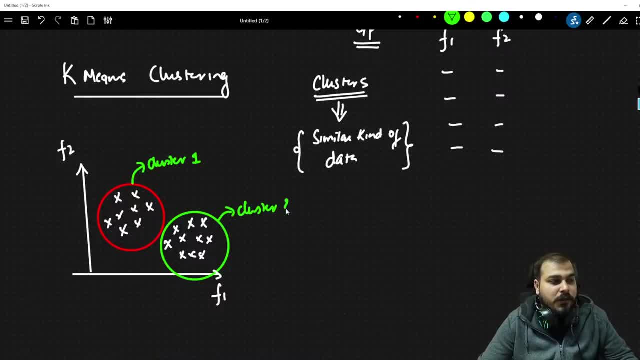 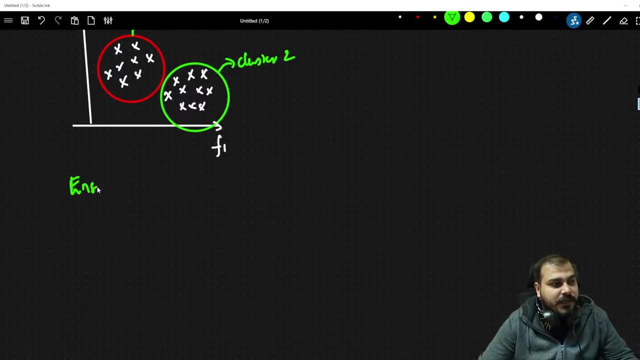 And this is my cluster two. Okay, let me talk about this and why specifically. it would be very much useful. Then we'll try to understand about math intuition also. now, always understand, guys. where does clustering gets used? Okay, In most of the ensemble techniques. I told you about custom ensemble technique, right? 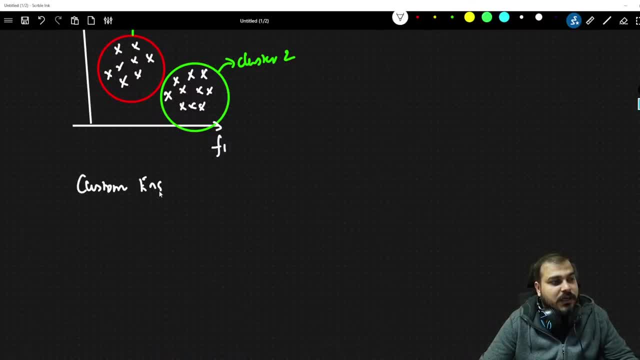 So custom ensemble, Ensemble, Ensemble, ensemble techniques In custom ensemble techniques. you know, whenever we are probably creating a model, first of all on our data set, what we do is that we create clusters. So suppose this is my data set during my model creation, the first algorithm we will probably apply will be clustering algorithm. 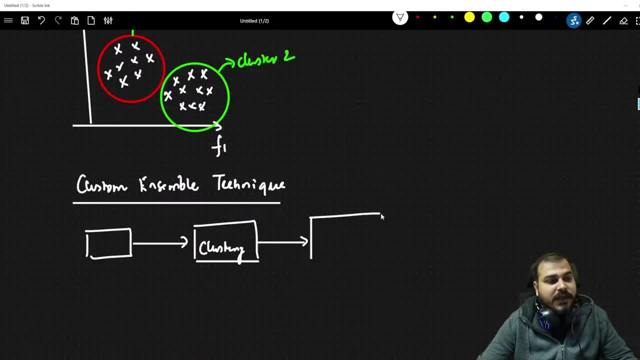 and after that it is obviously good that we can apply regression or classification problem. Suppose, in this clustering I have two or three groups. let's say that I have two or three groups over here. for each group we can apply a separate supervised machine learning algorithm if we know. 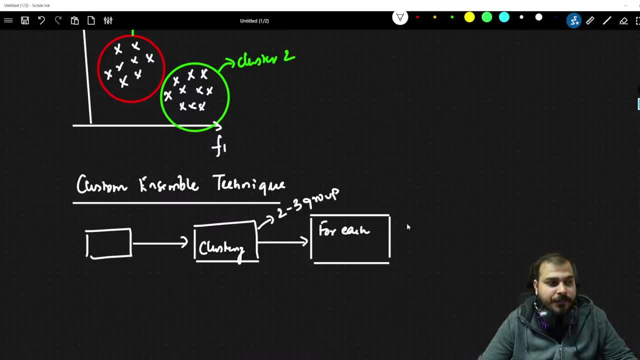 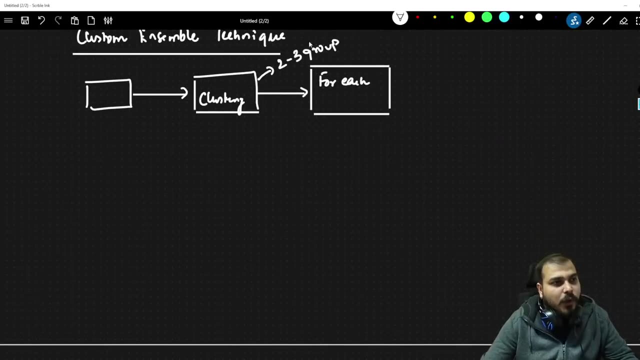 the specific output that we really want to take ahead. I'll talk about this and give you some of the examples as I go ahead. Now let's go ahead and focus more on understanding. how does K-means clustering algorithm work? So, so, so, so, let's go over here. The word K-means has this K value. This K are nothing but this K, basically. 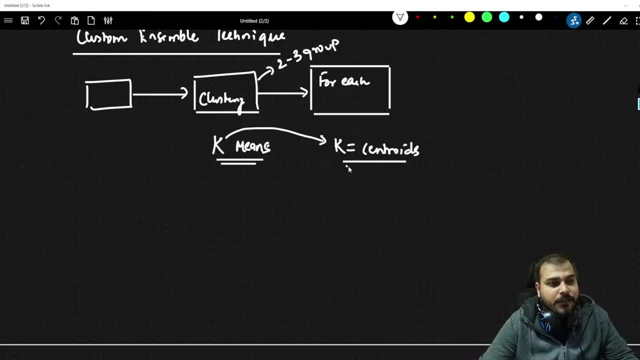 means centroids. K basically means centroids. So suppose, if I have a data set which looks like this, which looks like this, Let's say that this is my data set. Now, over here, just by seeing the data set, what are the possible groups you think? Definitely you'll be saying K is. 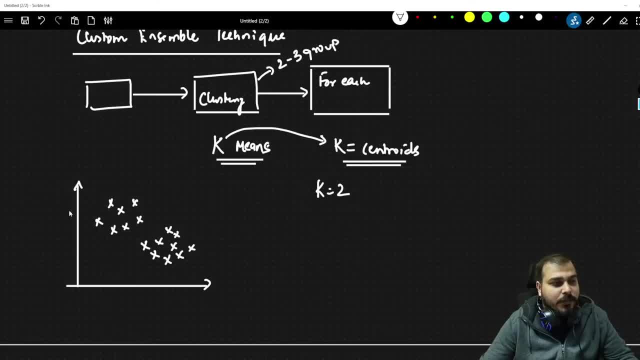 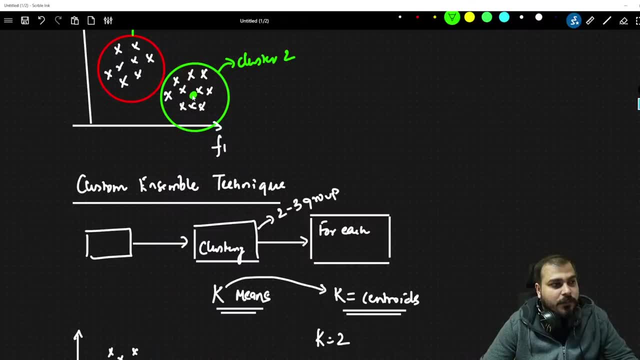 equal to 2.. So when you say K is equal to 2, that basically means you will be able to get two groups like this and each and every group will be having a centroid, a centroid point. Here also there will be a centroid point, OK. So this centroid will determine. basically this is a separate group over here. 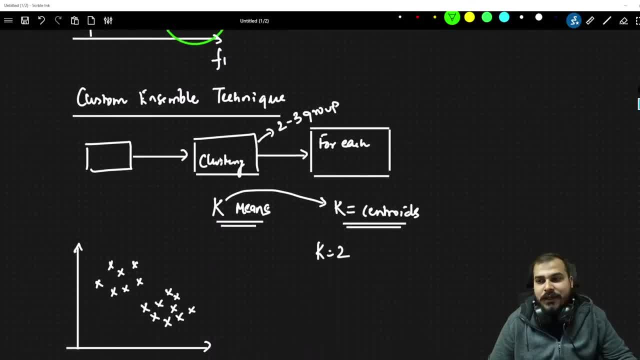 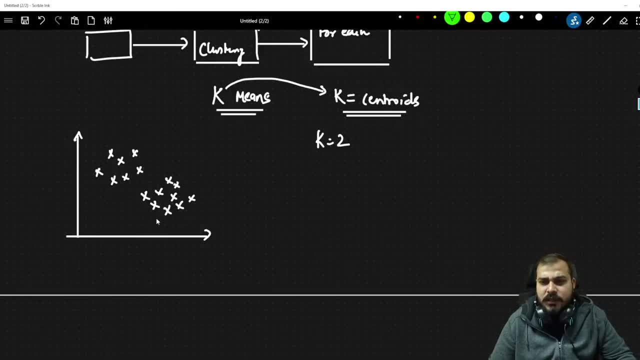 This is a separate group over here. OK, So over here here you can definitely say that, fine, this is two groups. But how do we come to a conclusion that there is only two groups? OK, We cannot just directly say that, OK, we'll try to, just by seeing the data, because your data will be having a high 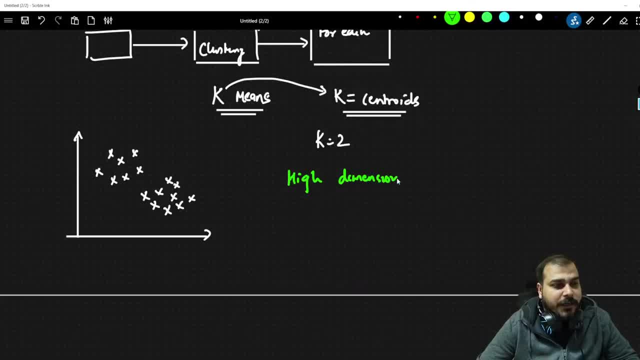 dimension data. Right Right now I'm just showing your two dimension data, But for a high dimension data, definitely you'll not be able to see the data points how it is plotted. So how do you come to a conclusion that only two groups are there? So for this, there is some steps that we basically perform. 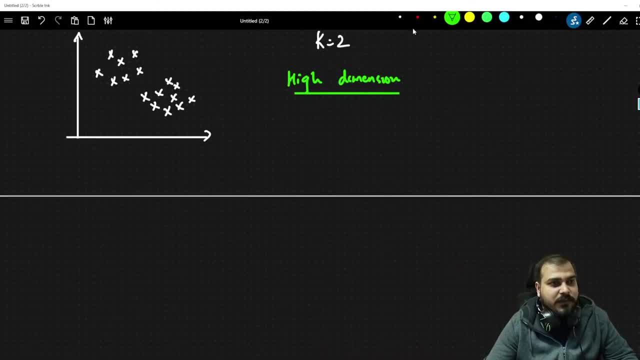 in K-means. OK, The first step, What is the first step? Let's write down the first step. The first step is that we try with different K values. We try with different K values, OK, And which is the suitable K value? K is nothing but centroid, OK. 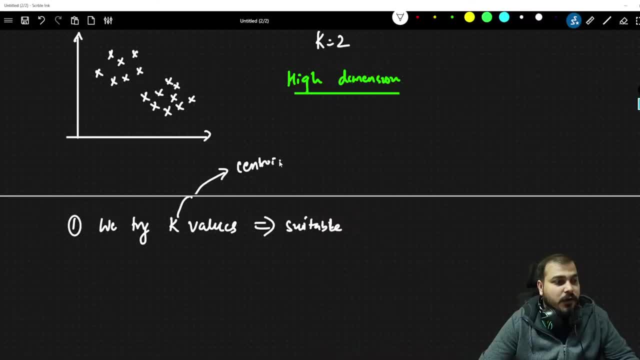 It is nothing but centroid. We try with different, different centroid. OK, In this particular case, Let's say that I have this particular data point, and I actually start with. K is equal to 1 or 2 or 3, anyone you want. 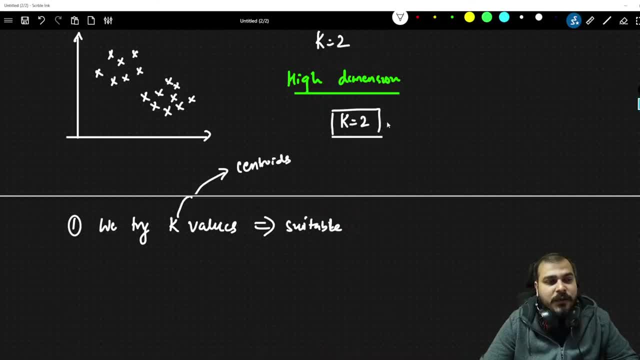 Let's say that I'm going to start with. K is equal to 2.. How to come up with this? K Is equal to 2 as a perfect value, That I'll talk about it. We need to know there is a concept which is called as within cluster sum of square. 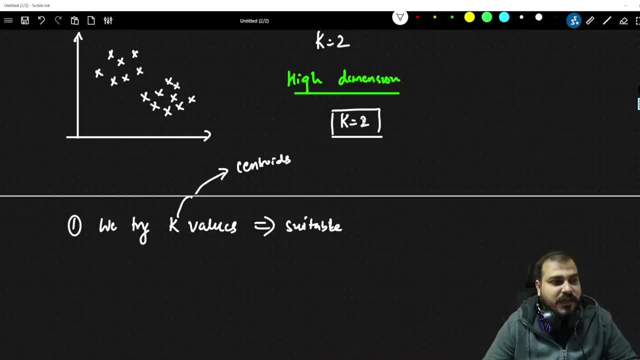 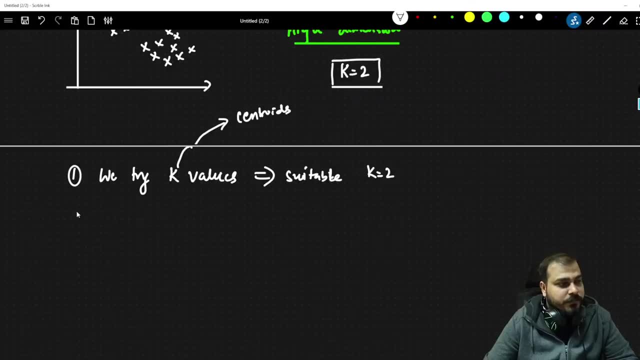 So when we try different K values, let's say that for K is equal to 2, what will happen? The first step: We select a, We try K values, So let's say that we are considering K is equal to 2.. The second step is that we initialize, We initialize, We initialize. 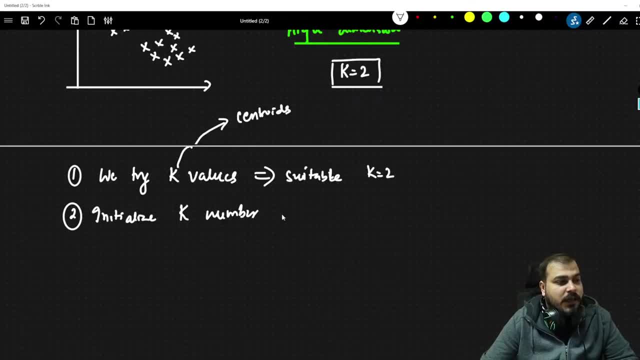 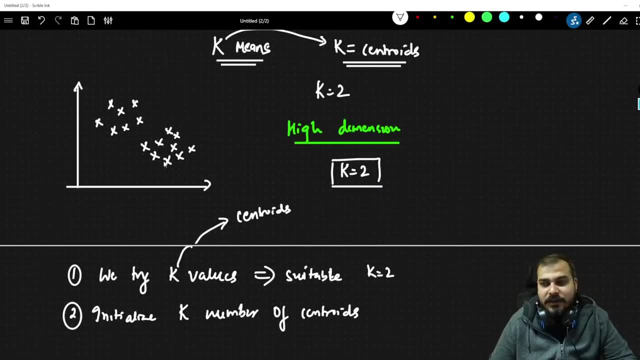 K number of centroids. K number of centroids. now, in this particular case, I know my K value is 2. So we will be initializing randomly. Let's say that K is equal to 2. So what we can actually do, let's say that this is: 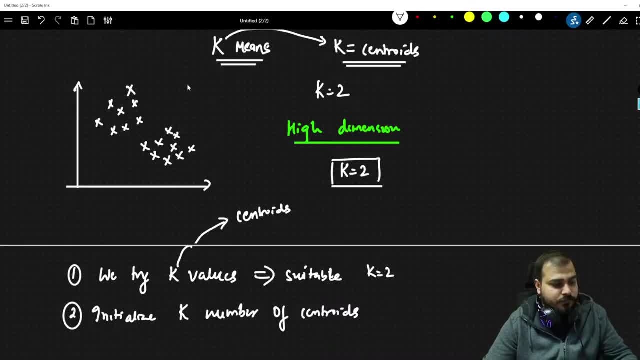 This is my one centroid. This is my one centroid. I will. I'll put it in another color, So this will be my one centroid And let's say that this is my another centroid. So I've initialized two centroids randomly in this space. OK, 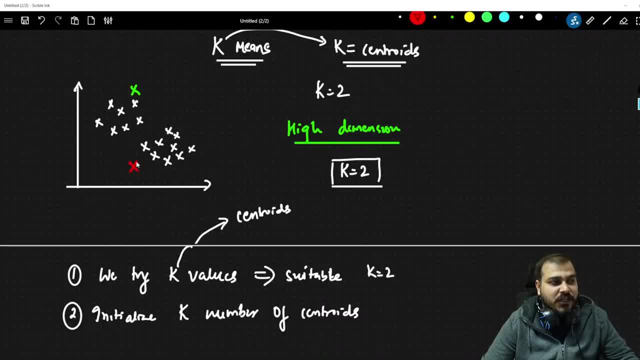 Now, after this particular centroid, What we have to do is that, after Initializing this centroid, what we have to do is that we have to basically find out which points are near to this centroid, and which points are near to this centroid Now, in order to find out. it is a very 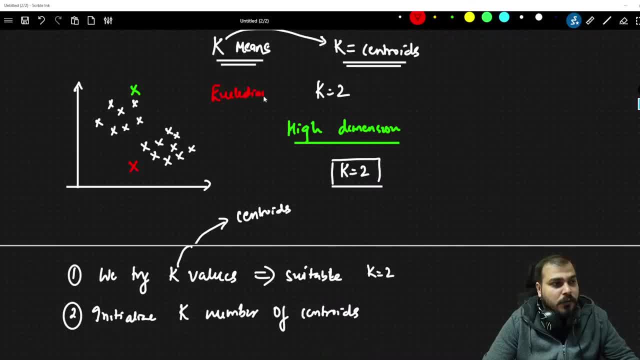 easy step. we can basically use Euclidean distance, okay, to find out the distance between the points in an easy way. if I really want to show you that you know, like, how many points I want to, in an easy way, what I can do, I can basically draw a straight line over here. let's say that. 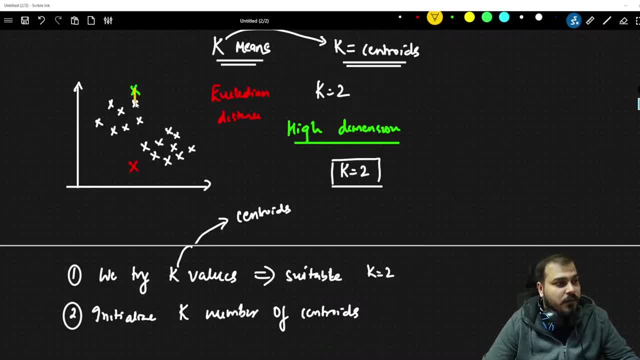 I'm drawing a straight line over here in another color. okay, I can draw a straight line and I can also draw one parallel line like this. So this basically indicates that whichever points you see over here, suppose, if I draw a straight line in between all these points, you will be able to. 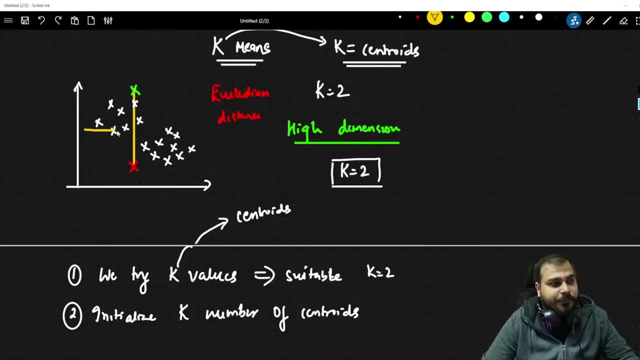 see that. let's say that I'm drawing one more parallel line which is intersecting together. So from this you can definitely find out. let's say that these are all my points that are nearer to this green line, green point. okay, so what i am actually going to do in this particular case? all these points. 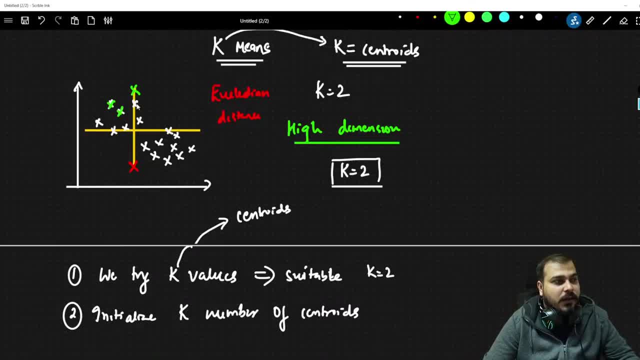 that you are seeing near the green, it will become green color. so that basically means this is basically nearer to this centroid, okay. and whichever points are nearer to this particular point, that will become red point. so that basically means this belongs to this group, okay, this belongs to this group, okay. so i hope everybody is clear till here. then what will happen is that this: 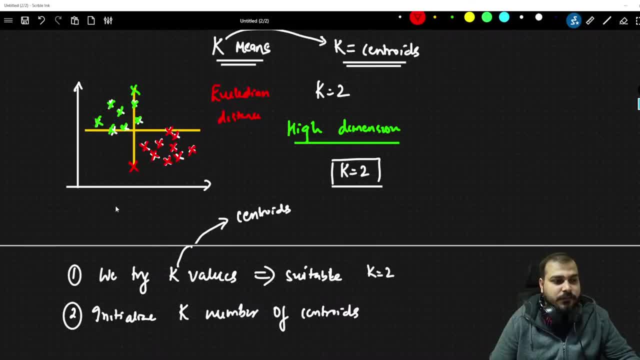 summation of all the values. then we initialize the k number of inter centroids. that is done. then we try to calculate a distance, we try to find out which all points is nearer to the centroid. let's say that this is my one centroid, this is my another centroid and we have seen that. okay. 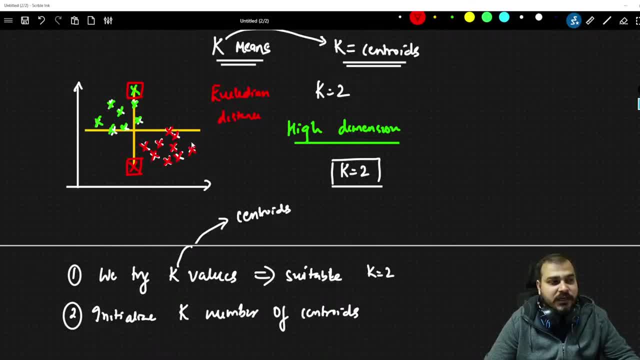 these all points belong to this centroid, it is near to this particular centroid, so this is becoming red, okay. so this is based on the shortest distance, and here it is becoming green. okay, now the next step. let's see what is the next step after this. so i am going to remove this team. okay, now the next step will be. 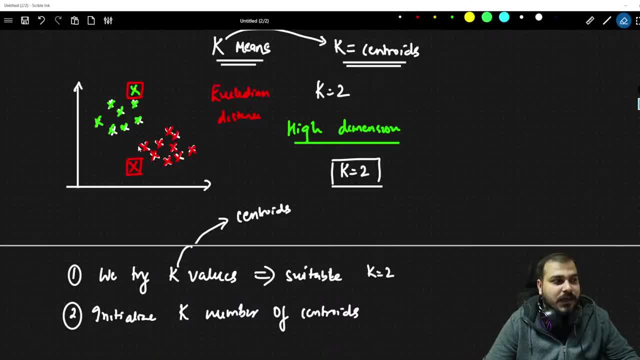 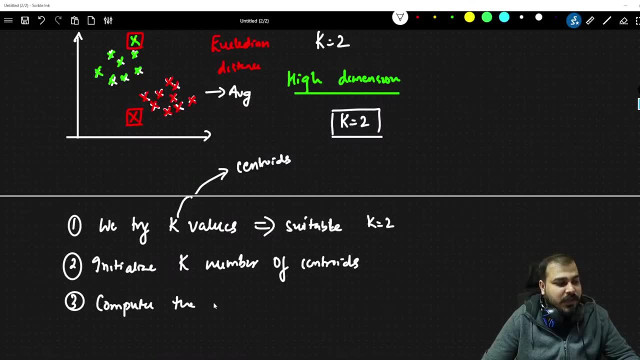 that the entire points, that is in red color. okay, all the average will be taken. so here again, the average will be taken. now, third step: here i am going to write here we are going to compute the average. the reason we compute the average is that we are going to compute the average because we are 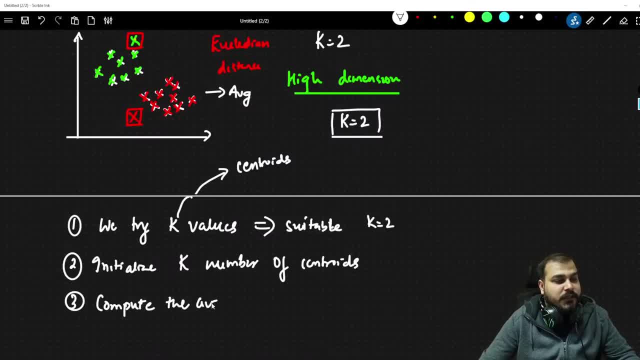 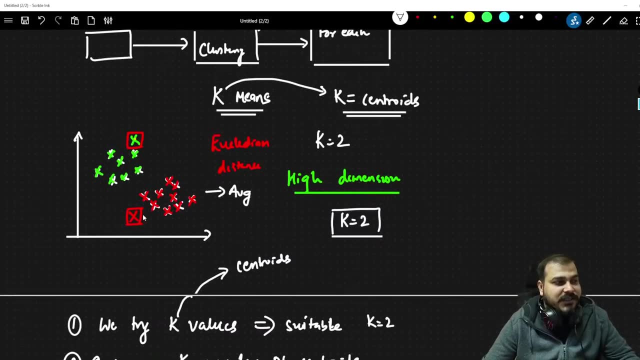 because we need to update the centroid. so compute the average to update centroid, to update centroids. okay, so here you will be able to see that what i am actually doing as soon as we compute the average. this centroid is going to move to some other location. so what location it will move? it will obviously become somewhere in center. 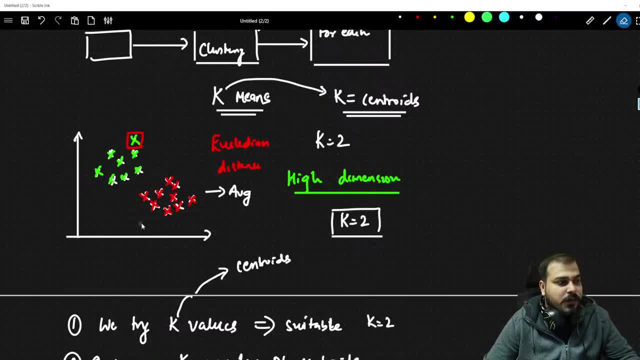 so here, now i am going to rub this, rub this, and now my new centroid will be this point where i am actually going to draw like this. let's say, this is my new centroid now. similarly, this thing will happen with respect to the green color. okay, so with respect to the green color also, it. 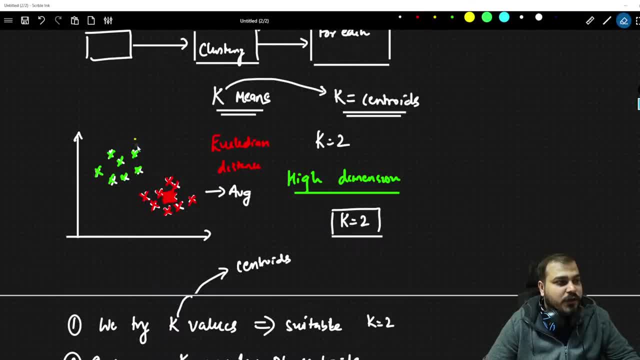 will happen and this green will also get updated. so i am going to rub this and this will be my new green point, which will get updated over here, over here. okay, then again, what will happen? again, the distance will be calculated and again, a perpendicular line will be calculated. 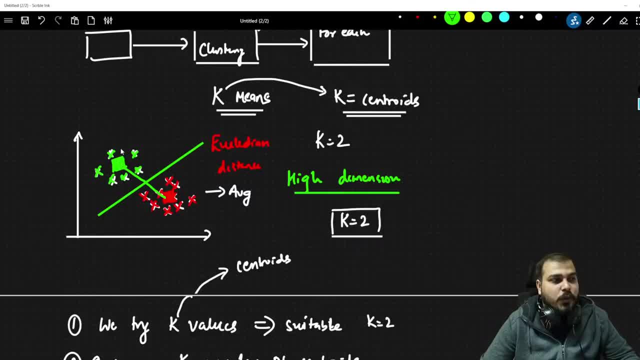 here you can see that now all the points are towards there. okay, again the centroid based on this particular distance. again it will be calculated, and here you can see that all the points are in its own location. so here now no update will actually happen. let's say that there was one point which was red color over here. 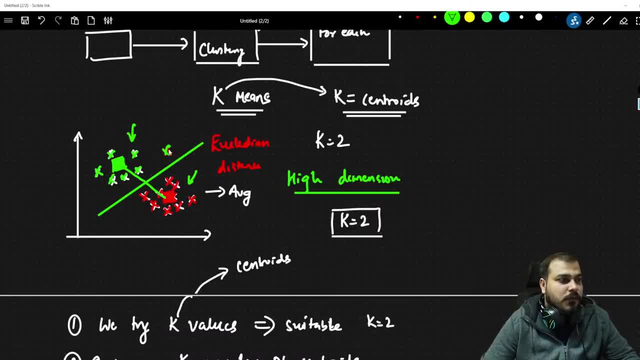 then this would have become green color. okay, but since the updation has happened perfectly, we are not going to update it and we are not going to update the centroid right. so now you can understand that. yes, now we have actually got the perfect centroid and now this will be. 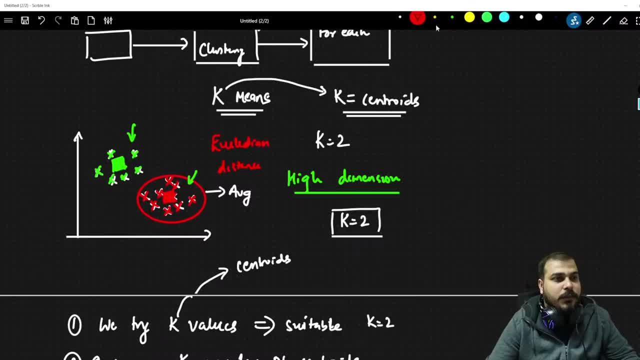 considered as one group and this will be basically considered as the another group. sorry, this will be considered as my another group. okay, it will not intersect, but right, by default, here intersection is happening. harsh saw, please check your internet. if the screen is blurry, okay, because of your internet. 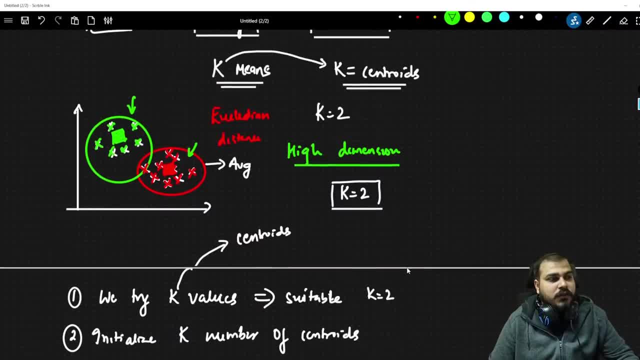 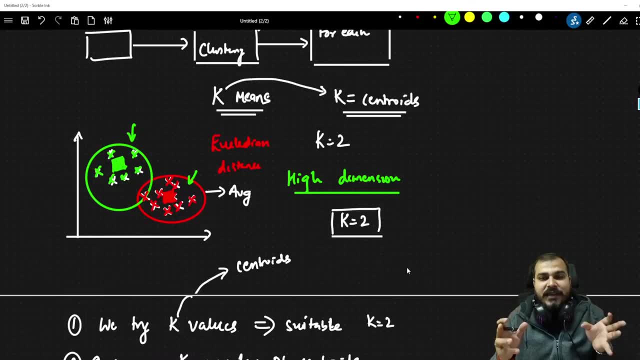 it is taking in different pixels, okay, so i hope everybody is understood the steps that you have actually followed in initializing the centroids, in updating the centroids and in updating the points. is it clear? everybody, with respect to k, means yes, everybody. everybody is it clear? everybody is it clear? so what we are trying, 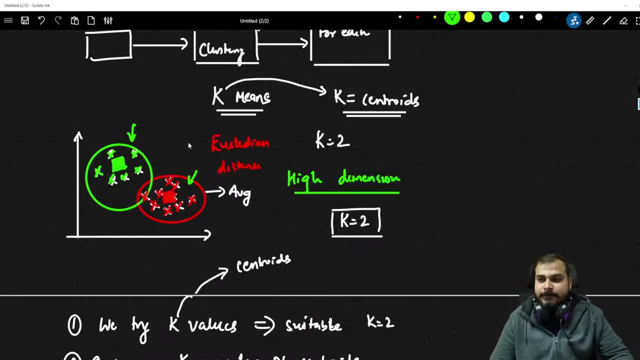 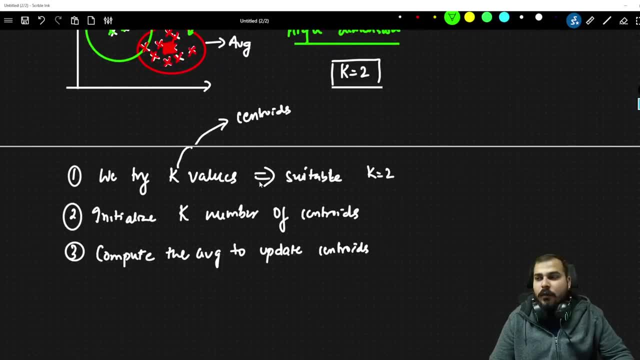 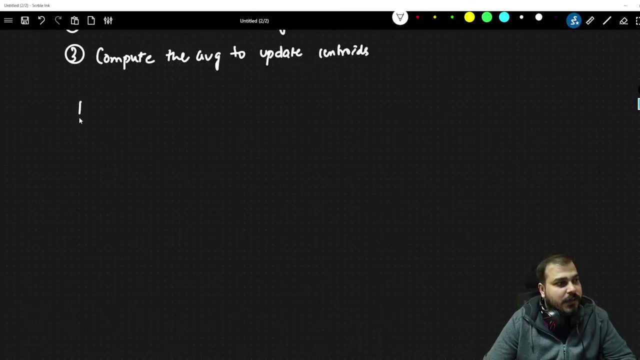 to do in this? k means clustering. yes, yeah, everybody. perfect, okay, now let's discuss about one point: how do we decide this k value? okay, how do we decide this k value? so for deciding the k value, there is a concept which is called as elbow method. okay, so here i'm going to basically define my elbow method now. elbow method says: 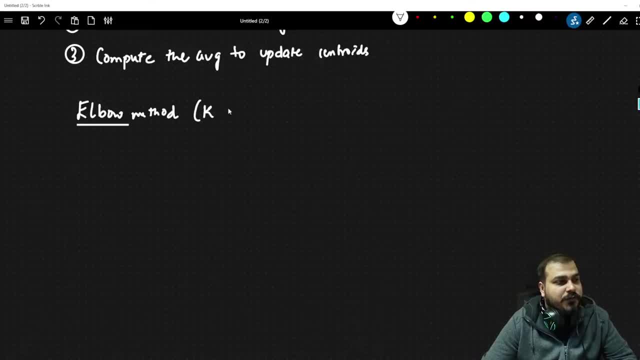 something very much important, because it's a concept which is called elbow method. okay, this will actually help us to find out what is the optimized k value: whether the k value should be 2, whether the k value is going to be 3, whether the k value is going to become 4. okay and always. 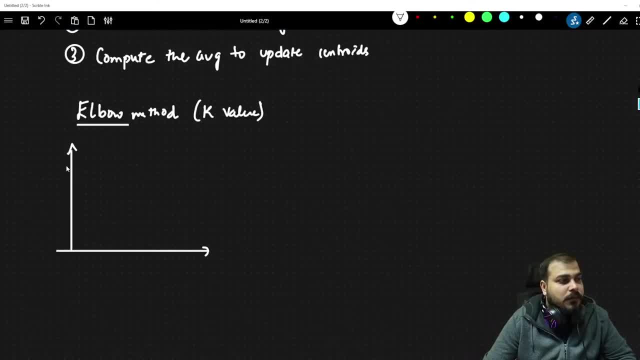 understand. suppose this is my data set. suppose this is my data set initially. let's say that i have my data points like this. we cannot go ahead and directly say, say that, okay, k is equal to 2 is going to work. so obviously we are going to go with iteration, for i is equal to probably 1 to 10. 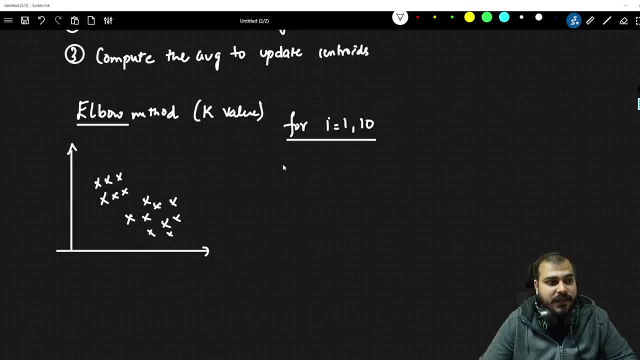 i'm going to move towards iteration from 1 to 10. let's say so: for every iteration, we will construct a graph with respect to k value and with respect to something called as wcss. now, what is this wcss? wcss basically means within cluster, within cluster. sum of square. 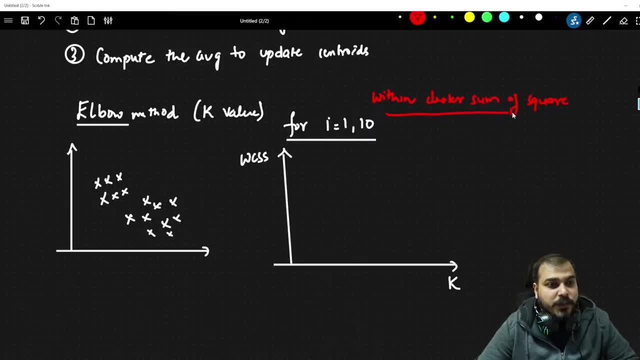 okay, okay, okay, this is the meaning of wcss within cluster sum of square. okay, now let's say that initially we start with one centroid. so one centroid, let's say it is initialized here. okay, one centroid is basically initialized here if we go and compute the distance. 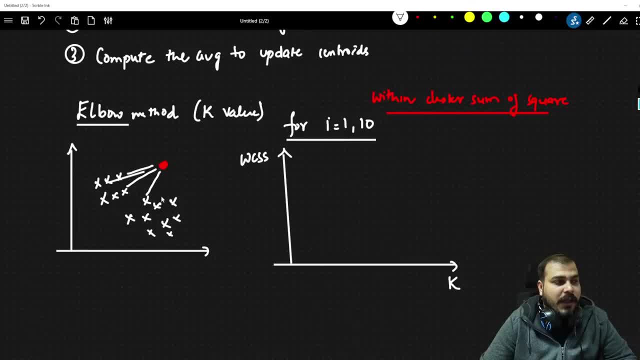 between each and every points to the centroid. and if we try to find out the distance, will the distance value be greater or it will be smaller? tell me. will the value be smaller or greater? one, two, three, four, five, six? will it be smaller or greater, tell me, if we try to, 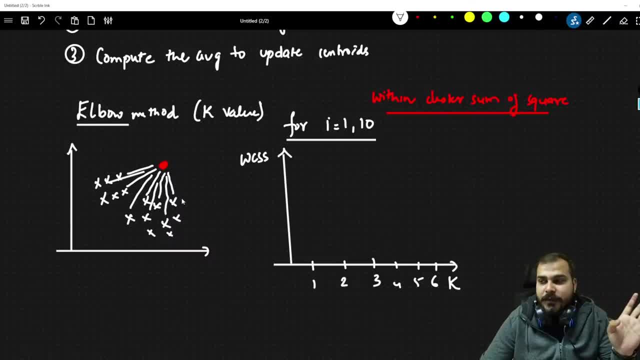 calculate this distance from this centroid to every point. this is what is within cluster sum of square right. tell me whether it will be greater or whether it will be smaller. whether it will be greater or whether it will be smaller, it will always be very, very much greater. 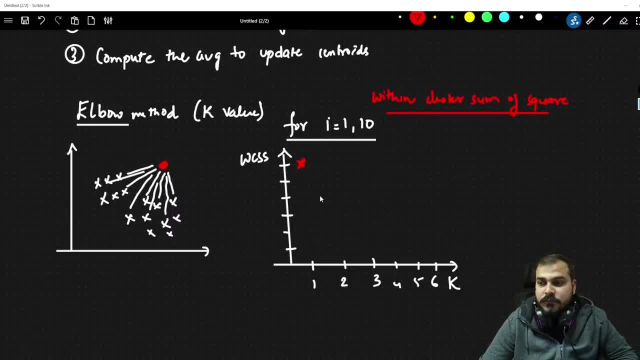 so let's say that my first point has to be greater, or whether it will be smaller. come somewhere here. okay, it is going to be obviously greater. okay, let's say that my first point is coming over here. fine, so within k is equal to one. initially, we took and we found out, 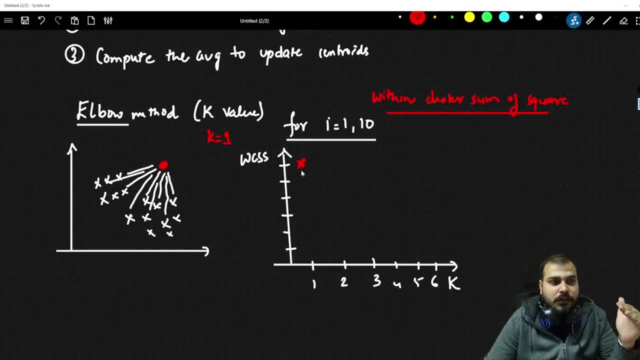 the distance of wcss, and it is a very huge value. okay, because we are going to compute the distance between each and every point to the centroid. now, the next thing that i'm actually going to do is that now we'll go with next value, that is, k is equal to two. now, in, k is equal to two, i will 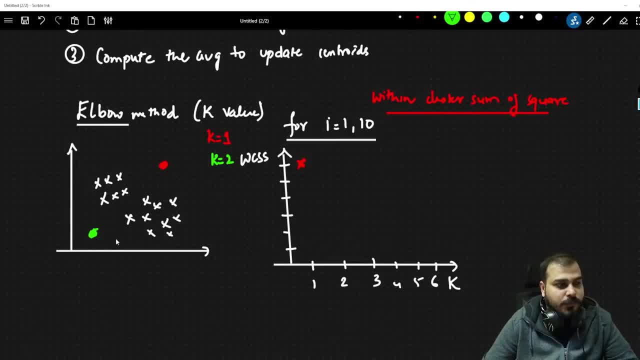 initialize the distance between each and every point to the centroid and i'm actually going to initialize two points. okay, i will initialize two points and then probably i will do the entire process which i have written on the top. now tell me whichever points is nearer to this green point. 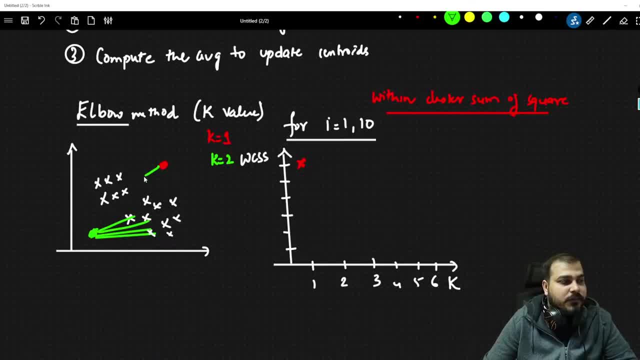 if we compute the distance and whichever points is nearer to the red point. if we compute the distance like this now, this summation of the distance will be lesser than the previous wcss, or not. obviously it is going to be lesser than the previous wcss. so what i'm actually going to do, probably with k, is equal to two. your value may come somewhere here. 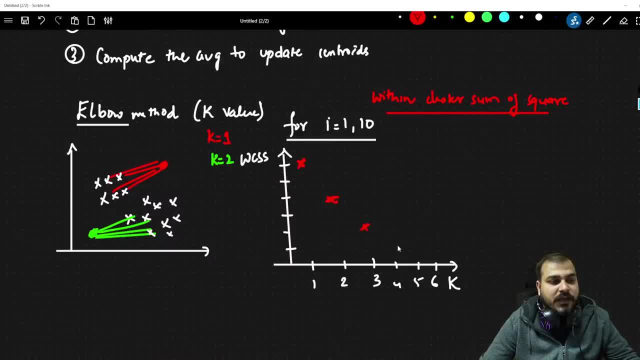 then with k is equal to three, your value may come somewhere here. then k is equal to four will come here to five, six, like this it will go okay. so here, if i probably join this line, you'll be able to see that there will be an abrupt changes in the wcss value. okay, in the wcss value there will. 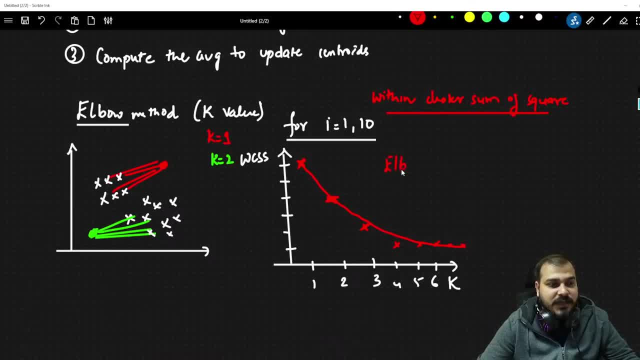 be an abrupt changes and this, this is basically called as the wcss value and this is called as elbow curve. now, why we say it as elbow curve? because it is in the shape of elbow. okay, and here, at one specific point, there will be an abrupt change and then it will be straight. 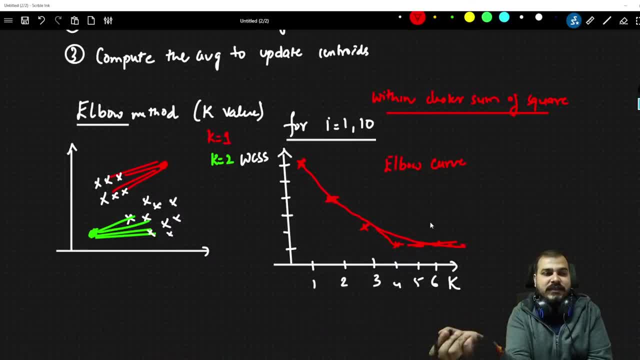 so that is the reason why we basically say this as elbow. okay. so this is a very important thing. see, in finding the k value, we use elbow method, but for validating purpose, how do we validate that this model is performing well? we use silhout score. that i'll show you just in some time. 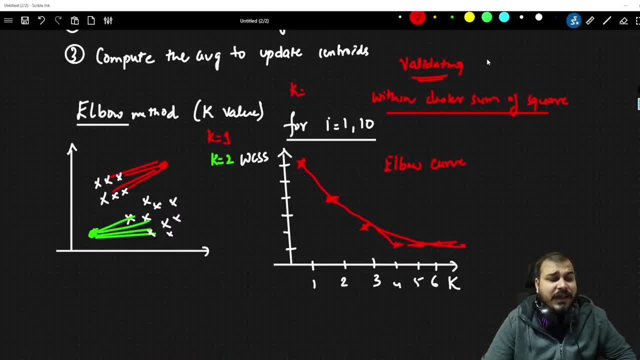 but understand that in k means clustering. we need to update the centroids and based on that we calculate the distance and as the k value keep on increasing, you will be able to see that the distance will become normal or the wcss value will become normal, and then we really need to find. 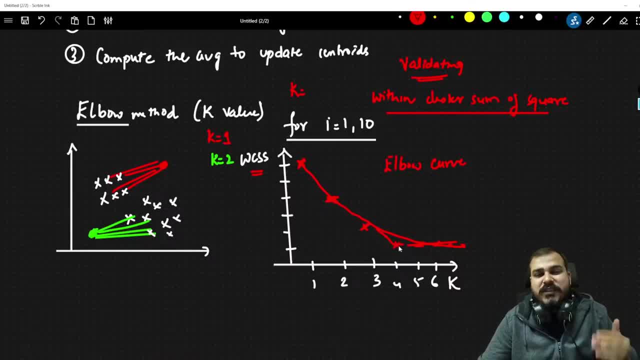 out which is the feasible k value where the abrupt change see over here. suppose abrupt change is there and then it is normal, then i will probably take this as my k value. i hope everybody is able to understand, okay. so obviously the model complexity will be high because we are going to check with respect to different, different k values and wcss values. 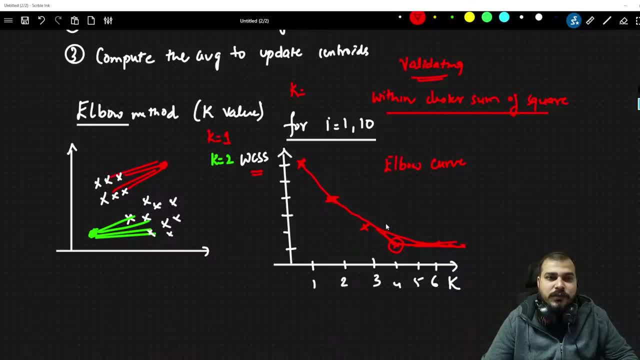 and this basically means that the value that we will probably get. first of all, we need to construct this elbow curve, then see the changes where it is basically happening. we'll need to find out the abrupt change and once we get the abrupt change, we basically say that this may be. 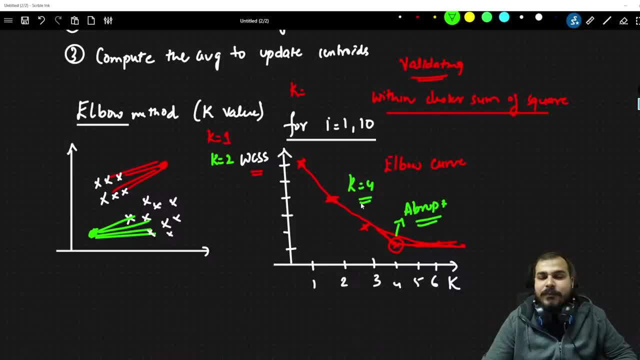 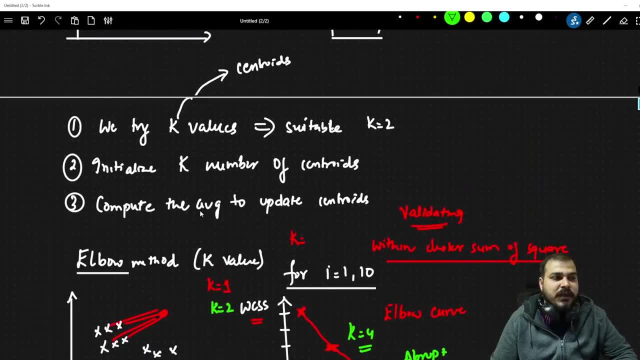 the k value and then we will be able to calculate the k value, and then we will be able to calculate the k value. so k is equal to four, as an example. i'm telling you. okay, so, unless and until, if you really want to find the cluster, it is very much simple. we take a k value, we initialize k number. 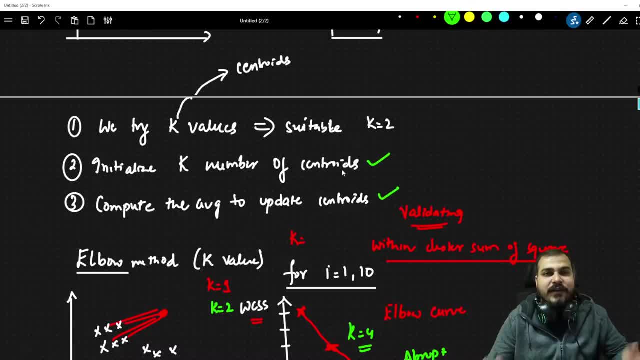 of centroids. we compute the average to update the centroids and again we try to find out the distance, try to see that, whether any points has changed, and continue that process unless and until we get separate groups. okay, so this is the entire funda of claimants clustering. okay, so finally you. 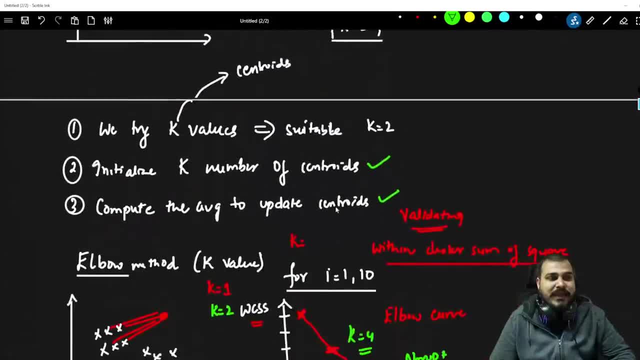 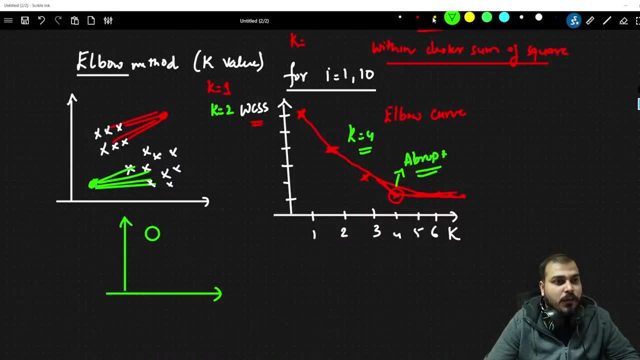 see that, with respect to the k value, will we be able to get that many number of groups? if my k value is four, that basically means i will be probably getting four different groups like this, one, two right, three like this and four. i will be getting four groups like this with k is equal to four. that 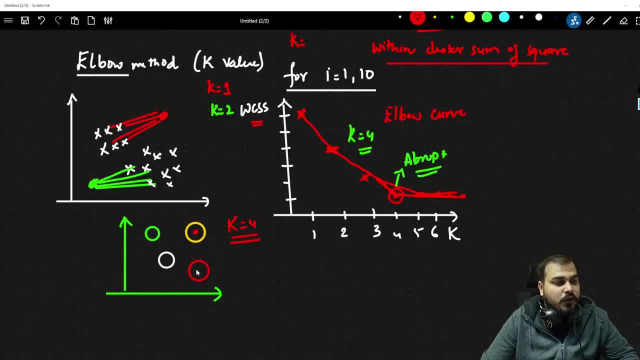 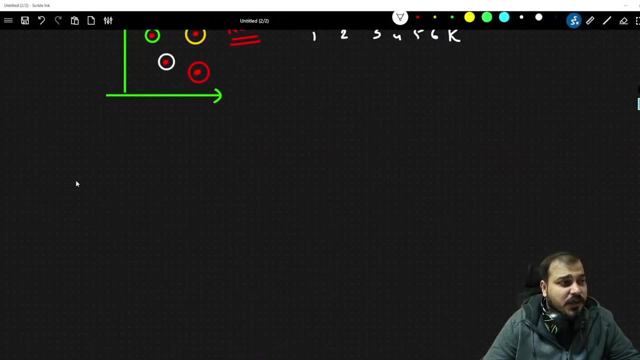 basically means k is equal to four clusters and every group will be having its own centroids. okay, every group will be having it with its own centroids. okay, centroids are very much important. okay, yes, i'll try to show you in the coding also, guys, don't worry. now let's go towards the second algorithm, the second algorithm that we will be. 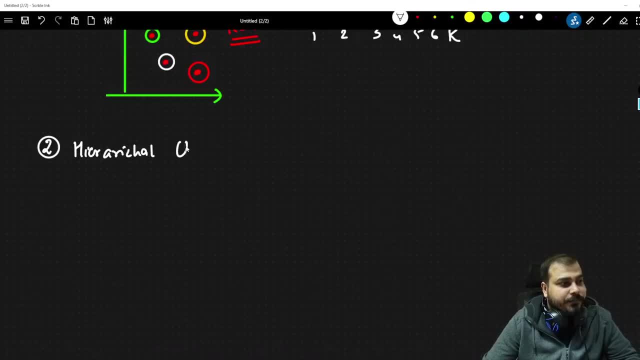 probably discussing is called as hierarchical clustering. now, hierarchical clustering is very much simple, guys. all you have to do is that let's say this is your data points, this is your data points. okay, let's say this is your data points. let's say this is your data points and this is my p one. let's say p two. okay, now hierarchical. 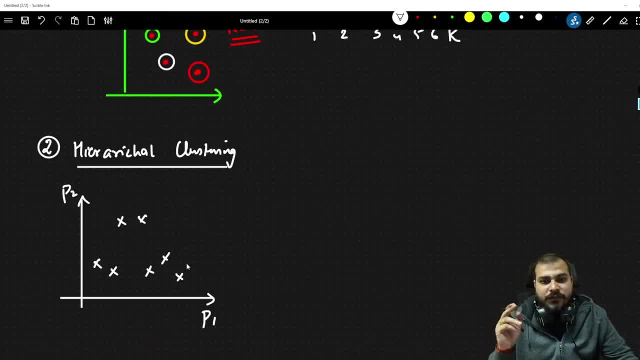 clustering says that we will go step by step. the first thing is that we will try to find out the most nearest value. let's say this is my x and y. let's say these are my points like, this is my r one point, this is my p, d, p. 2 point, this is my k right. see, sometimes we have to do some functions at least. 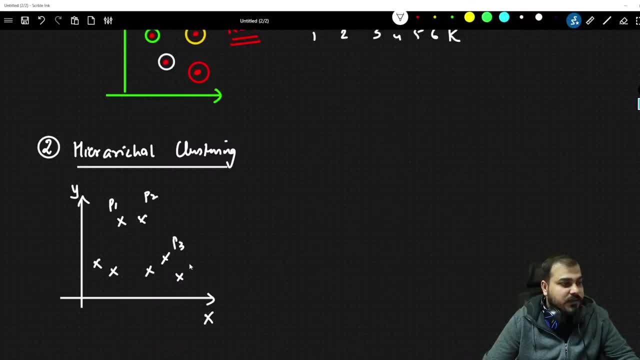 this is my p3 point, this is my p4 point, p5 point, p6 point, p7 point. okay, so these are my points that i have actually named over here. okay, now let's say that this is maybe the nearest point to each other. so what it will do? it will combine this together into one cluster. it will start. 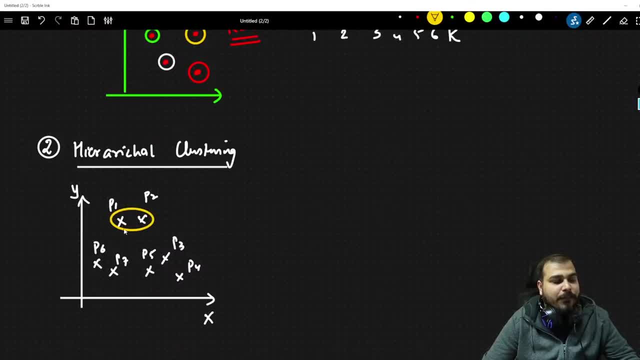 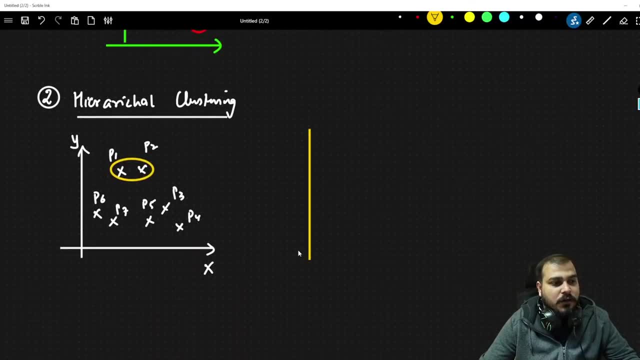 combining into one cluster. so let's say that this, we have computed the distance, so it will create one cluster. okay, now what will happen? on the right hand side, there will be another notation which may be using in connecting all the points one. so suppose this is my p1, this is my p2, this 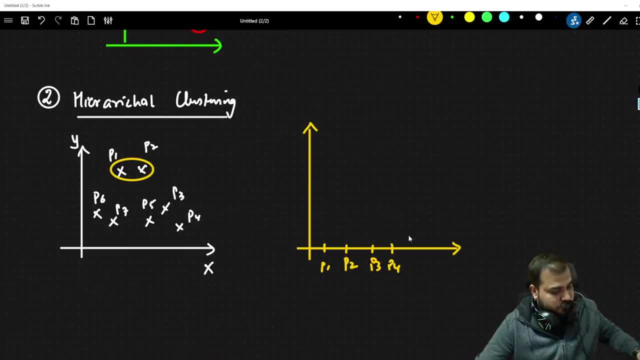 is my p3, p4, p5 and p6. okay, let's say that i have this many points and probably i will also try to make p7. so these are my points: p7. okay, now you know that the nearest point that we are having, okay, this will probably be distance one. 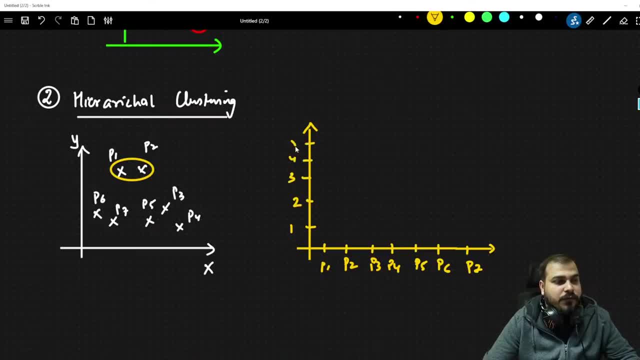 two, three- this is distance- okay- four, five, six, like this we have a lot of distance, okay, so hierarchical string will first of all find out the nearest point and try to compute the distance between them and just try to combine them together into one, into one. what do we do? we basically. 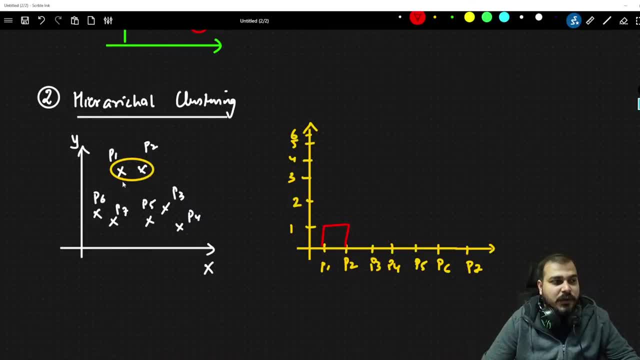 combine them into one group. okay, so p1 and p2 has been combined. let's say, then it will go and find out the other nearest point. so let's say p6 and p7 are near, so they are also going to combine into one group. okay, so once they combine into one group then we have 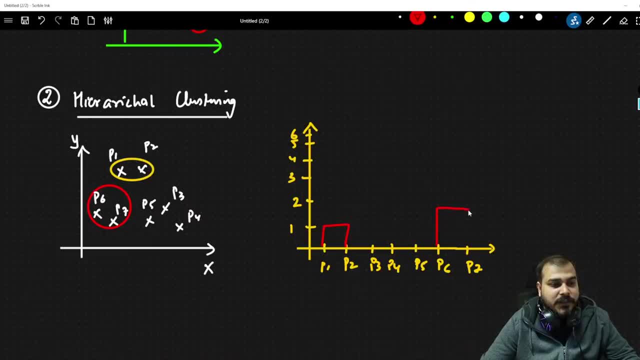 p6 and p7, which will be obviously greater than the previous distance, and we may get this kind of computation and another combination or cluster will form, get formed over here. then you have seen that, okay, p3 and p5 are nearer to each other, so we are going to combine this. so i am going to 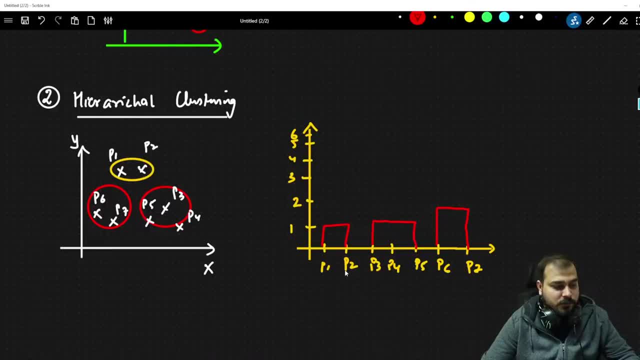 basically combine the distance between them and get the distance between them, and get the distance between p3 and p5. okay, and let's say that this distance is greater than the previous one, because we are basically going to start with the shortest distance and then we are going to capture the. 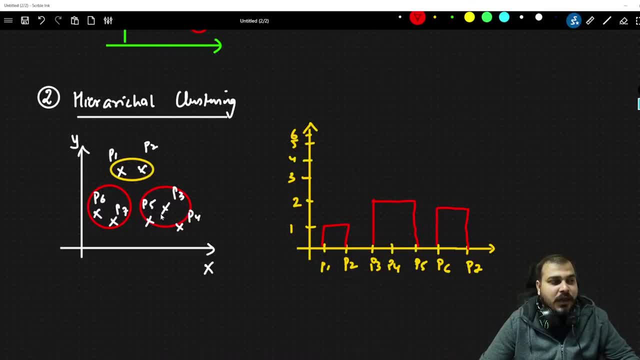 longest distance right now. this is done. now you can see that the next point that is near right to this particular group is p4, so we are going to combine this together into one group. okay, so once we combine this into one group, this p4 will get connected like this: 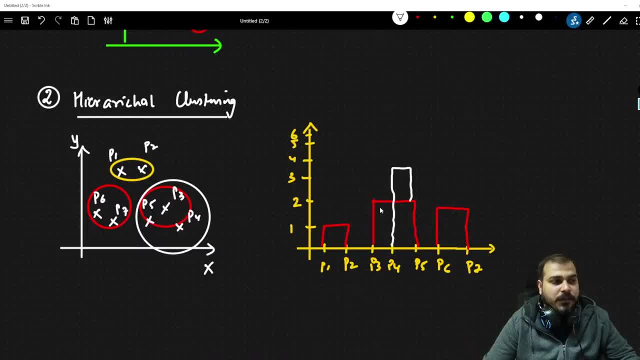 let's say it is getting connected like this: okay, p4 has got connected. then what is the nearest point? whether it is p6, p7, group of p1, p2, obviously here you can see that p1, p2 is there. so i am probably going to combine this group together. okay, that basically means p1- p2. let's say i am just going. 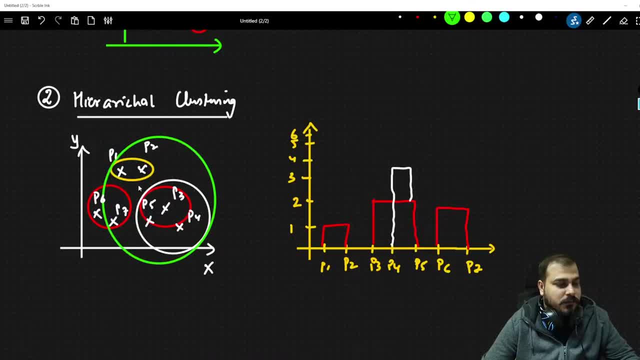 to combine this group together. again, circle is coming, so i will make a dot. let's say i am going to combine this group together because these are my nearest groups. so what will happen? p1 and p2 will get combined to p5. sorry, p4, p5 this one. so i will be getting 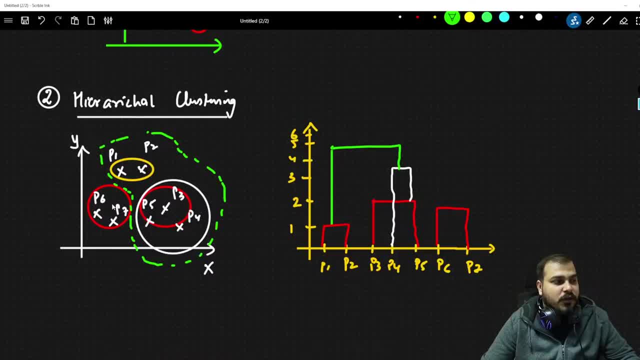 another line like this: okay, and then finally you will be seeing that p6, p7, is the nearest group to this, so this will totally get combined and it may look something like this: so this will become a total group like this, so all the groups are combined, so finally you will be able to see that. 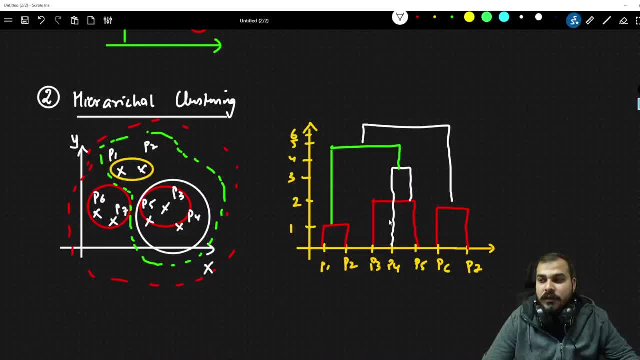 they will be one group and then you will be able to see that they will be one group and then you will be able to see one more line which will get combined like this: this is basically called as dendogram- dendogram okay, which is like bottom root to top okay. now the question arises is that: 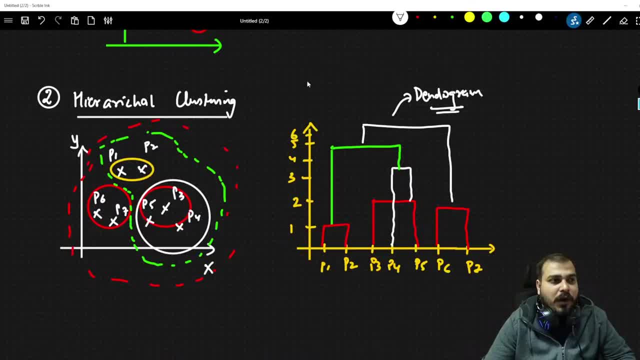 how do you find that how many groups should be here? okay, how do you find out that, how many groups should be here? the funda is very much clear, guys in this is that you need to find the longest vertical line. you need to find out the longest vertical line. 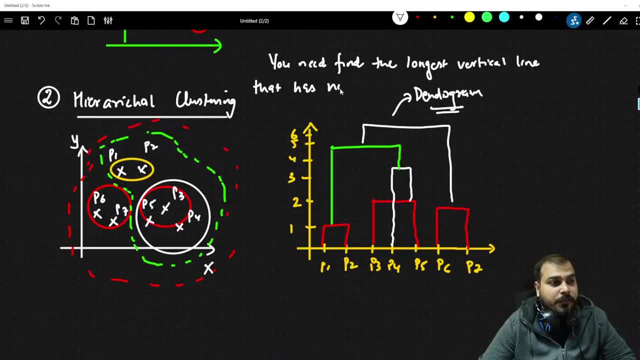 that has no horizontal line passed through it. no horizontal line passed through it. this is very much important. that has no horizontal line passed through it. now, what this is basically meaning is that i will try to find out the longest line, longest vertical line line, in such a way that none of the horizontal line passes through it. 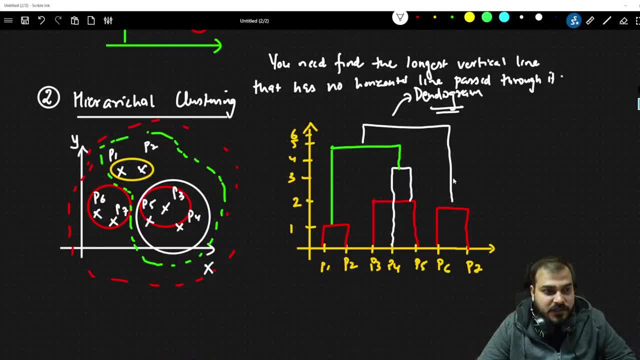 What is horizontal line? Suppose, if I consider this vertical line, this vertical line over here, if you see that if I extend this green line, it is passing through this. If I extend this line, it is passing through this right. If I'm extending this line, it is passing through this right. 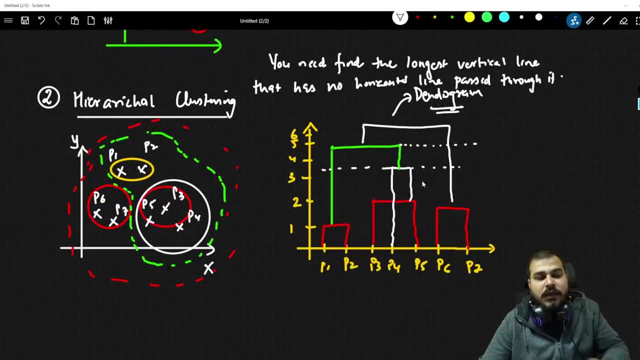 So, out of this, the longest line that may be passing in such a way that no horizontal line probably is this line that I can actually see. Okay, So what do you do over here is that you basically just create a straight line over this and 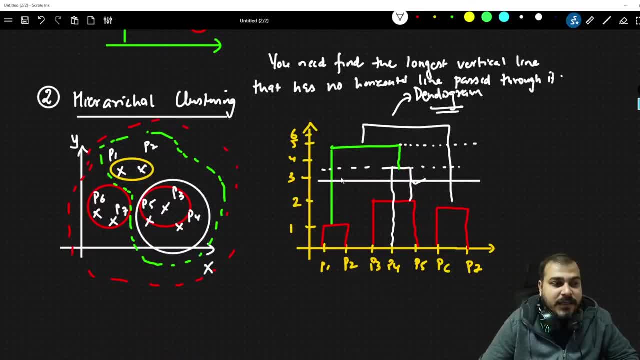 then you try to find out that how many clusters will be there by understanding that how many lines it is passing through. If it is passing through this one line, two line, three line, four line, that basically means your clusters will be four clusters. 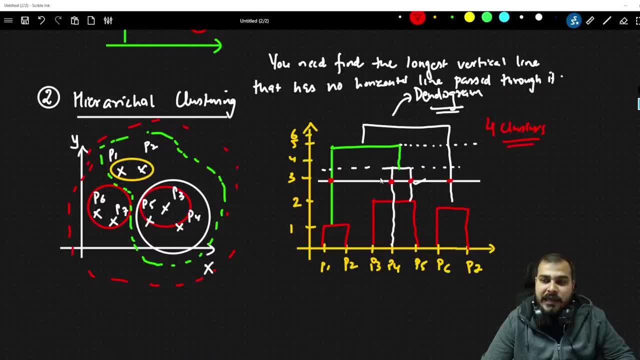 This is how we basically do the calculation in hierarchical clustering. Again here, it may not be the perfect line. I've just drawn with some assumptions, But if you are trying to do this, probably you have to do it in this specific way. 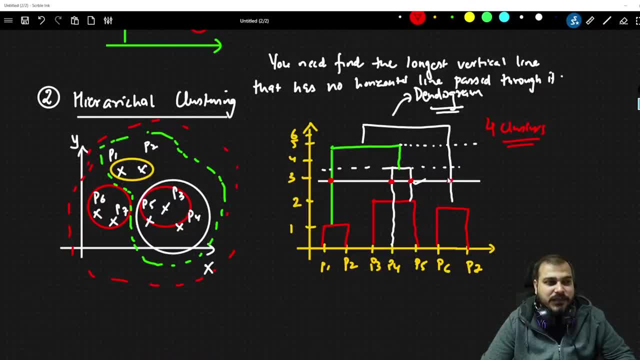 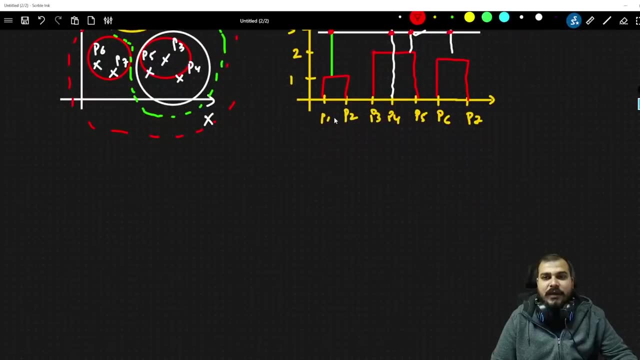 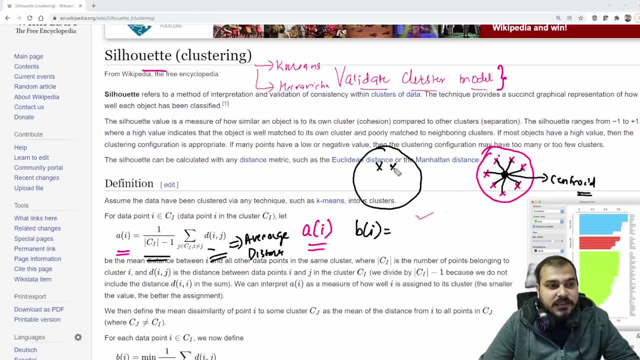 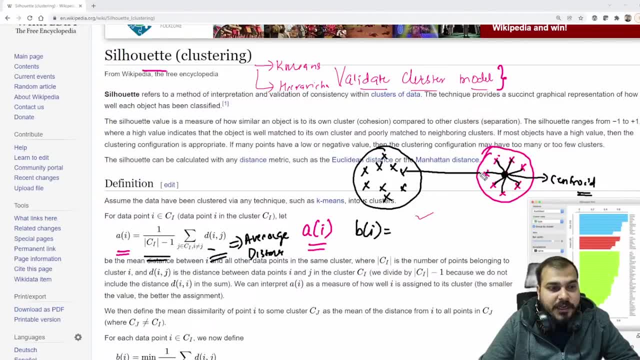 try to compute the distance between each point and the other point in this centroid- sorry, in this cluster. so this is my cluster 1, this is my cluster 2. so what i am actually going to do is that here i am going to compute the distance between this point to this point, then this point to this. 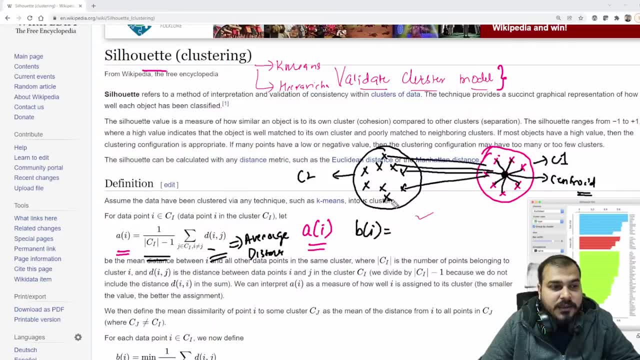 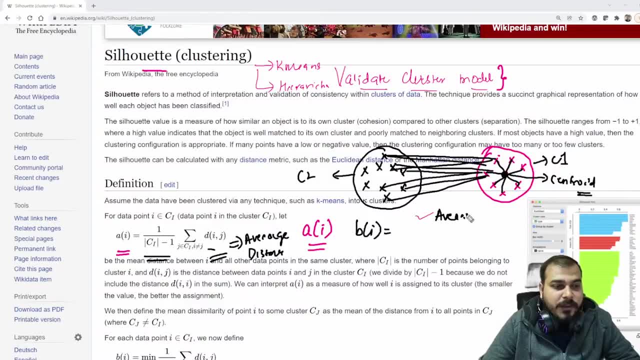 this particular distance. what we are going to do, we are going to do the average of them. average. okay, now tell me, if i try to find out the relationship between a of i and b of i, if my cluster model is good, will a of i will be greater than b of i, or will b of i will be greater than a of i if i have a good? 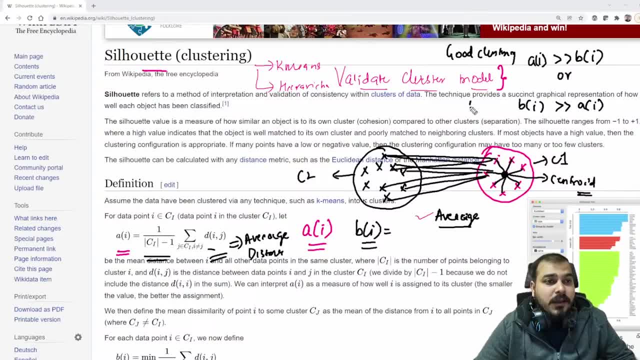 clustering model. tell me, if i have a good clustering model, will a of i is greater than b of i will be greater than b of i, or whether b of i will be greater than a of i. out of this, if we have a really good model, tell me guys. 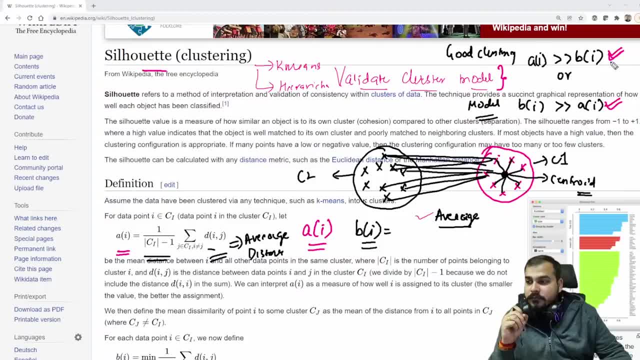 tell me, guys, whether a of i will be greater than b of i or whether b of i will be greater than a of i in a good model. obviously, the distance between b of i will be greater than a of i in a good model. okay, that basically means, if i talk about silhouette clustering, the values will be between minus one to. 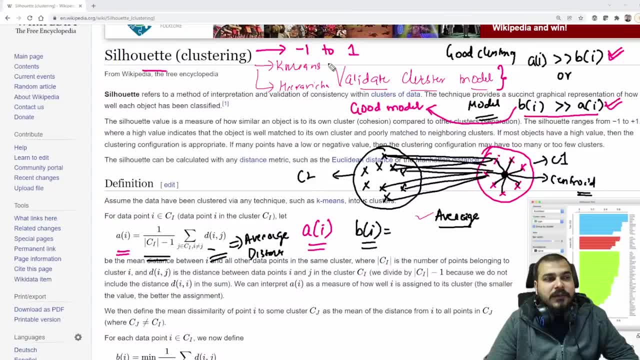 plus one, the more the value is towards plus one. that basically means: the good the model is, the good the clustering model is okay, the more the values towards negative one. that basically means this condition is getting applied. now what does this condition basically say? that basically means that this distance is far than the cluster distance. this is what this information is getting. 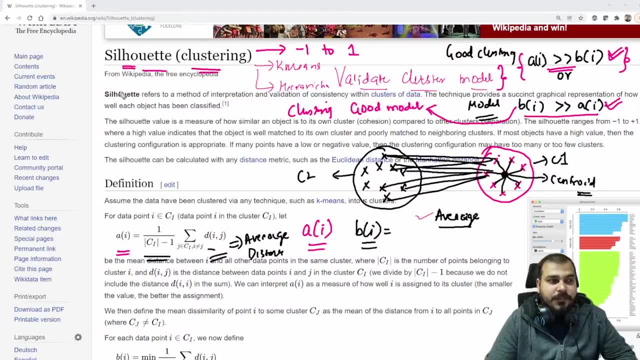 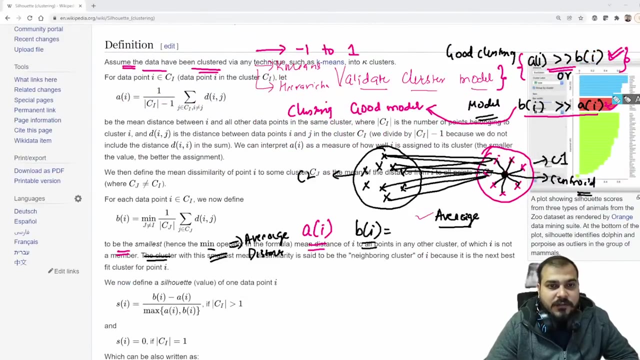 portrayed, and this is the importance of silhouette clustering. finally, when we apply the formula of silhouette clustering, you will be able to see that silhouette clustering is nothing. but let me rub this everything, guys, for you. okay, let me just show you what is silhouette clustering. silhouette clustering formula will be something like this: b of i. so here you have silhouette clustering. 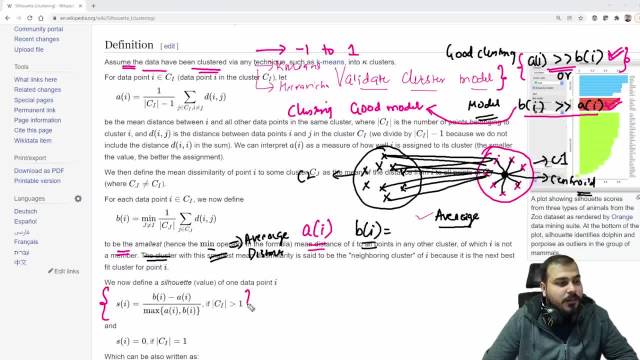 this is the formula b of i, minus a of i, max of a of i, comma b of i if c of i is greater than one right. so by this you will be getting the value between minus one to plus one, and more the value is towards plus one, the more. 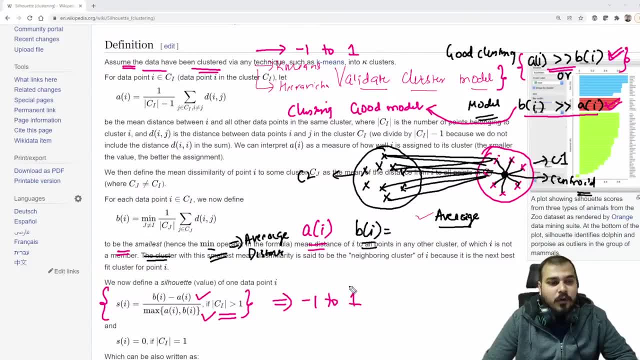 good your model is, more the value is towards minus one, more bad your model is because if it is towards minus one, that basically means your a of i is obviously greater than b of i. okay, so this is the outcome with respect to silhouette clustering. okay, so this is the outcome with respect to. 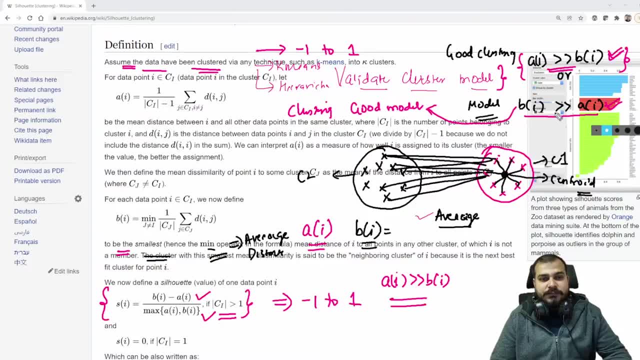 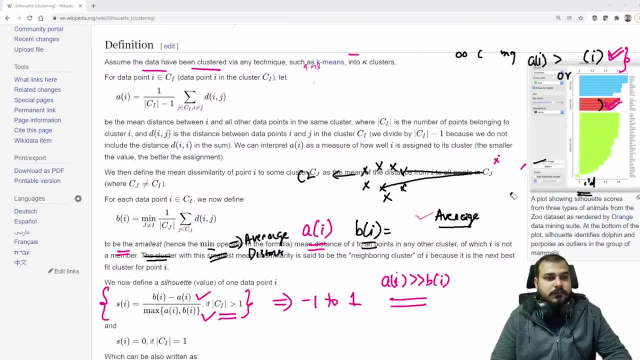 silhouette clustering. so everybody wants to do a practical session, just let me know. i hope everybody understood till here. we'll also discuss about db scan. don't worry, db scan is pretty much amazing than k means and hierarchical mean. i'll discuss about what is exactly db scan and then we'll discuss about the 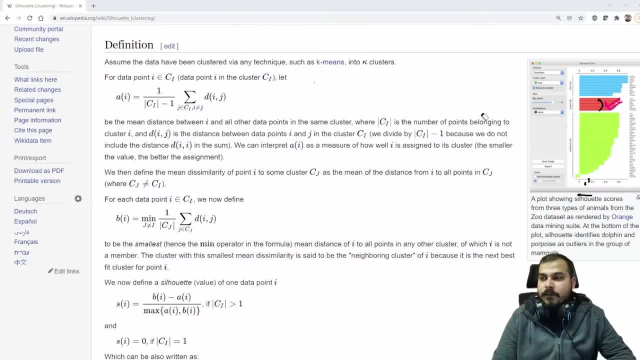 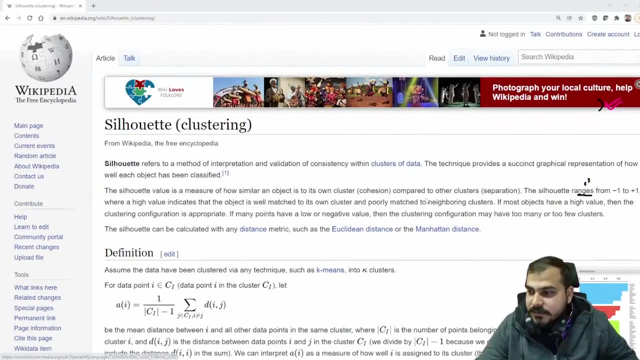 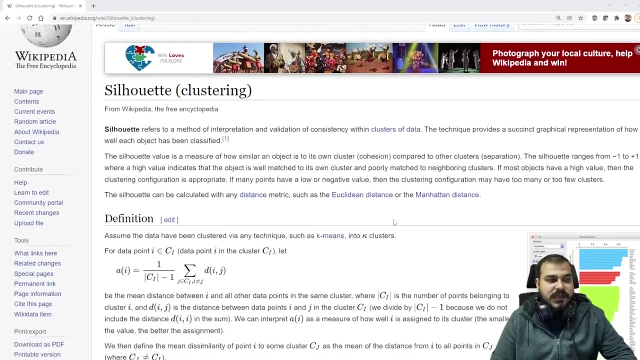 practical problem and then we'll finish it off. so i hope you had an amazing way of learning things. if s is equal to zero, that basically means still, your model needs to be basically, the clustering needs to be improved. okay, okay. what is i over here is nothing but one data point. you can just read this, guys. 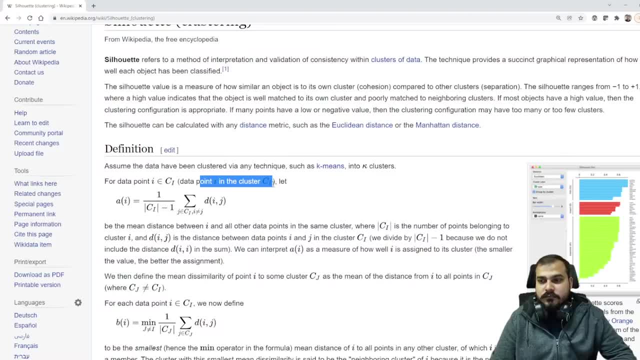 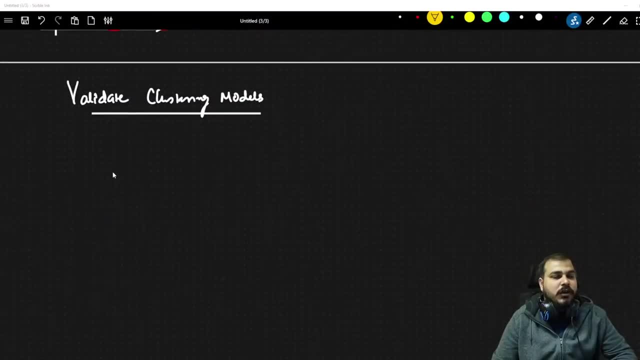 data point in i in the cluster c, so i hope everybody's understood this. now let's go ahead and let's discuss about the next topic. you can just read: we have obviously finished a silhouette clustering over here. let's discuss about something called as db scan pageации. 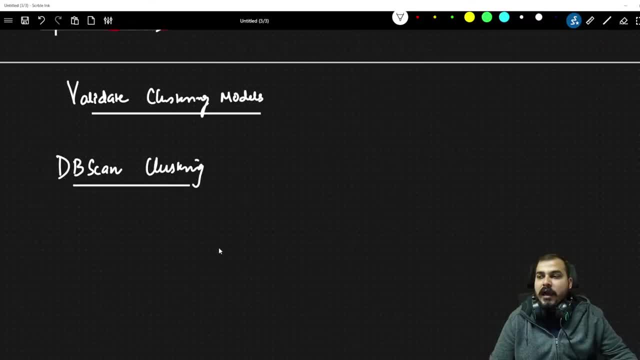 so for db scan clustering, this is an amazing clustering algorithm. we'll try to understand how to actually do do DB clustering and probably you'll be able to understand a lot of things from this. Let me show you one diagram. I'm going to take this diagram just a second. 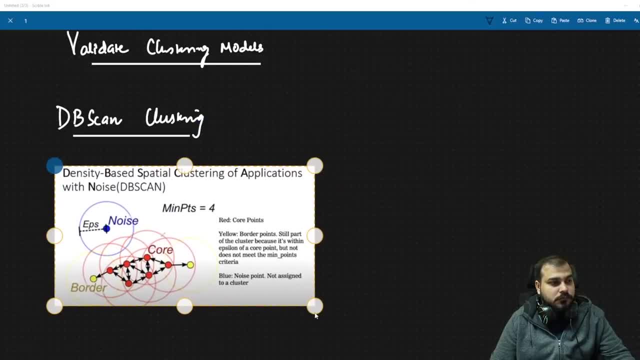 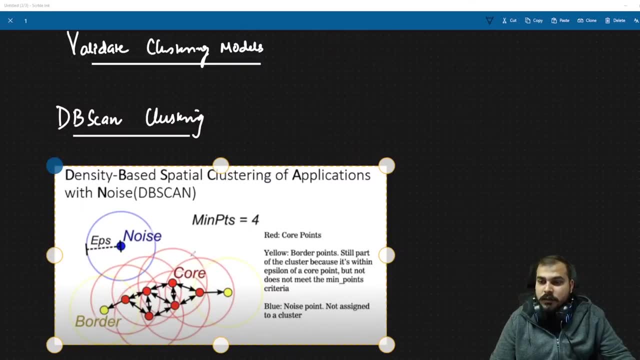 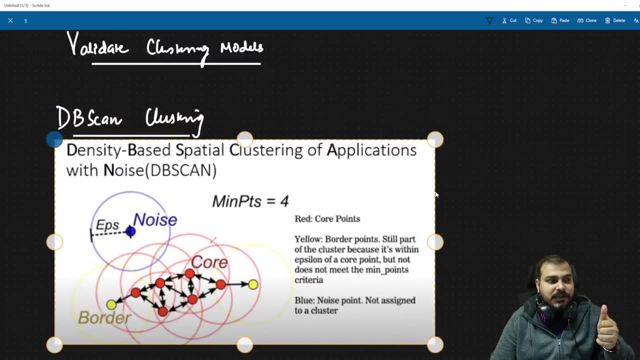 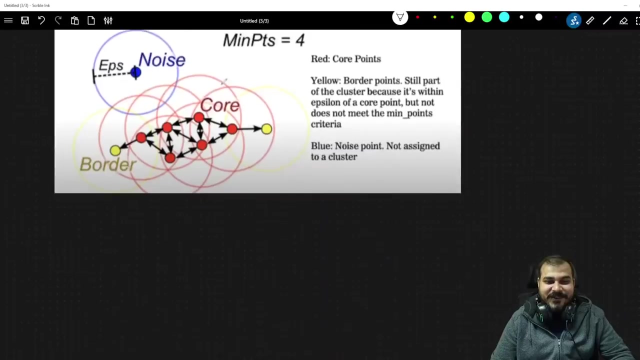 Yeah, practicals, I'll come ahead, Don't worry. Please hit like so that we'll be able to understand much, because I'll get the energy. When I get the energy, I'll be able to explain properly. I'm just kidding. anyhow, If you don't like also, it's okay. 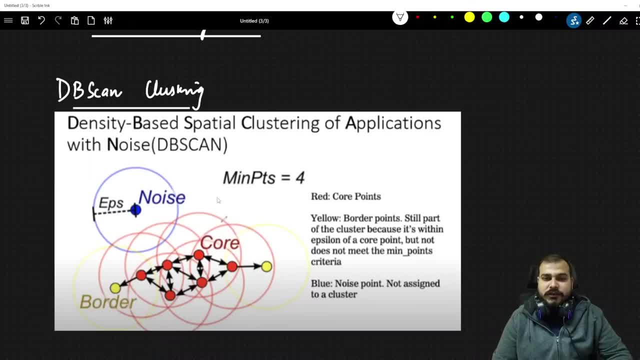 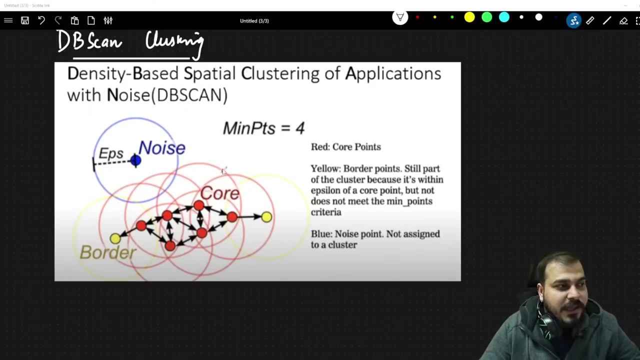 Okay, Now in DB scan, clustering, what are the important things? Okay, Shall I start everyone. Okay, Shall I start everybody. Okay, So let's start with respect to DB and clustering And let's understand some of the important things. So let's start with respect to DB and clustering. 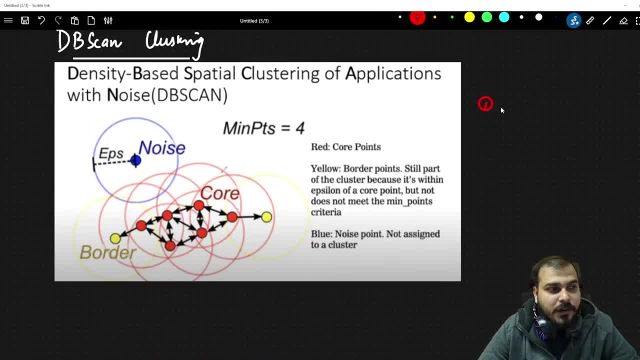 important points over here. the first point that you really need to remember is something called as score points. i'll also talk about when do you say core points or when do you say other points as such. so the first point that i will probably discuss about is something called as min points. 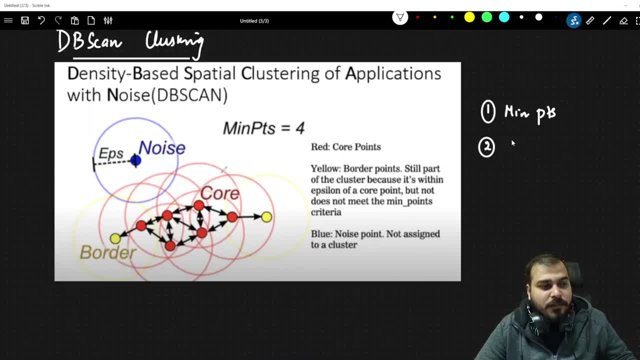 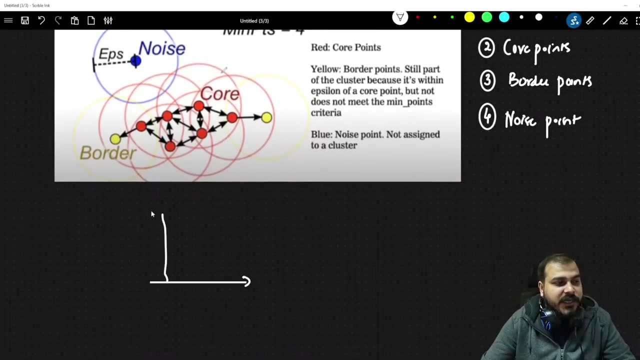 the second point that i will probably discuss about is something called as score points. okay, the third thing that i will probably discuss about is something called as border points, and the fourth point that i will definitely talk about is something called as noise point. okay, guys, now tell me in in, in k-means clustering if i have this kind of groups. 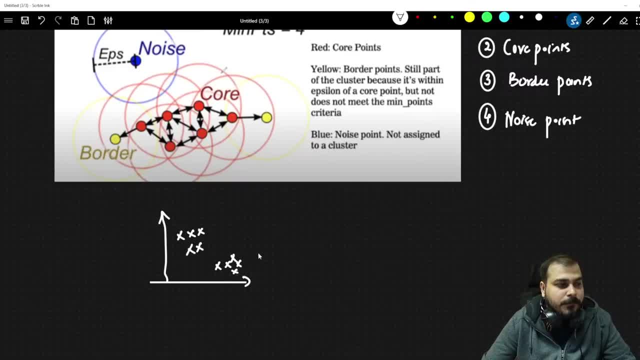 okay, don't you think? with the help of two different clusters, i may combine this two like this? yes, with the help of two different clusters, i may combine something like this. right, but understand over here what? what problem is basically happening with the second clustering? this is actually an outliers. let's say, for example, if you have a group like this: 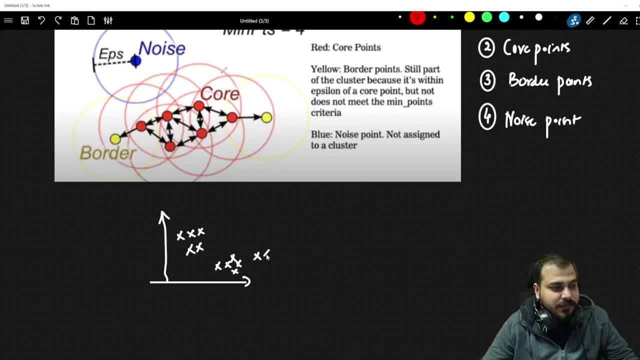 that let's, let's. let's say one thing very nicely. i will put: okay, let's say, i have one point over here, i have one point over here, so if i do clustering, probably i will get one cluster here and i may get another cluster which is somewhere here. 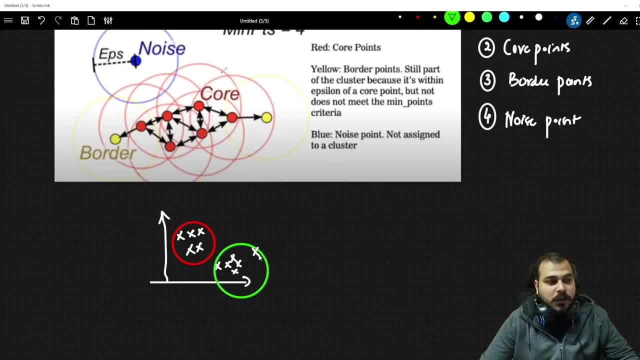 okay, now understand one thing: this point is definitely an outlier. even though this is an outlier with the help of k means what i am actually doing, i am actually grouping this into another group. so can we have a scenario wherein a kind of clustering algorithm is there, where we can leave the outlier separately and this outlier in this particular algorithm, and 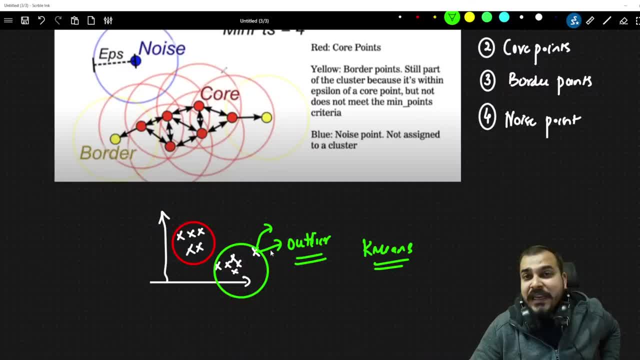 this is basically: we will be using db scan to relieve the outlier and this point will be called as a noisy point- noisy point or i can also say it as an outlier, so this will be a noise point, okay. so for this kind of algorithm where you want to skip the outliers, we can definitely use db scan. 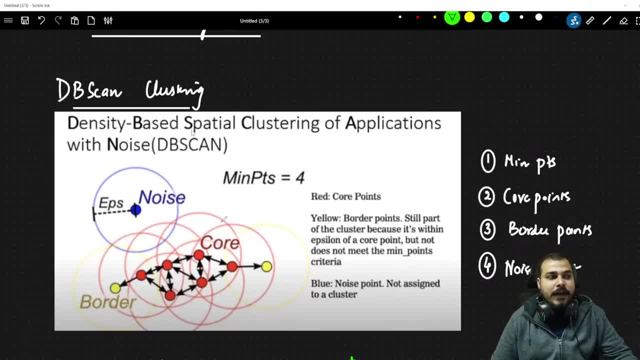 that is, density based spatial clustering of application with noise. a very amazing algorithm and definitely i have tried using this a lot. nowadays, i don't use k means or hierarchical means. instead, i use this kind of algorithm. okay, now see this. what are the important things over here? first of all, you need to know that, you need to know that. you need to know that you need to. 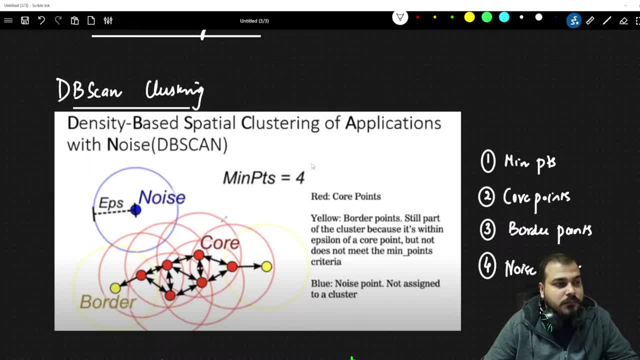 go ahead with min points, min points. so first thing is that you need to have min points. this min points is a kind of hyper parameter. this basically says what does? hyper parameter says: and there is also a value which is called as epsilon, which i forgot. i will write it down over here. this is called as epsilon. now what does? 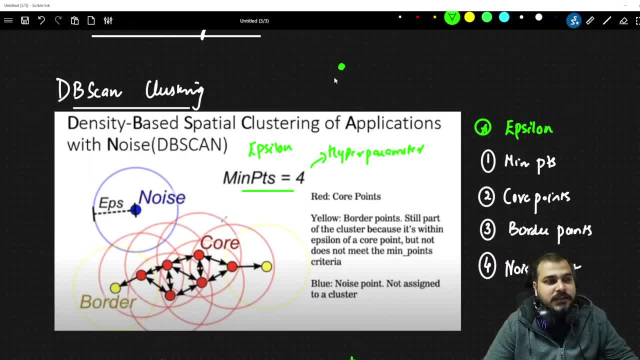 epsilon mean. epsilon basically means: if i have a value which is called as epsilon, i have a point like this: and if i take epsilon, this is nothing but the radius of that specific circle. okay, radius of that specific circle, okay. so epsilon is nothing but radius, okay, over here. 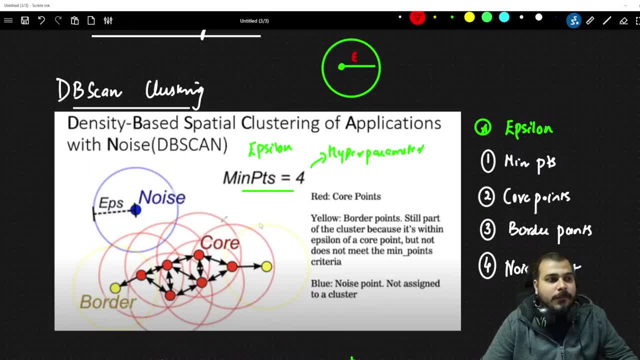 in this specific thing. now, what does minimum points is equal to four mean? let's say that i have, i have taken a point over here. let's say that this is my point and i have drawn a circle which is like this: okay, and let's say that this is my epsilon value. okay, this is my epsilon value. if i say: 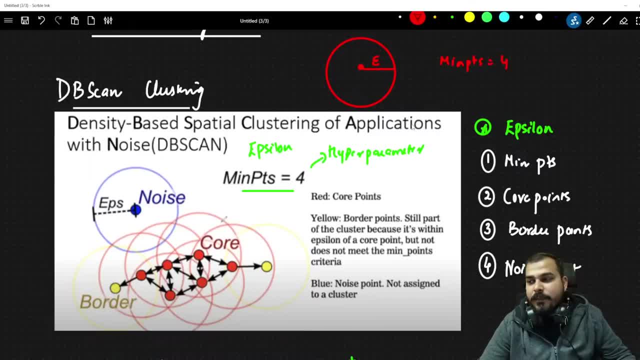 my min point is equal to four, which is again a hyper parameter. that basically means i can, if i have four, at least four points over here. at least four points over here, okay, at least four points near to me, near to this particular circle based on this epsilon value. then what will happen is that 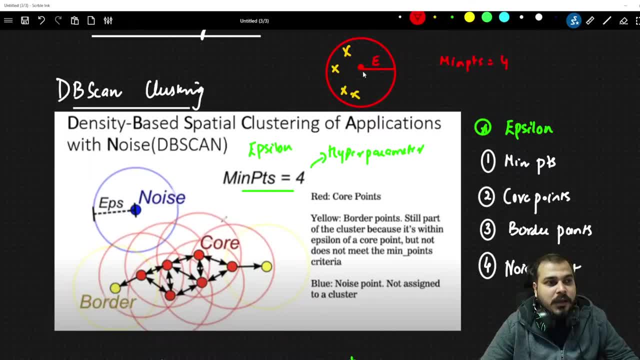 this point, this red point, will actually become a core point, a core point which is basically given over here. okay, if it has at least that many number of min points inside or near to this particular, within this epsilon. okay, within this particular cluster- suppose this is my cluster- with the help of 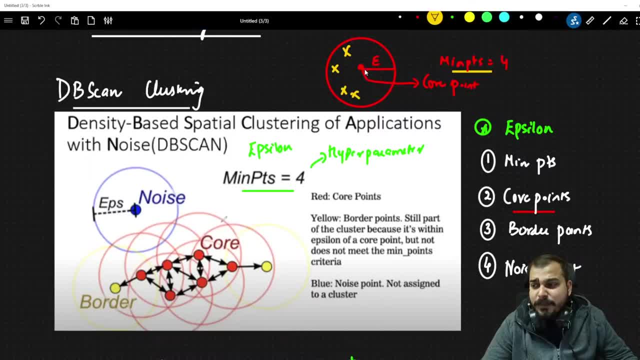 epsilon. i have actually created it. okay, is there a particular unit of epsilon or we simply take the unit of distance? no, epsilon value will also get selected through some way. okay, i'll show you. i'll show you in the practical application, don't worry. okay, now the next thing is that let's say, let's say i have another, another point over here. let's: 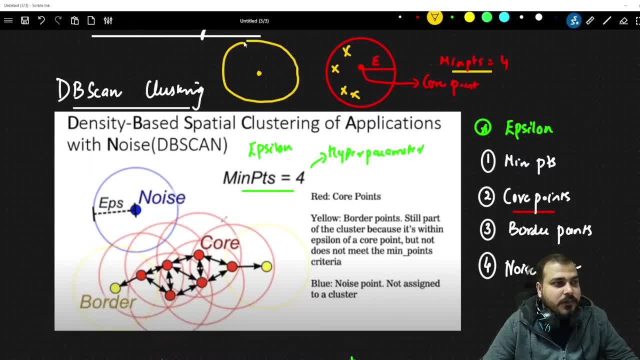 say that i have another point over here, and this is my circle with respect to epsilon. i have created it. let's say that here i have only one point. i have only one point inside this particular cluster. at that point, this point is going to be the point where i am going to be able to create a circle. 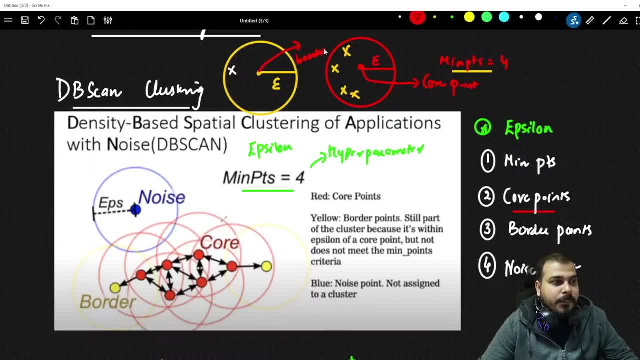 and that point becomes something called as border point, border point, border point also. we have discussed over here, right? so border point is also there, okay. so here i'm saying that at least one, at least one, if it is only one, it is present, okay, then it will become a border point if it has force, definitely. 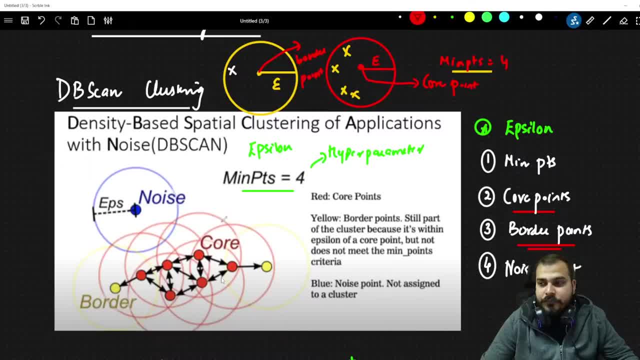 this will become a core point. core point, like how we have this red color. okay. so, and there will be one more slide here- and this is the point where i am going to be able to create a circle. okay, and this is the point where i am going to be able to create a circle. 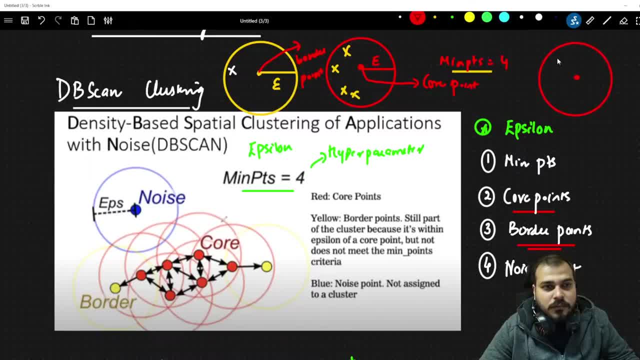 scenario: suppose I have this one cluster- let's say this is my epsilon- and suppose if I don't have any points near this, then this will definitely become my noise point and this noise point will nothing be, but this will be a cluster. okay, so here I have actually discussed about the noise point. 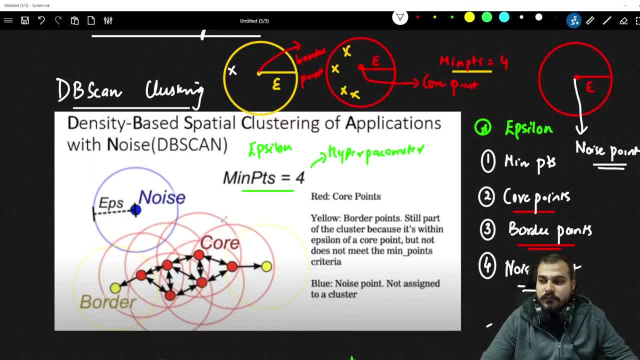 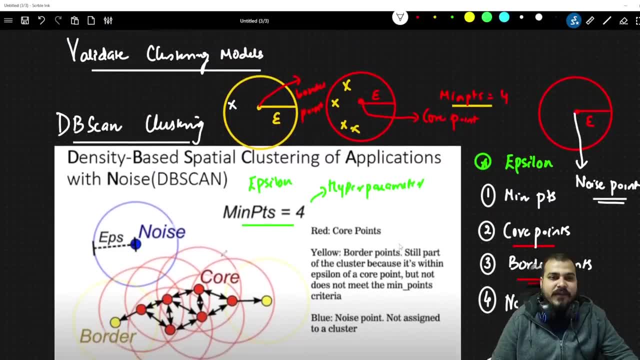 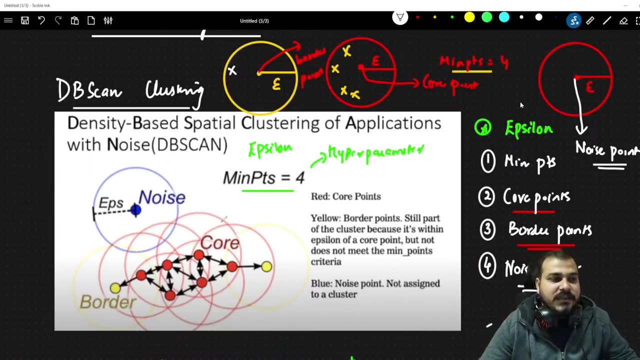 also right. so I hope everybody is able to understand the key terms now. what is basically happening is that whenever we have a noise point, like in this particular scenario, we have a noise point and we don't find any points inside this, any core point or border point. if we don't find 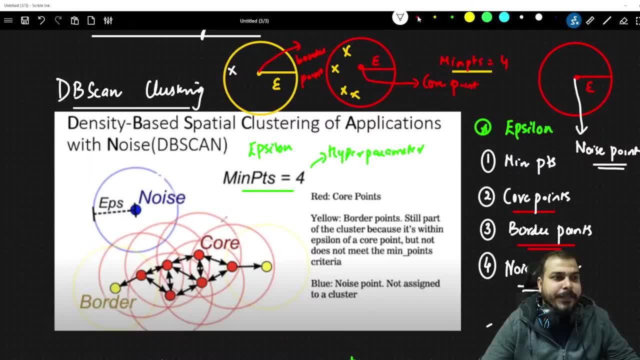 inside this, then it is going to just get neglected. it is just going to get neglected. that basically means this is basically treated as an outlier. okay, I hope everybody is able to understand here. okay, so I hope everybody is able to understand here. so I hope everybody is able to understand here. 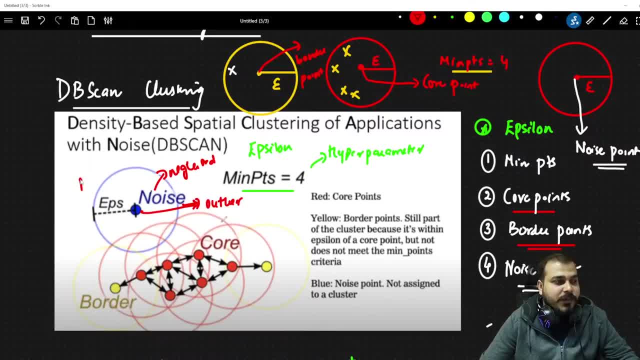 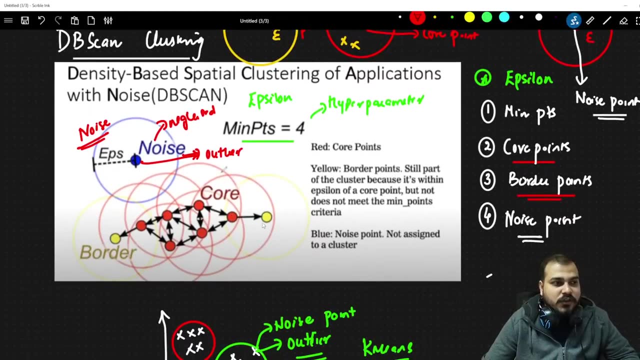 this point will be treated as an outlier or it can also be treated as a noise point and this will never be taken inside a group. okay, it will never, never be taken inside a group. suppose i have this set of points which you see basically over here, red core and all, and there is also a 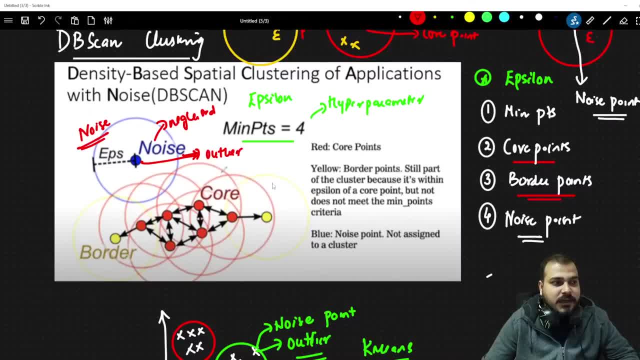 border point by making multiple circles over here. you can definitely say that how we are defining core points and the border points and this can be combined into a single group. okay, this can be combined into a single group because how the connection is now see this: this yellow line is: 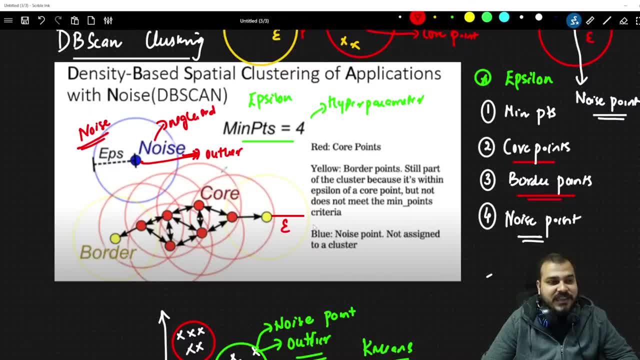 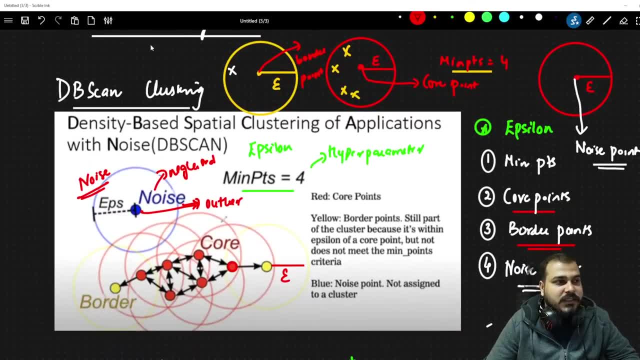 basically created by one. sorry, this yellow point is basically created by one- epsilon, and we have one core point over here. remember, over here it should be at least one core point. okay, not one point, but one core point at least. if it is having one core point, then it will. 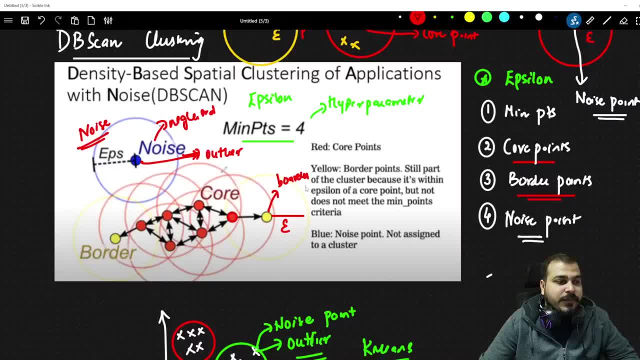 be a single group and if it is having one core point, then it will be a single group, become a border point. this will become a border point. that basically means, yes, this can be the part of this specific group. okay, so understand one this. these things, don't worry guys. tomorrow, 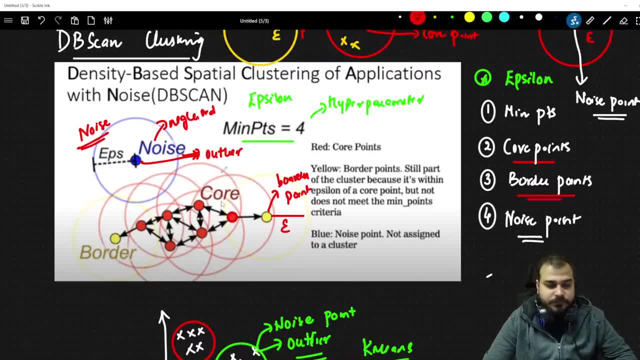 xg boost will get covered. we'll also cover svm and sdr, don't worry. okay, focus on the session right now. so what we are doing: whenever there is a noise, we are going to neglect it. wherever there is a broader and core points, we are going to combine it. so i will show you one more diagram, which is: 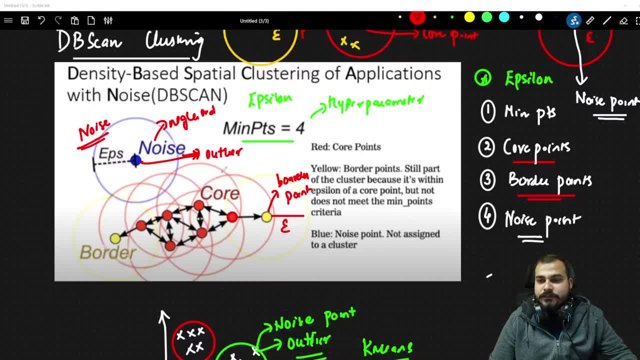 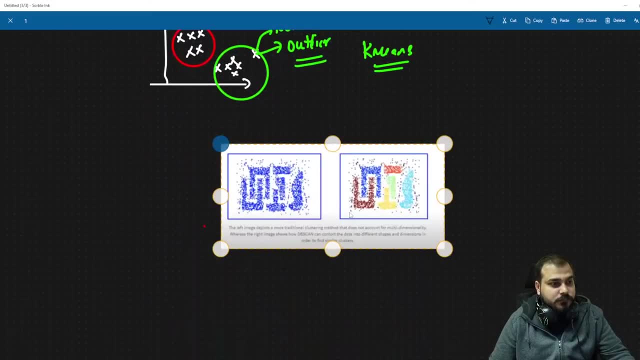 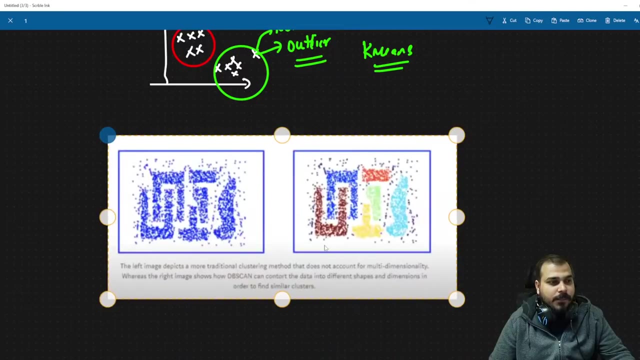 an amazing diagram which will help you understand the core points and the core points and the core points and more in this. just give me a second. i'm just going to keep that screenshot. now i'm going to show you the difference between, difference between a k-means clustering and hierarchical mean clustering. now see this everybody. 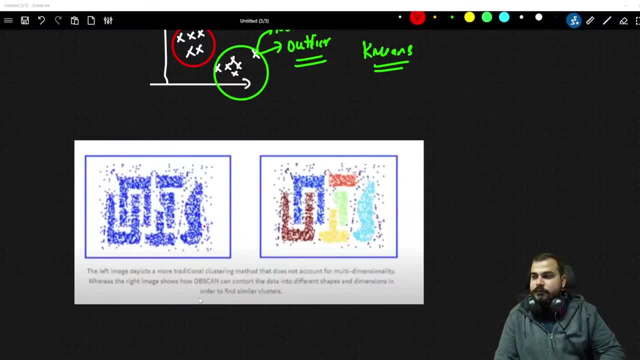 i hope everybody is able to see this group. see this. don't worry guys. svm xg boost tomorrow. i'll complete it now. the right hand side of diagram that you see is based on dv scan clustering and the left hand side is basically your traditional clustering method. let's say that. 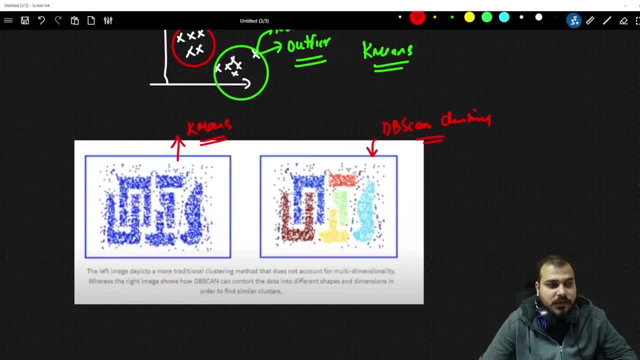 this is k-means. which one do you think is better over here? you see this. these all outliers are not combined inside a group, but whichever are nearer to the outliers are not combined inside a group. as a core point and the broader point, separate separate groups are actually created. 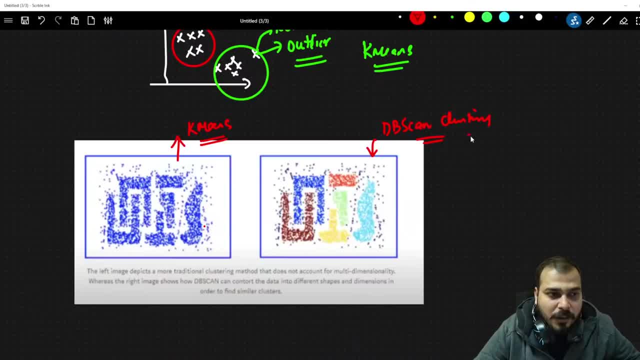 right. so this is how amazing a db scan clustering is right. a db scan clustering is pretty much amazing. that is basically the outcome of this here in k-means clustering. you can see this. all these points has also been taken as blue color as one group, because i'll be considering this as one. 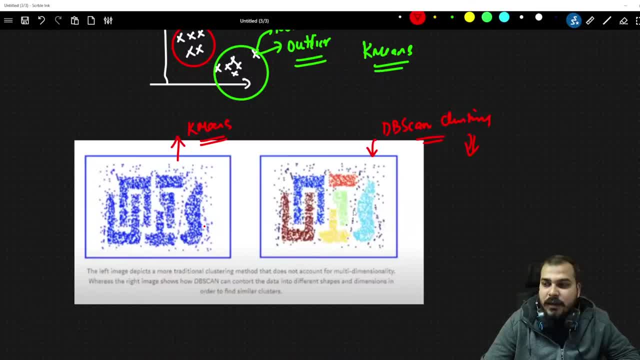 group, but here we are able to determine this in our amazing groups. so any, i'm saying you guys directly use db scan without worrying about anything. okay, so now let's focus on the practical part. uh, i'm just going to give you a github link. everybody, please download. 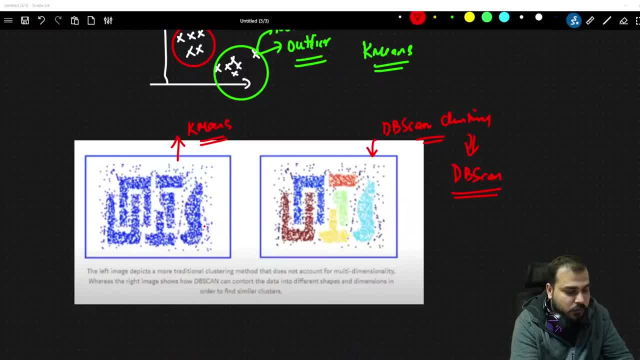 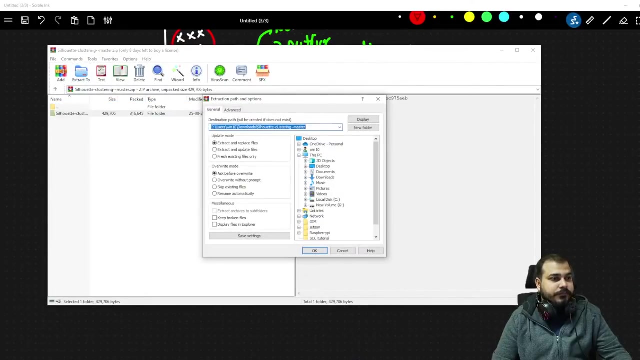 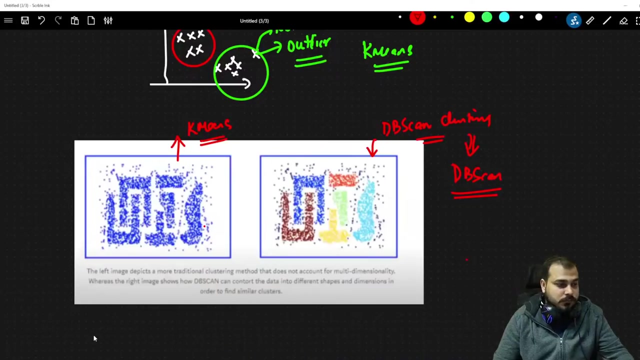 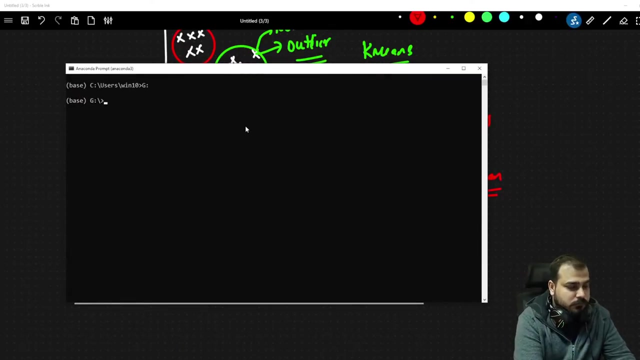 the github link. download the code. so download the code, guys. i've given you the github link. quickly download and keep your file ready. i'm also going to download. i'm going to open my anaconda prompt, probably open my jupyter notebook. we'll do one practical problem. 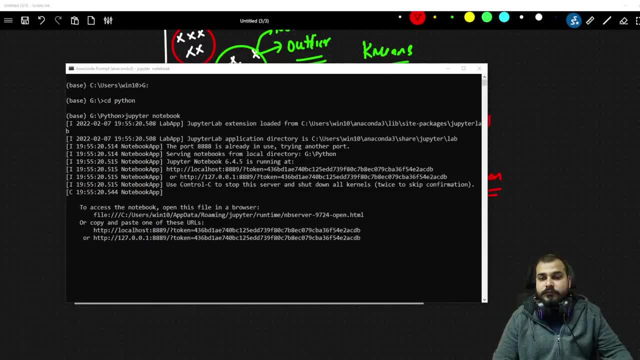 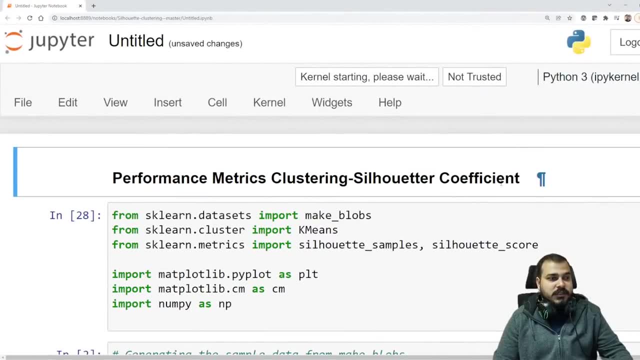 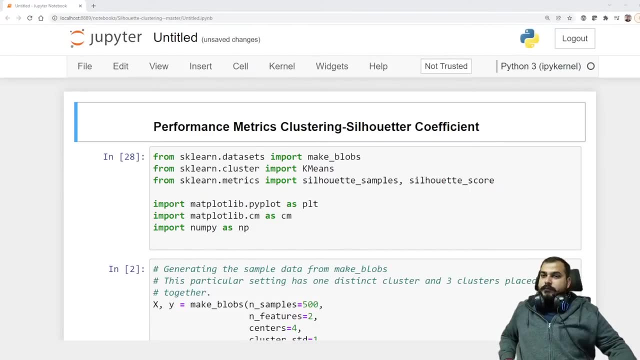 we'll do one practical problem. so i've given you the link, guys, please open it. so this is what we are going to do today. just let me know once you have downloaded it or not, and hit like let's make it at least 300. and hit like let's make it at least 300. 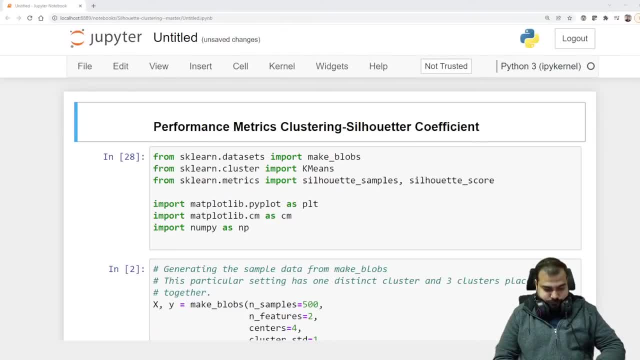 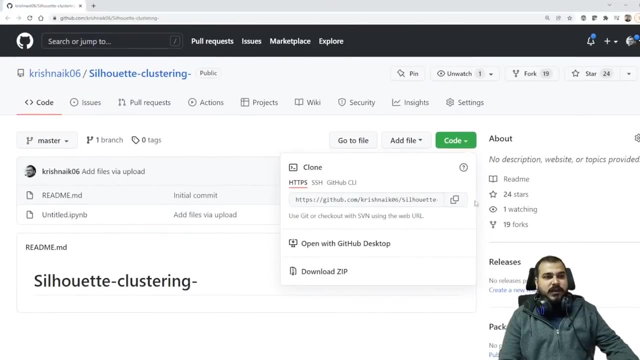 300. how to download? you don't know how to download. i've given you the github link. no, seriously, you don't know how to download. so this is the github link. go to the code, download the zip file or fork the this entire repository. just download the zip file. 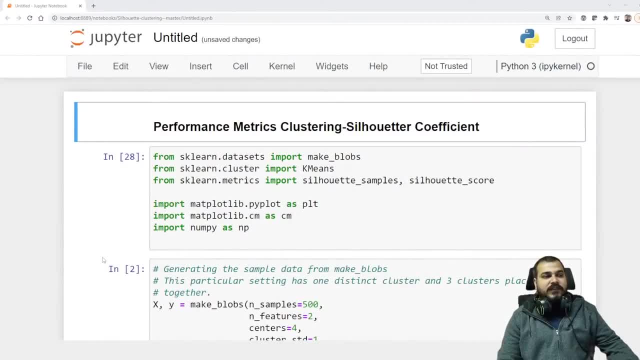 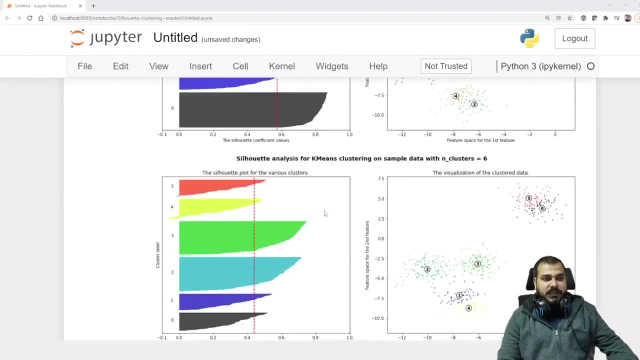 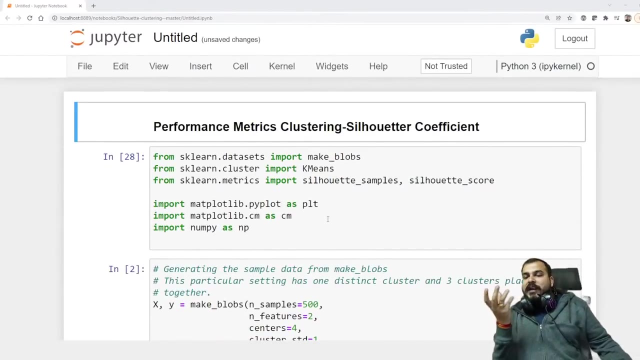 and please open the file and keep it ready, and then we will try to explain. see this, this will be amazing. here you will be able to see amazing things. how do you come to know that overfitting or underfitting is happening? you don't know the. 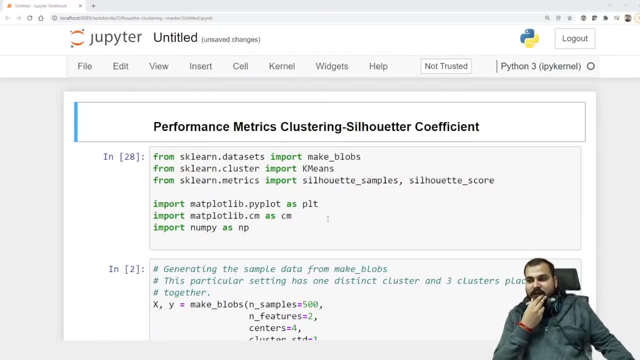 real value right. so in in clustering, there will not be any underfitting or overfitting. everybody ready, you, everybody ready. just give me a confirmation. it's so amazing. daily five to six messages. i get one one. the last one is where people are making successful career transition. 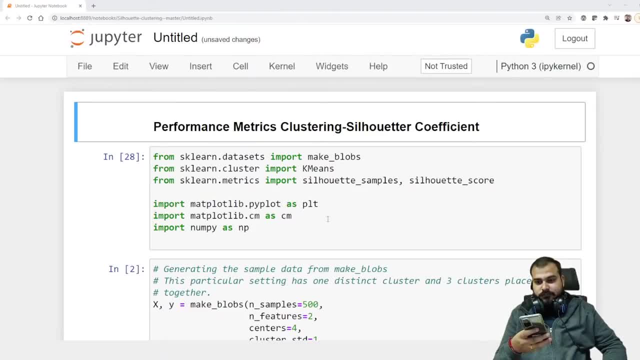 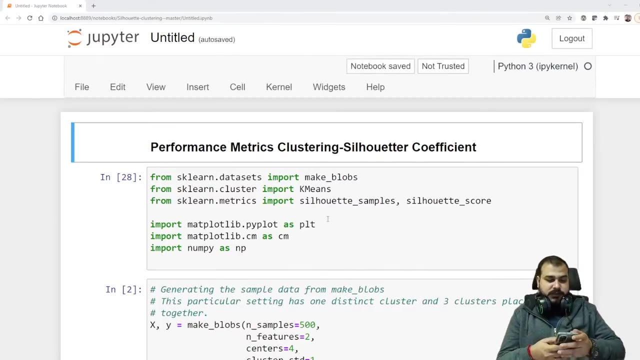 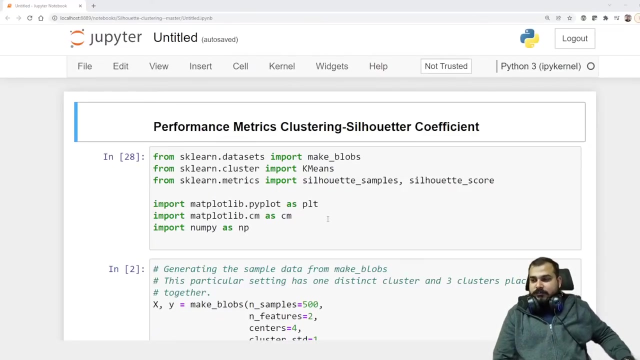 amazing five to six. today i got around 10 messages both in linkedin and- uh, you know the other platforms- whatsapp, many, many people, many people are getting jobs in data science. they are part of amazing right. so this, this is give basically the motivation to be able to do the work that you are doing and to be able to do the work that you are doing, and to be able to do the work that you are doing and to be able to do the work that you are doing. 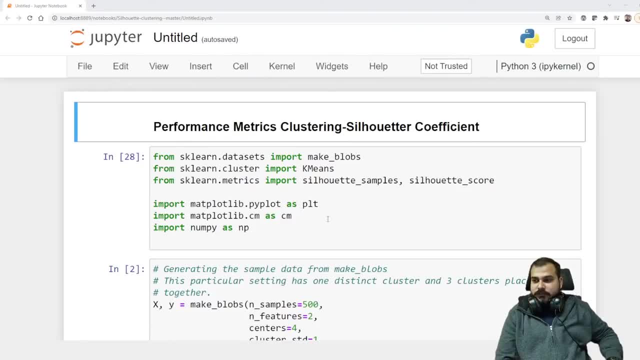 okay, now let's start. everybody focus on the code over here now. so, uh, what all things we will be importing first is that we'll try k-means clustering, we'll do silhouettes scoring and then probably we'll see the output okay and um, and we'll do db scan also. let's say, db scan is also. 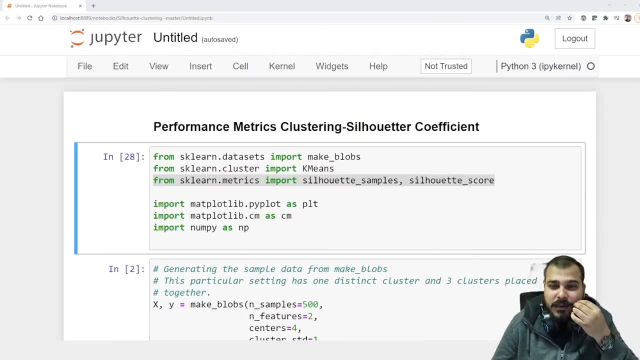 there, uh, db scan. i'll refer it to one video so that you can check it from there. not a problem, okay, so, uh, what are the things we have basically done? so we have done the basically imported one is the k-means clustering. one is the silhouettes, samples and silhouettes. 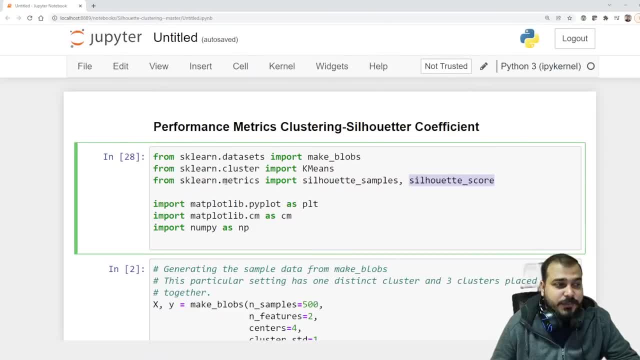 scores. these all are present in the sklearn and it is present in the matrix. that basically means we use this specific parameter to validate clustering models. okay, now we'll try to execute this. and apart from that, matplotlib, we are just trying to import, numpy we are trying to import 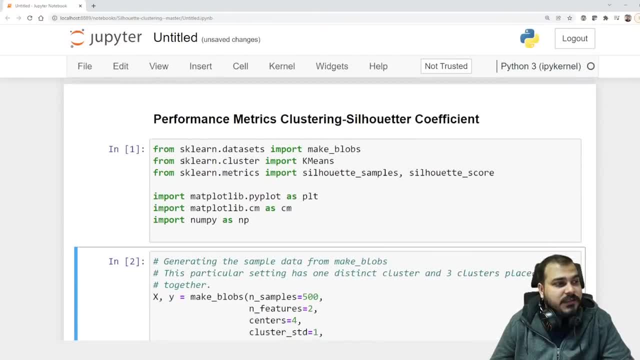 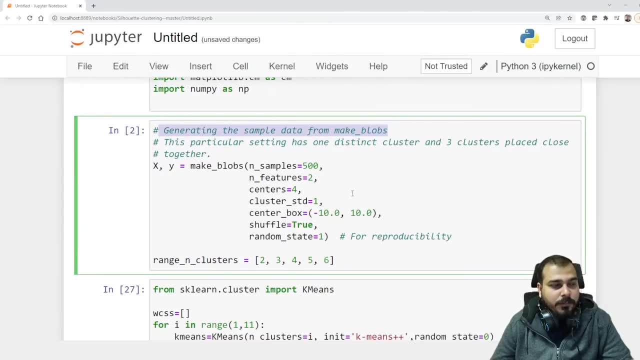 and all okay. so here we are executing it perfectly. the next thing is that here. the next thing is that we are trying to import the k-means clustering model and we are trying to generate the sample data from make underscore blobs. first of all, we are just trying to generate 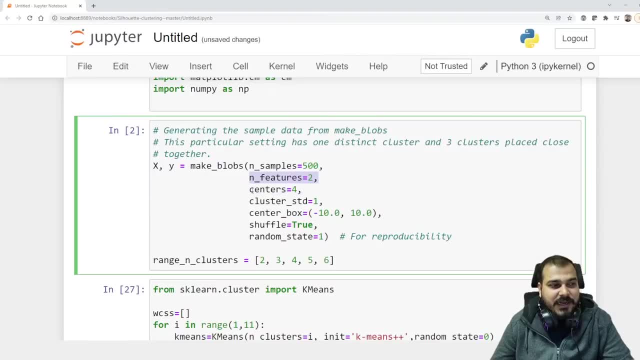 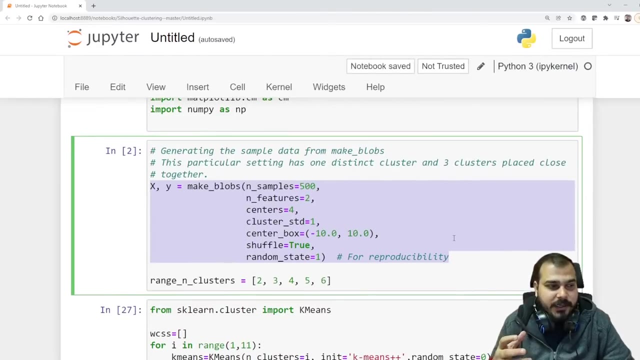 some samples with some two features and we are saying that, okay, it should have four centroids, or see centroids itself with some features. i'm trying to generate some x and y data randomly, okay, and this particular data set will basically be used in performing clustering algorithms. okay, forget. 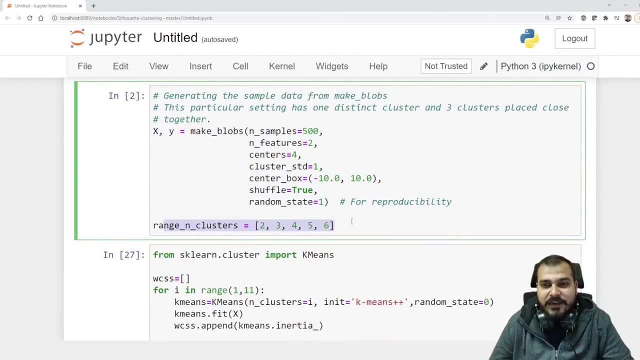 about range underscore, n underscore clusters, because we need to try with different different clusters and try to find out how to do that. so we are just trying to generate some samples with these two features and try to find out the silhouette score. so right now i've just 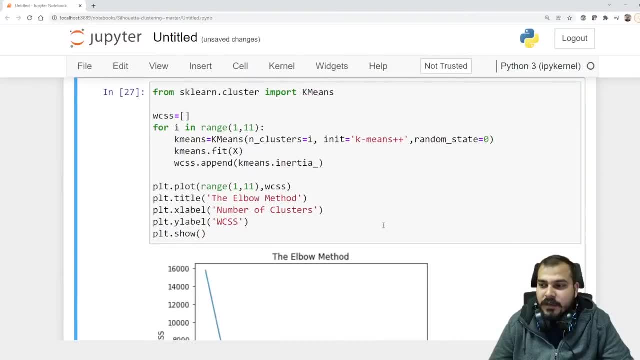 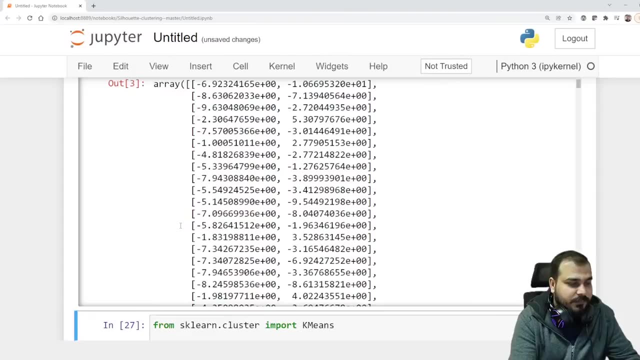 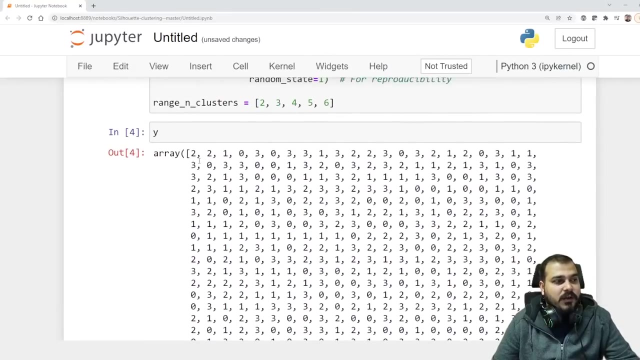 initialized with two, three, four, five, six values. okay, so it is very simple. so if i go and probably see my x data, so my x data will look something like this. so this is my x data with two features and this is my y data with one feature, which is my output, which belongs to a specific class. 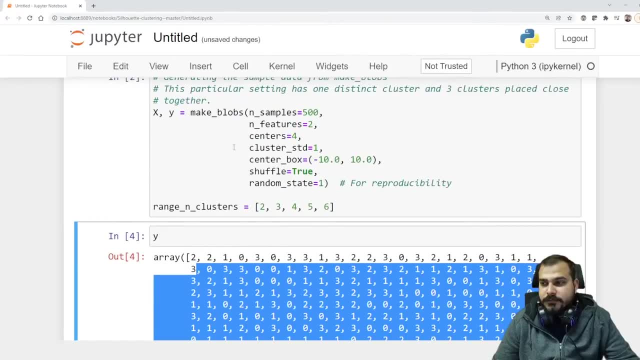 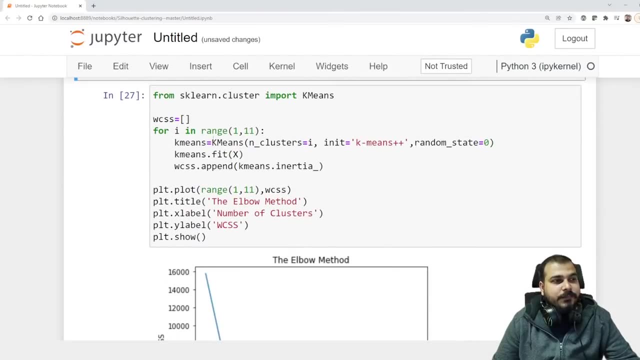 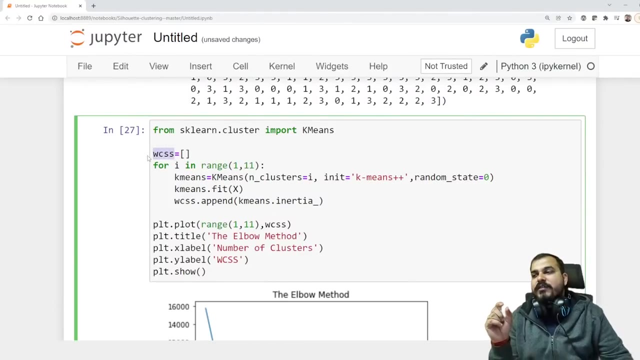 okay, so that you can actually do with the help of make underscore blobs. okay, now let's say how to apply k-means clustering algorithm. so, as i said that i will be using wcss- wcss basically means within cluster sum of square, so i'm going to import k-means over here for i in. 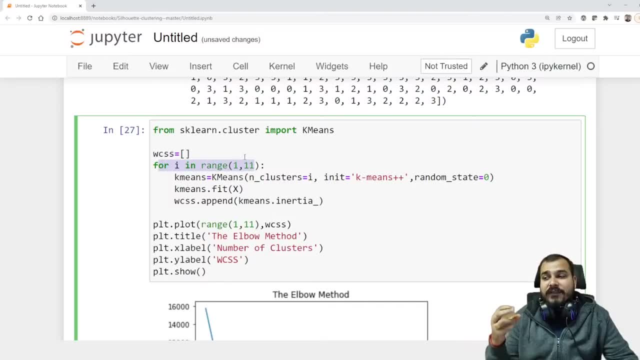 range 1 comma 11. that basically means i'm going to use different different k values or centroid values and try to see which is having the minimal wcss value and i'll try to draw that graph which i had actually shown you with respect to elbow method. so here i will basically be also using 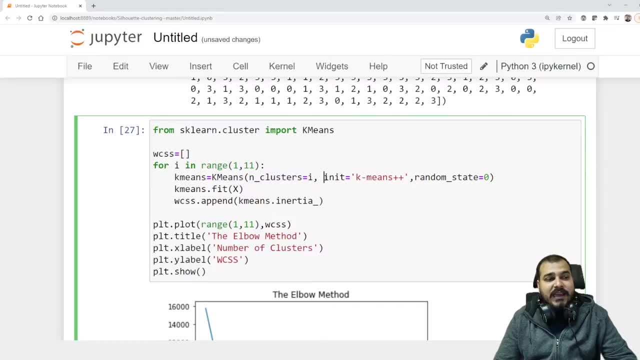 k-means, number of clusters will be i and initialization technique: i will be using k-means plus plus, so that the points, the centroids that are initialized, those, those points are very, very far okay, and then you have random. state is equal to zero, then we do fit and finally we do wcss dot. 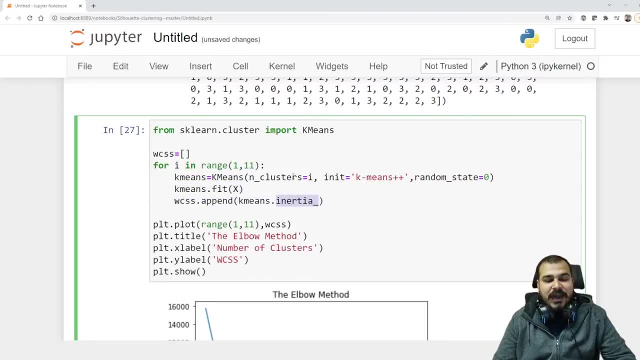 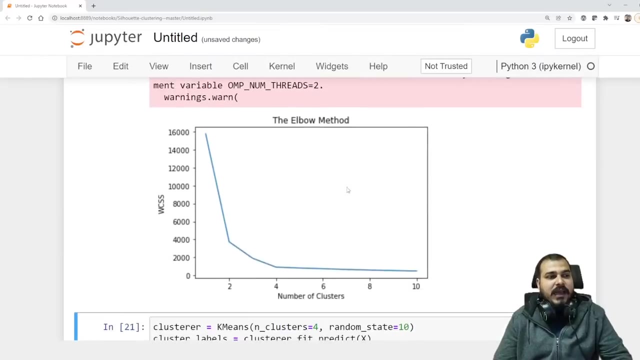 append k-means dot inertia. okay, this dot inertia will give you the distance between the centroids and all the other points. okay, and this is what i'm going to append in this wcss value. and finally, i'll just plot it now. here you can see that i'm just plotting it. 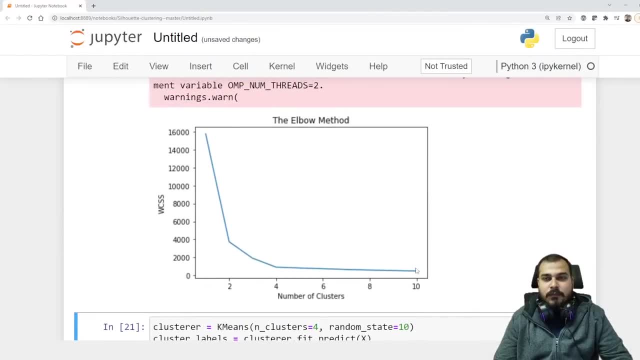 obviously, by seeing this graph, this graph looks like an elbow. okay, this graph looks like an elbow. so the point that i'm actually going to consider over here, see, which is the last abrupt change. so if i talk about the last abrupt change here, i have the specific value with respect to this. 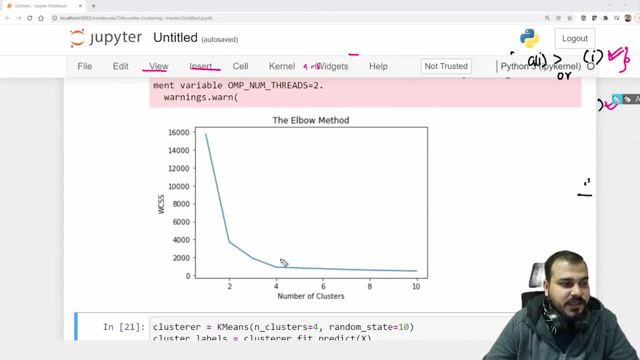 okay, i have one specific value with respect to this. this is my abrupt change from here. the changes are normal, so i'm going to basically select. k is equal to four. now what i'm actually going to do, with the help of selhout- i hope, i'm sorry- with the help of 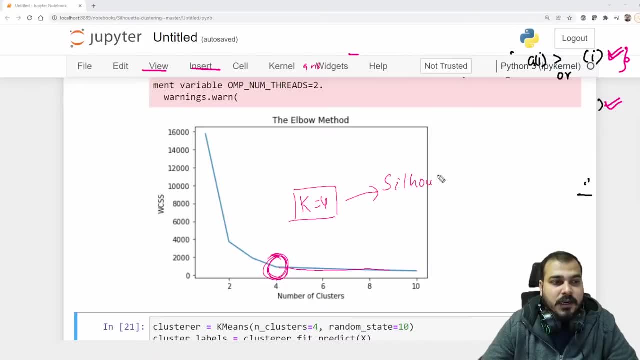 selhout plus score. we are going to compare whether k is equal to four is valid or not. so that is what we are going to do. okay, valid or not? so here we are going to do this. okay, now let's go ahead and let's try to see it how we are going to do it. so here you can see n. 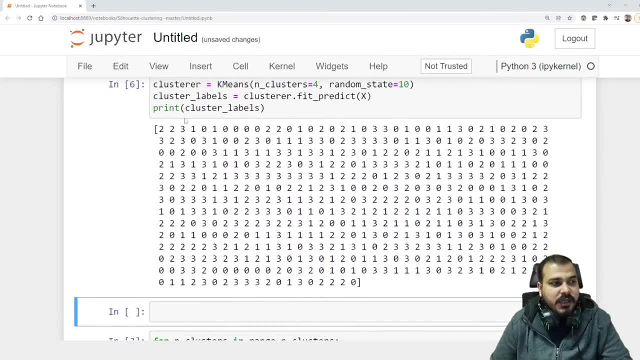 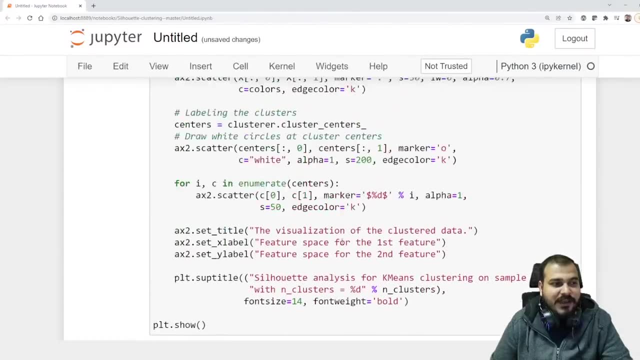 clusters equal to four, then i'm actually able to find out the prediction, and this is specifically my output. okay, this is done. now see this code. okay, this code is a huge code. i have actually taken this code directly from the sk learn page of selhout. okay, 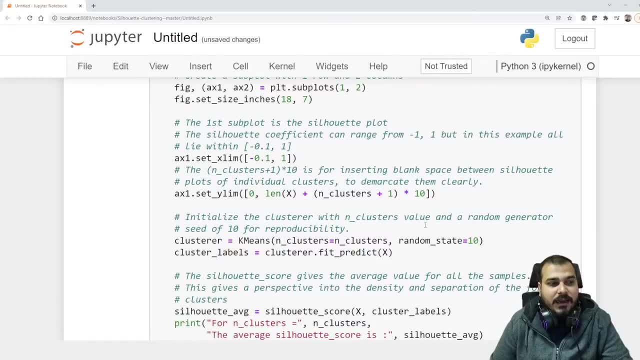 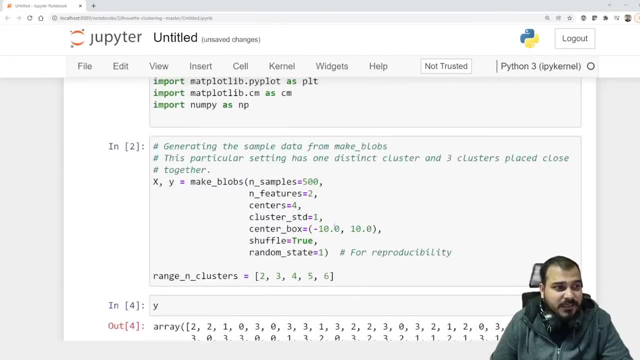 if you go and see this, this code is directly given over there. but i'm just going to talk about, like, what are the important things we need to see over here with respect to different, different clusters? see, see this: clusters two, three, four, five, six. i'm going to basically compare whether. 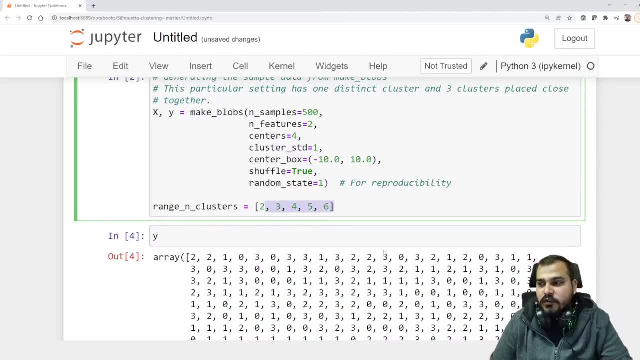 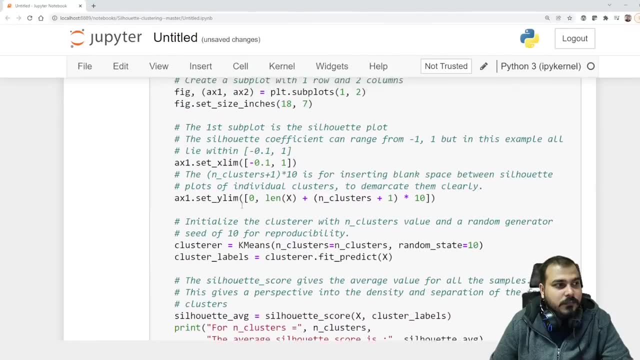 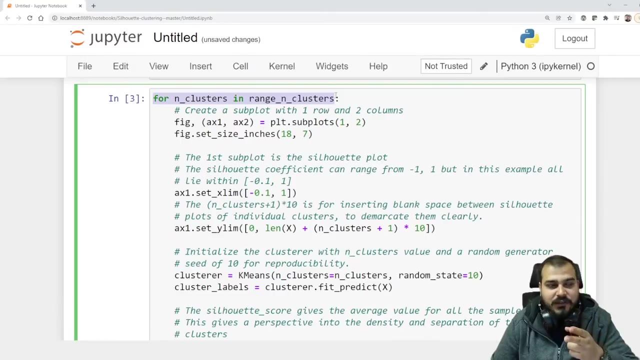 the k value should be four or not, with the help of selhout scoring. okay, so let's go here, and here you can see that i'm applying this one first. i will go with respect to four for n underscore clusters. in range underscore clusters, different different cluster values are: 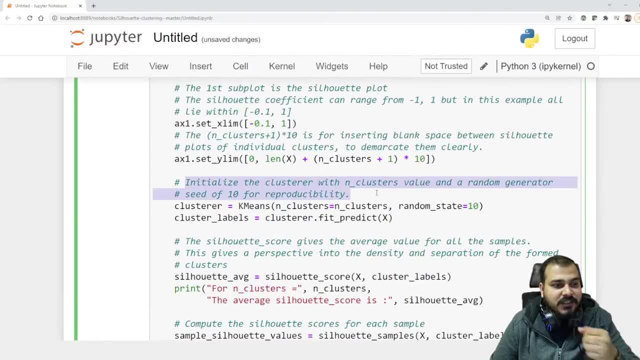 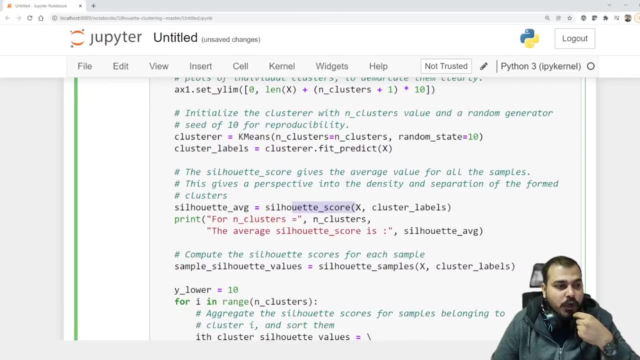 there. first we'll start with two. so here you can see, initialize the cluster with n cluster value and a random generator seed of 10 for reproducibility. so n underscore clusters. first i take, took it as two and then i did fit predict on x. after i did fit predict on x, i am using this score. 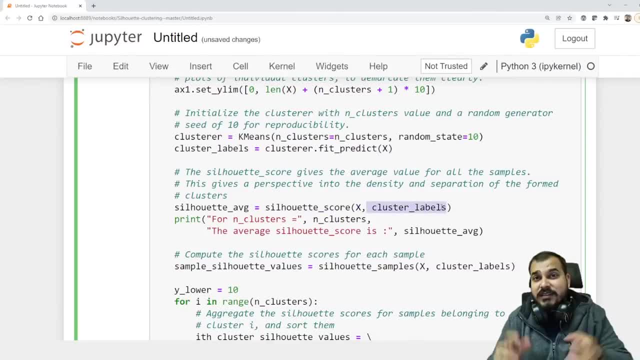 on x comma cluster label. now what this is going to do. understand in selhout. what did we discuss? we discussed that. what did we discuss? it will. it will try to find out all the clusters, the clusters over here, like this, and it will try to calculate the distance between them, which is the a of i. then it will try. 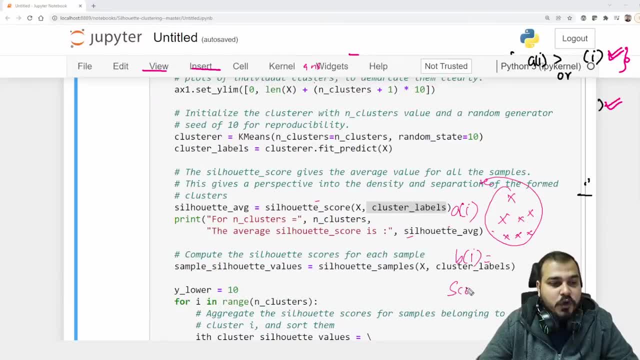 to compute the b of i. then, finally, it will try to compute the score and if the value is between minus one to plus one, the more the value is towards plus one, the more better it is right. so this, all things we have already discussed, and that is what this specific function will do. 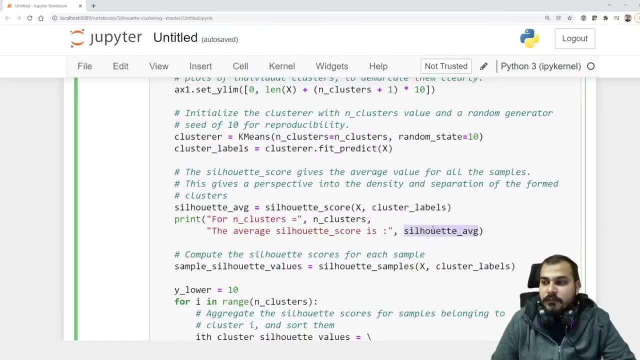 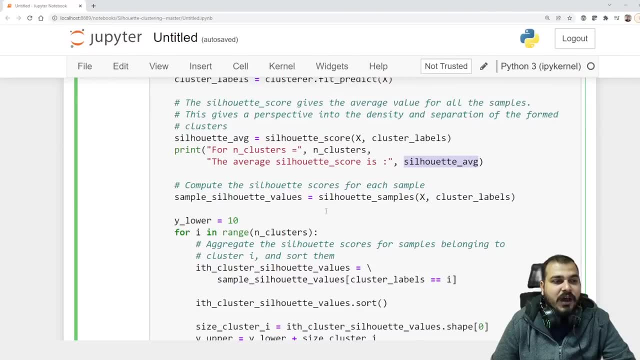 and this will give my selhout average value over here. okay, selhout value will be over here. okay, this we have done and then we can continuously do it for another another things you can actually find it over here, and this value that you see, this code. 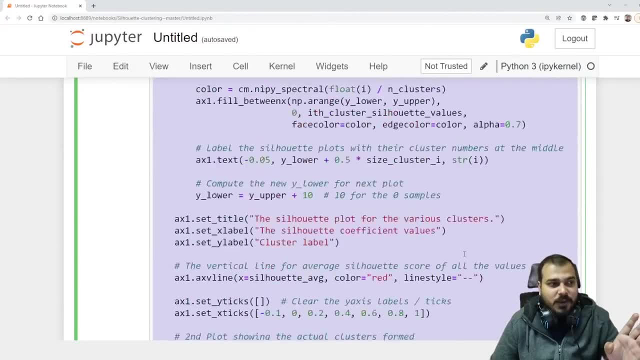 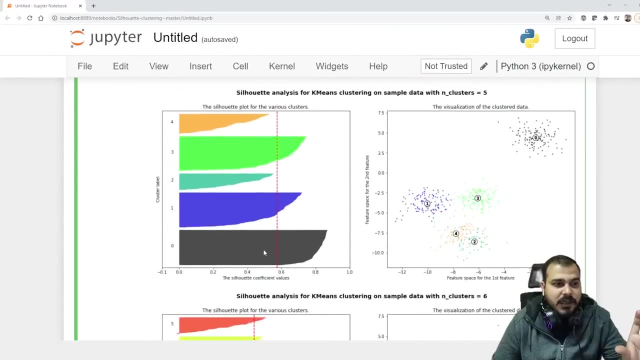 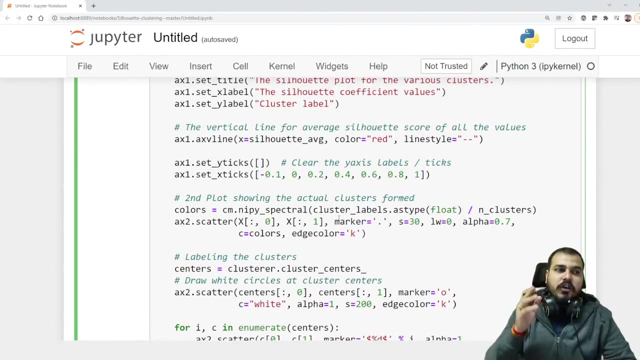 that, you see, is nothing so complex. okay, this is just to display the data properly in the form of graphs. okay, in the form of graphs. so again, i'm telling you, i did not write this code, i've directly taken it from the uh sklearn page of selhout. okay, so just try to see this particular uh plotting diagrams and all that. 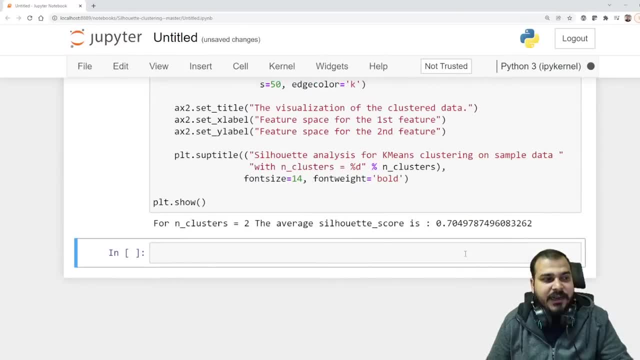 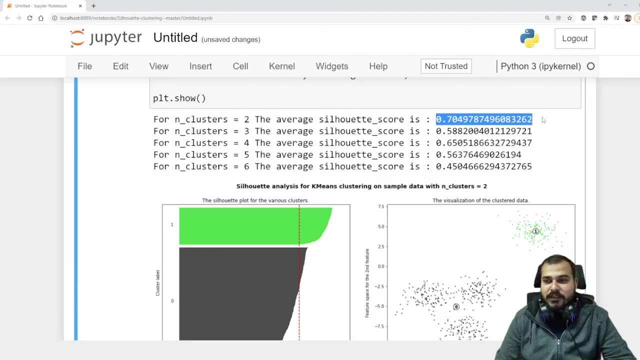 you can definitely figure out, but let's see. i will try to execute it and try to find out. the output now, see for n: underscore cluster is equal to two. the average selhout score is 0.70. i told you the value will be between minus one to plus one, and i'm actually getting 0.704, which is very, very good. 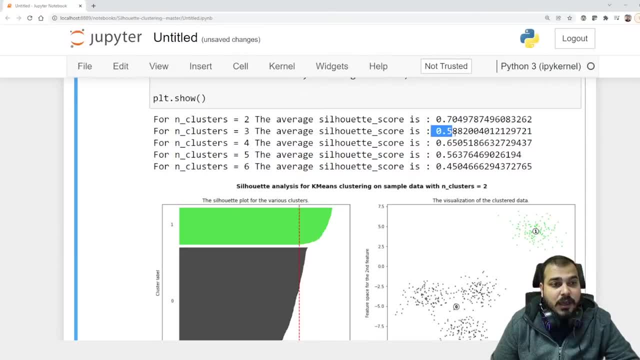 okay. and then for n underscore cluster is equal to three point five eight, eight. then n underscore cluster is equal to four. i'm getting 0.65, which is pretty much amazing. and then for n underscore cluster is equal to five, the average score is 0.563 and n underscore cluster is equal to six. 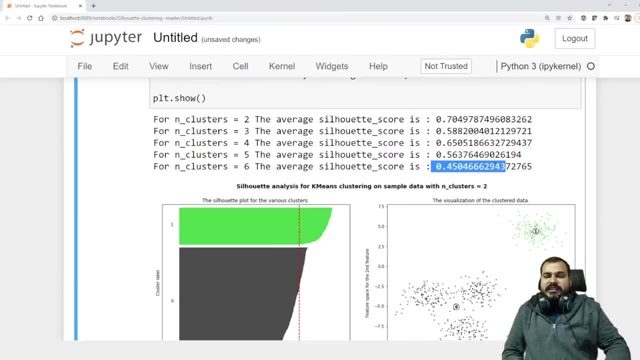 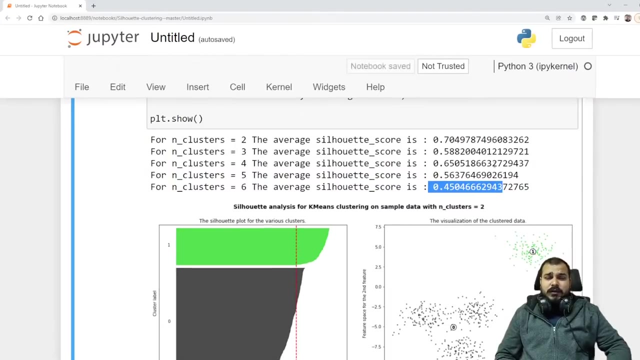 you are saying 0.45 here directly. you can actually say that, fine for n. underscore cluster is equal to two. i'm getting an amazing score of 0.704. okay, obviously you're. you're getting the highest value over this. so should we select n? underscore cluster is equal to two, should we? okay, we should not. 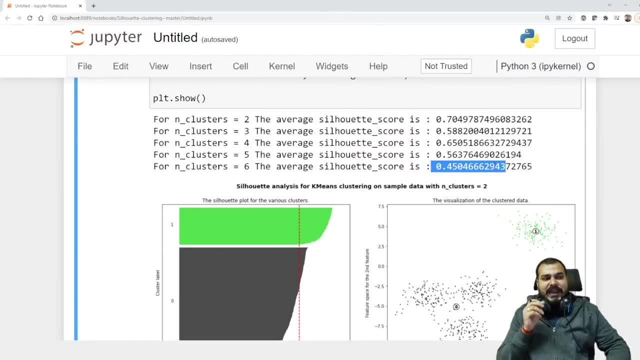 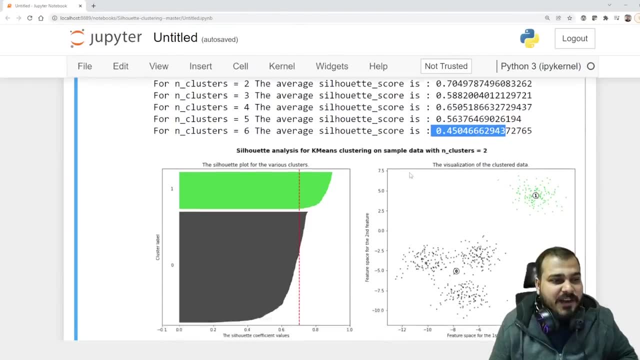 directly conclude from it, because here we need to also see that any feature value or any cluster value is also coming as negative value. that also we need to check. so here we will go down over here. you will see the first one over here. with respect to the first one, you see that i'm getting the 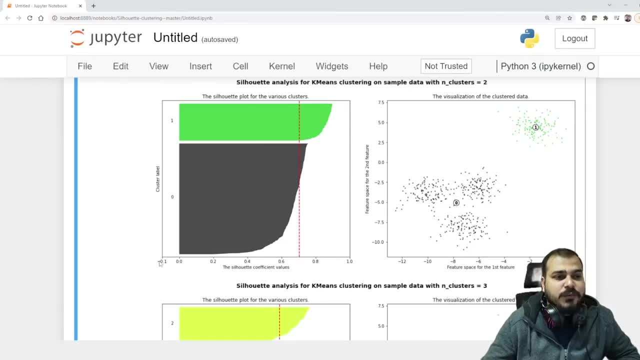 value from zero to one. it is not going to minus 0.1, so definitely two clusters was able to solve the problem, so i'll keep it like this with me. i definitely have a chance that this may this may be able to solve the problem, so i'll keep it like this with me. i definitely have a chance. 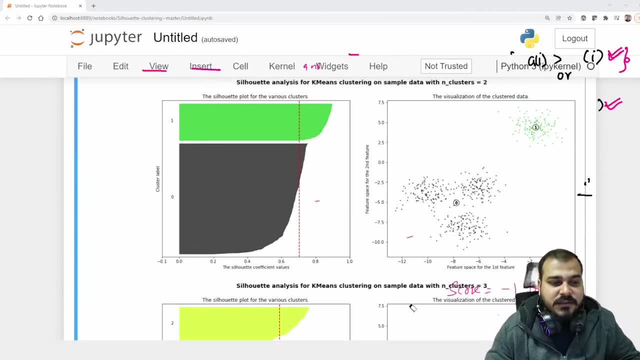 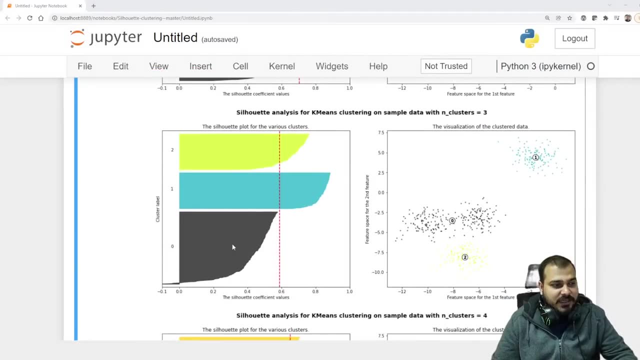 that this may perform well. i may have a chance that this, this, this k, k is equal to two- may perform well. okay, so i may have a chance. let's see through the next one to the next one over here. you can see that for one of the cluster, the value is negative. if the value is negative, that basically means the 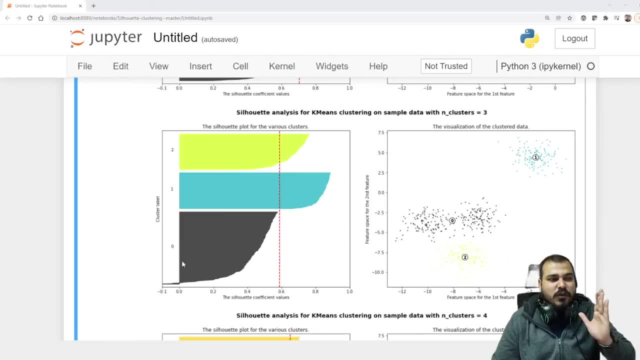 ai is obviously greater than b of i, so i'm not going to refer this because it is having some negative values, even though my cluster looks better. but again, understand what is the problem with respect to this cluster and i'm not going to refer this because it is having some negative. 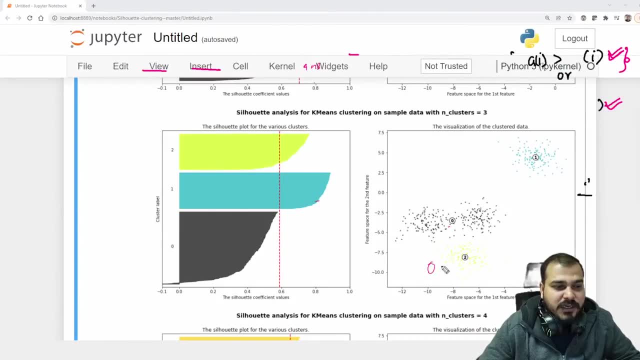 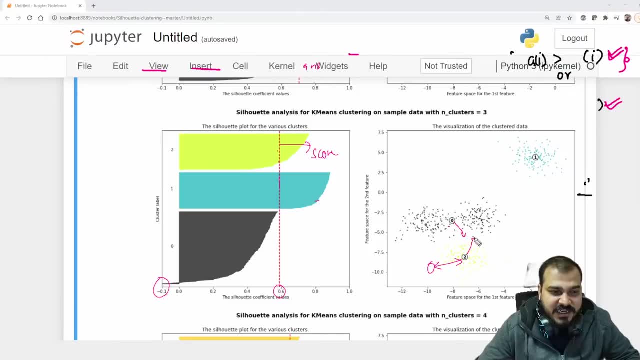 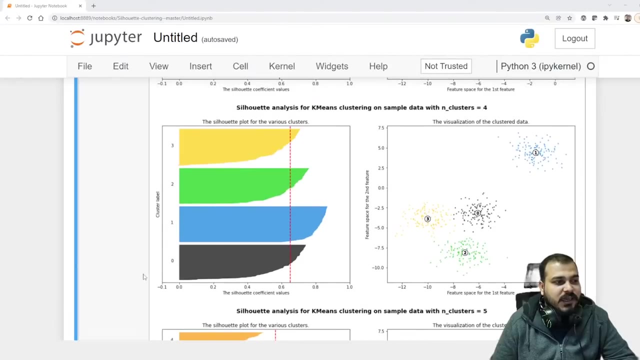 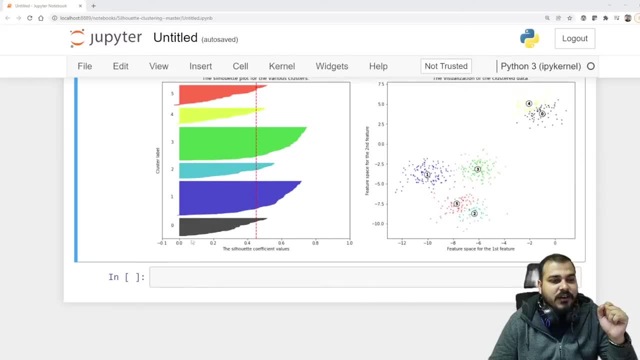 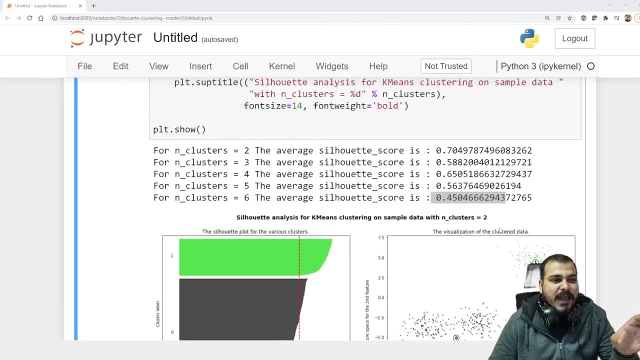 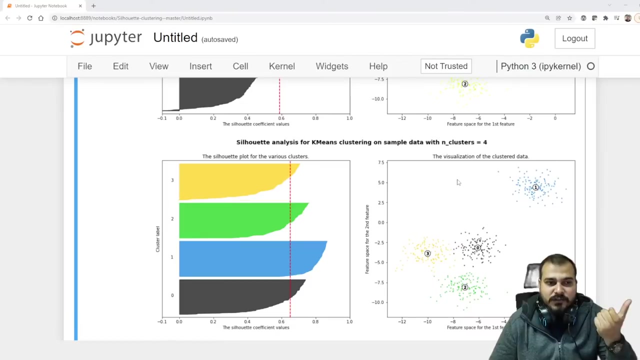 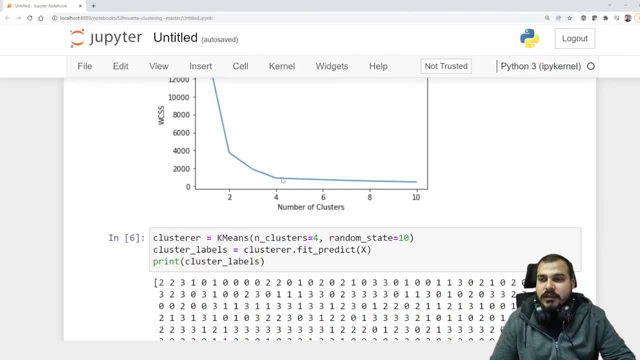 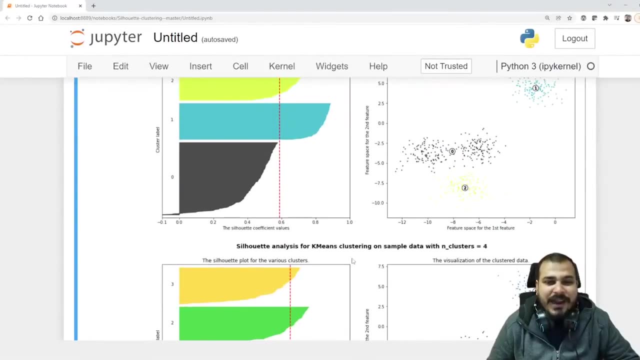 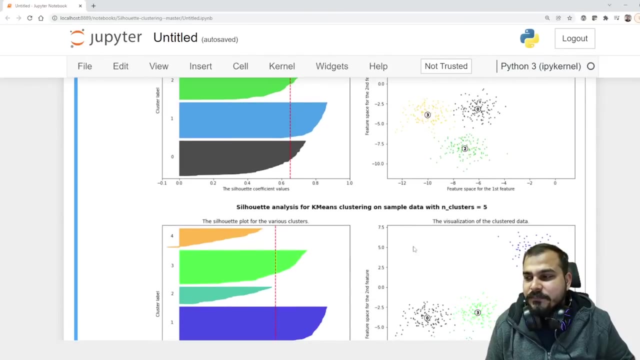 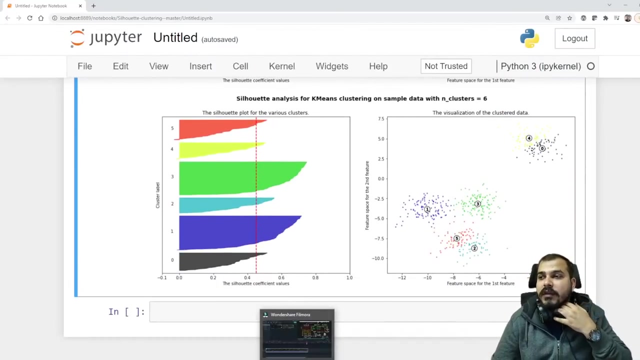 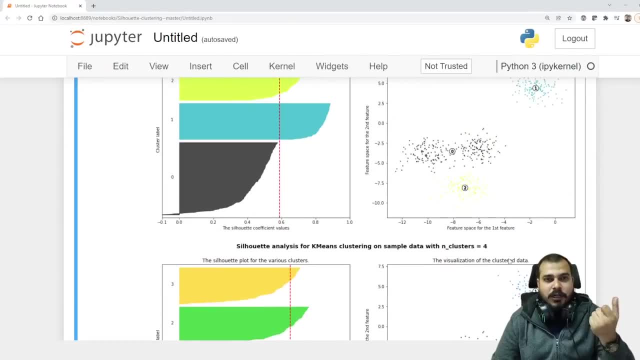 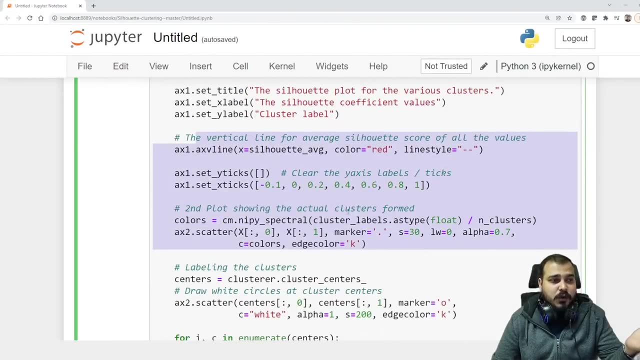 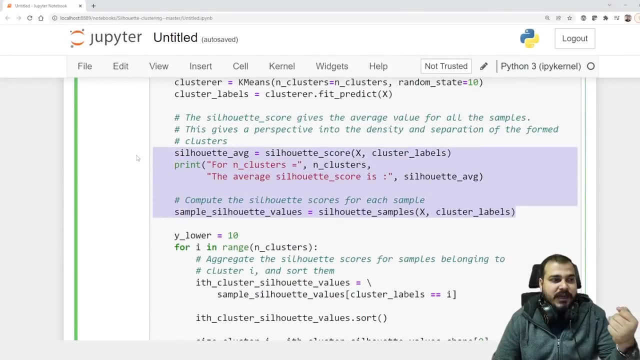 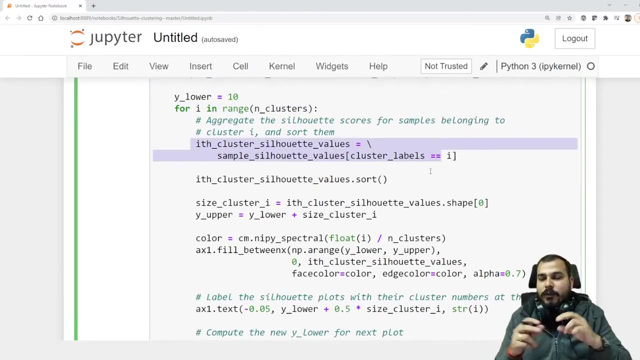 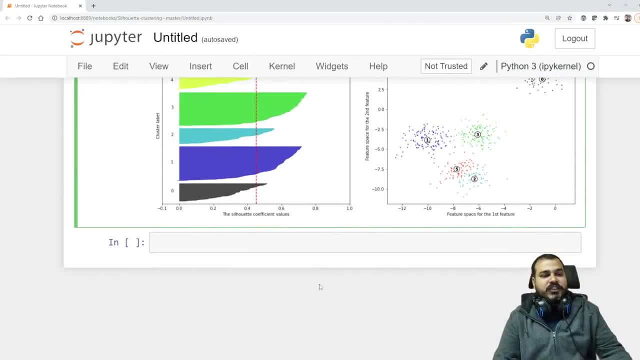 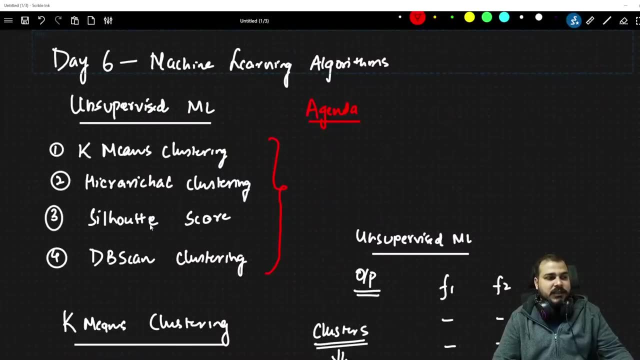 so this was the session and, yes, in today's session we efficiently covered many topics. we covered k-means, hierarchical clustering, siloids, code dbk and clustering. in tomorrow's session, the topics that are probably pending is: first, i'll start with svm and svr. second, i will go ahead with 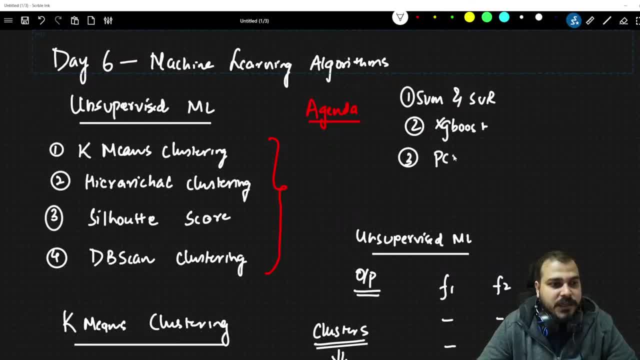 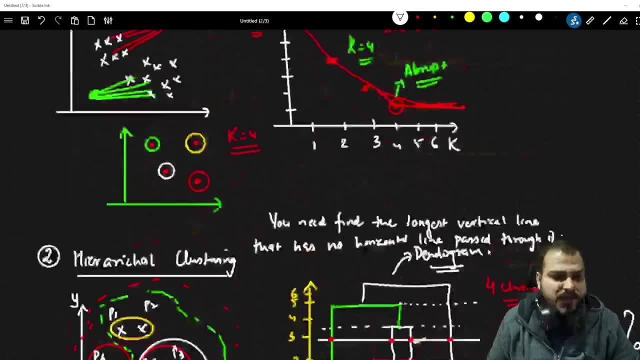 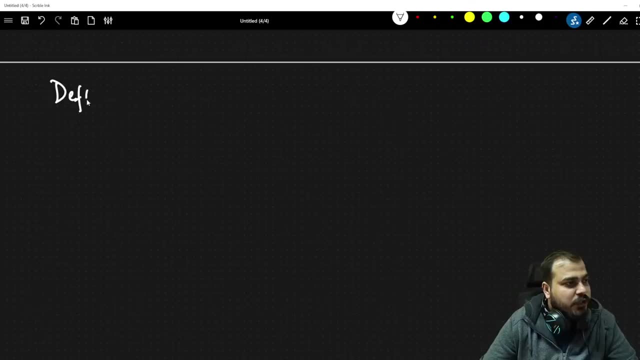 xg boost. and third, i will cover up pca. let's see whether i'll be able to complete this session. uh, one, one amazing thing that i want to teach you guys, because many people ask me the definition of bias and variance. definition of bias and variance. so let's should i explain this. 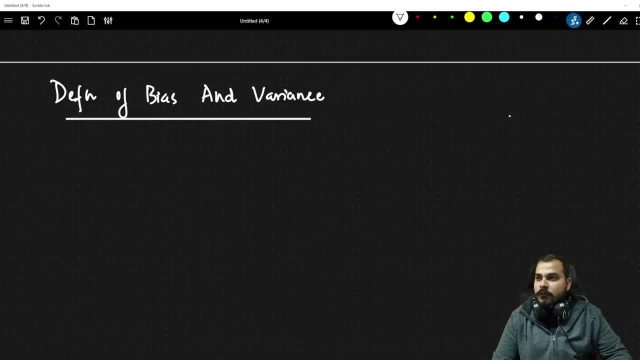 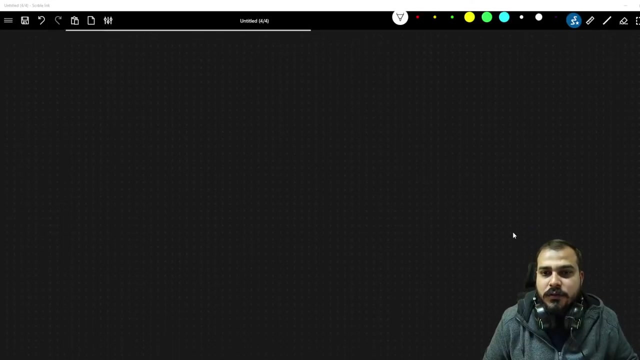 everyone. just let me know. should i explain this, it's okay. who have not understood? please revise the session, okay? so let's go ahead and let me do one thing i will also do. one good thing in this is that here we are going to understand about definition of bias and variance. 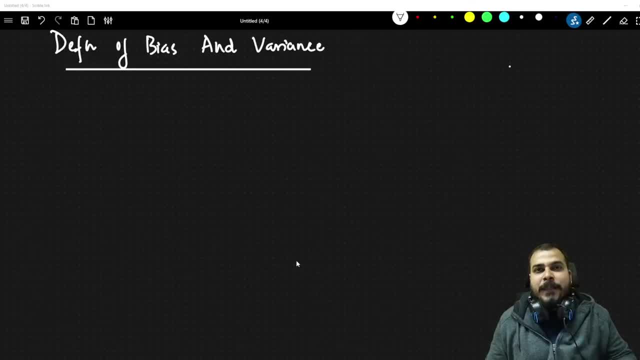 okay, let's understand. so, guys, many people get confused when we talk about bias and variance. so let's go ahead and let me do one thing i will also do. one good thing in this is that here we are going to do one thing about bias and variance, you know, because let's say that, uh, i have a model for the. 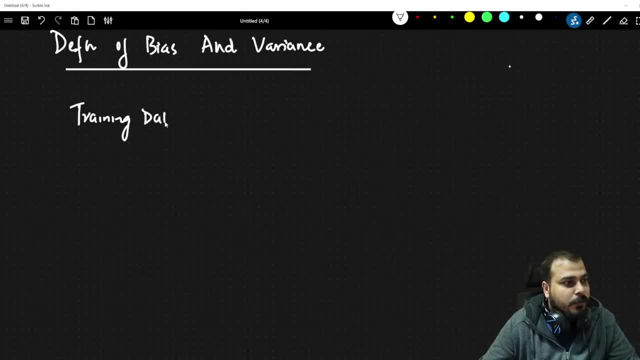 training data set. for the training data set, it gives us somewhere around 90 accuracy. let's say i'm getting a 90 accuracy. for the test data, i may probably getting somewhere around 70 accuracy. now tell me which scenario is basically this? most of the people will be saying that okay, fine, it is. 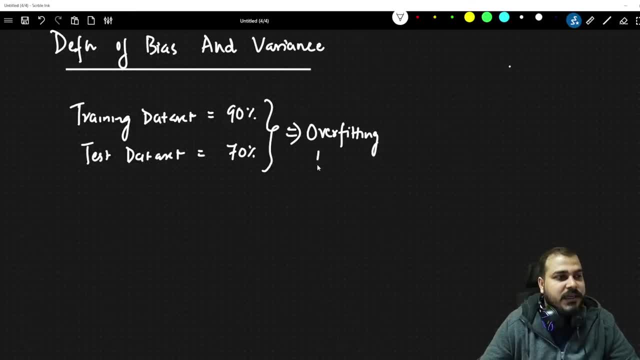 overfitting. now, when i say overfitting, i basically mention overfitting by low bias and high variance, right? so many people get confused. krish, tell me just the exact definition of bias and variance. low bias: obviously you are saying that because the training is. 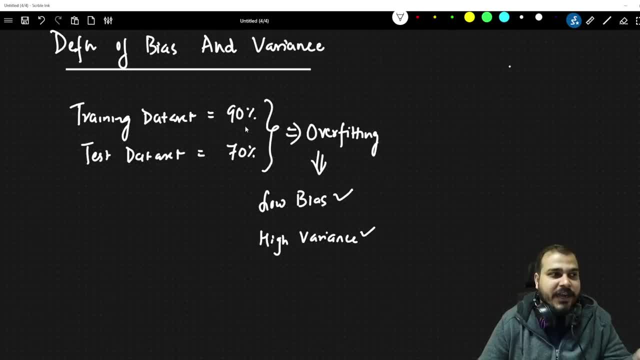 performed like. the model is performing well with the help of training data set, but with respect to the test data set, the model is not performing well. with respect to training data set, why do we always say bias? and with respect to test data set, why do we always say variance? okay, so for this. 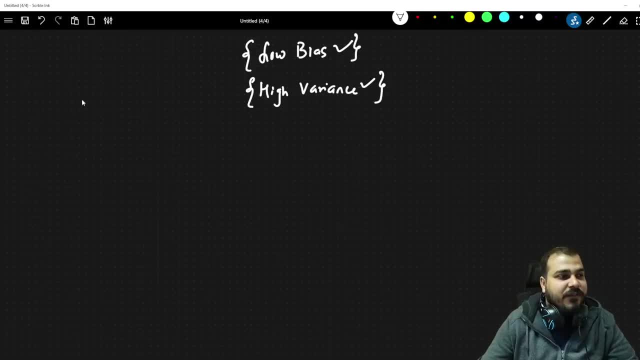 you need to understand the definition of bias. so let me write down the definition of bias over here. so here i we can definitely write that bias it is a phenomena. it is a phenomena that skews, that skews the, the result of an algorithm in favor, in favor. 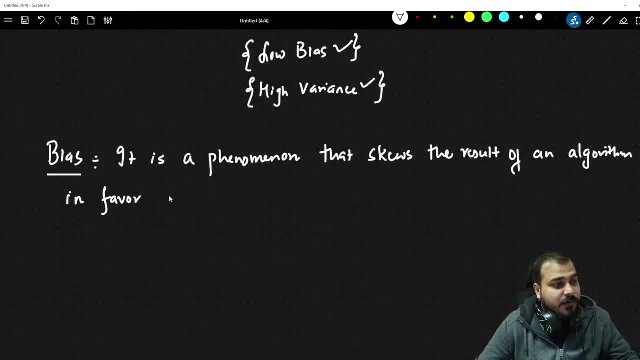 in favor or against an idea. against an idea, i'll make you understand the definition. uh uh, but understand the understand. understand what i have actually written over here. it is a phenomena that skews the result of an algorithm in favor or against an idea. whenever i say this specific. 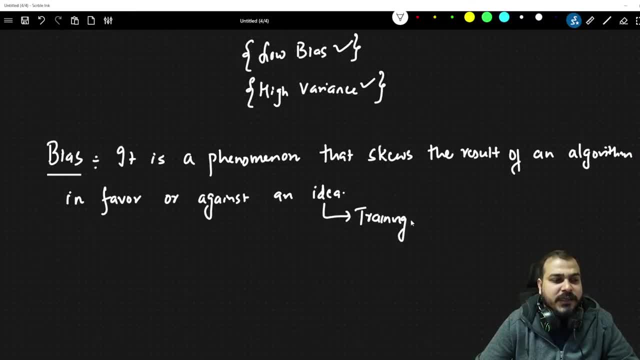 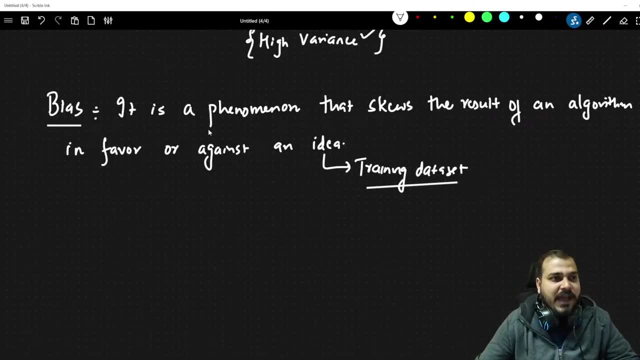 idea, this idea. i will just talk about the training data set initially. okay, training data set. now, when we train a specific model, suppose if i have this specific model over here and i'm training with specific training data set, so this is my training data set. training data set now based on the. 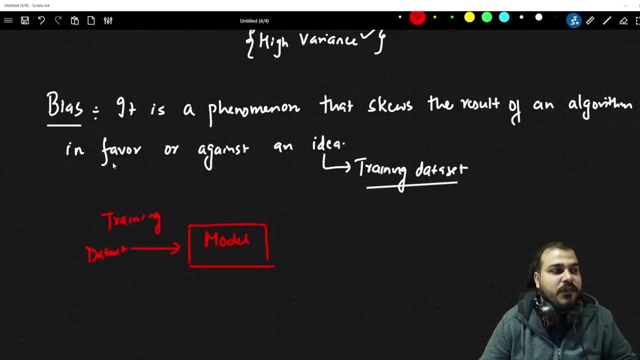 definition. what does it basically say? it is a phenomenon that skews the result of an algorithm in favor or against an idea or a this specific training data set. so, even though i am training this particular model with this training data set, with this data set, okay it may. it may be in favor. 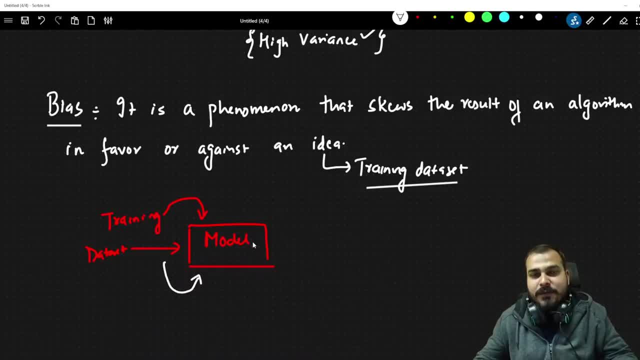 of that, or it may be against or that. that basically means it may perform well, it may not perform well. if it is not performing well, that basically means the accuracy is down right. if the accuracy is better at that point of time, what we'll say. see, if the accuracy is better that time, what we'll say. 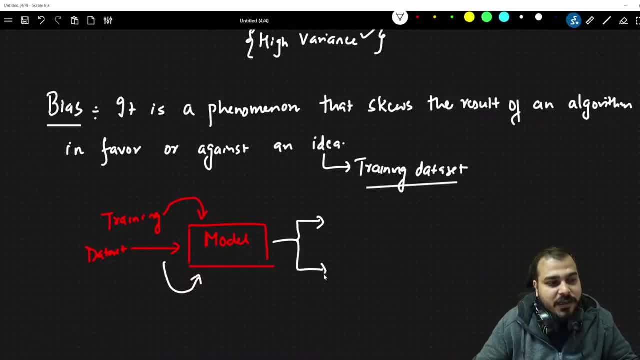 we'll come up with two terms from here. obviously you understand. okay, there are two scenarios of bias now here. if it is in favor, that basically means it is performing well. with respect to the training data set, i will basically say that it has high bias if it is not able to perform well. 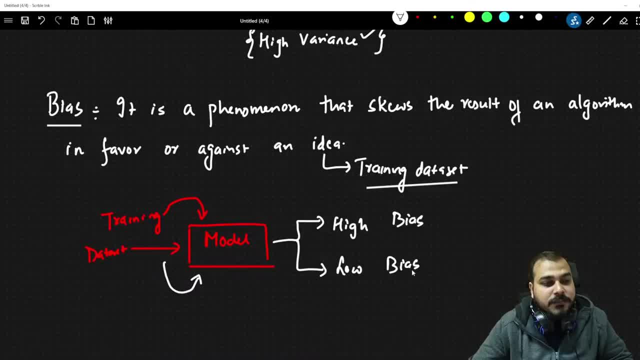 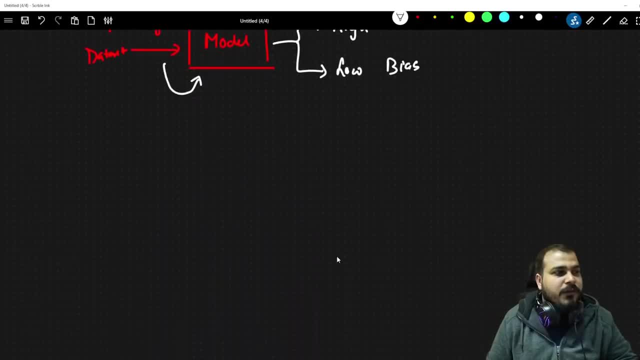 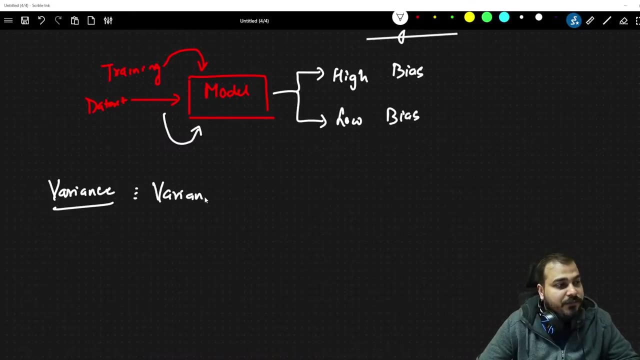 kind of confusion. okay now, similarly, if i talk about variance, let's say about variance, because you need to understand the definition. a definition is very much important. okay, if i? if i just talk about the definition of variance, i'm just going to refer like this: the variance refers to 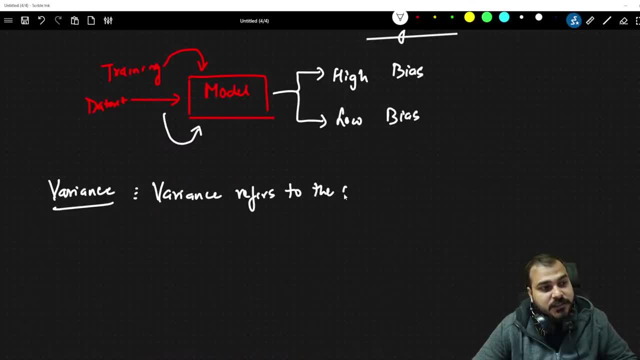 the changes in the model when using different- when using different portion of the training or test data. now let's understand this particular definition. variance refers to the changes in the model when using different proportion of the test training data or test data when using different proportion of the. 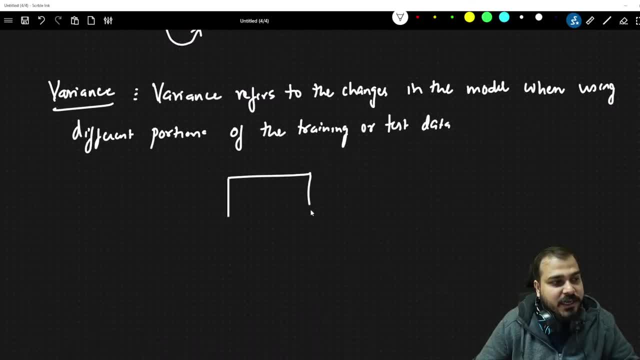 test data. we obviously know that whenever, initially, if i have a model, understand from the definition, everything will make sense. i am basically training initially with the training data. okay, because we divide our data set. see our data set whenever we are working with. we divide this into two parts. one is our train data and test data. okay, because this is a test. data is a part. 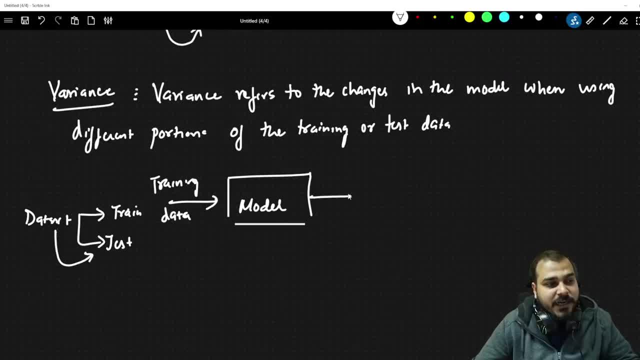 of that particular data set right and suppose in this particular training data. it gets to crazy like, therefore, because in this particular course, if any stage i am, basicallyrooms, data is the training data for underographics, the view of the model, and there aresoci Vegeta. 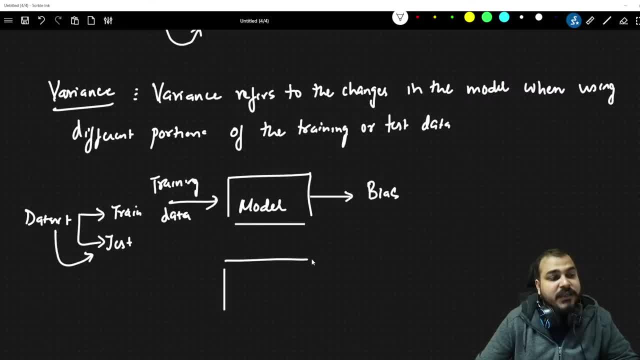 coma to the sets of быстро test probes. okay, because actuallyregister was trained and performed as well. here i'm actually talking about biased. but when we come with respect to the prediction of this specific model, at that point of time i can use other training data. that basically. 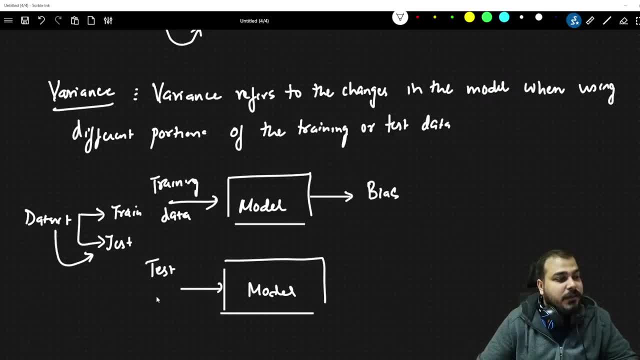 training data may not be a lot, or i can also use test data. now, in this test data, what we do do some kind of predictions. these are my predictions and in this prediction again i may get two scenario. i may get to scenario which is basicallyemensionbij variance refers. 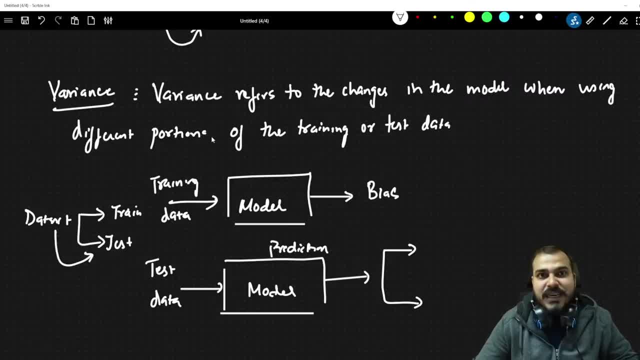 to the changes i can imagine. often you can see a few on one. one can say sorry, but we will see at two. i don't think we can end at two scenario, which is basically mentioned by variance. it refers to the changes we make in the model when using, when using different portion of the training or test data. refers to 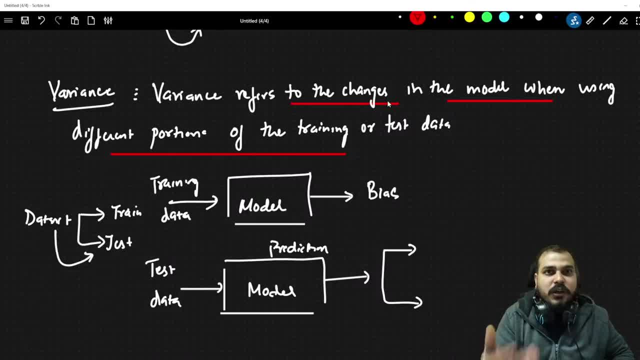 the changes basically means whether it is able to give a good prediction or wrong predictions. that's it so in this particular scenario. if it gives a good prediction, i may definitely say it as low variance. that basically means the accuracy with the accuracy with respect to the test data. 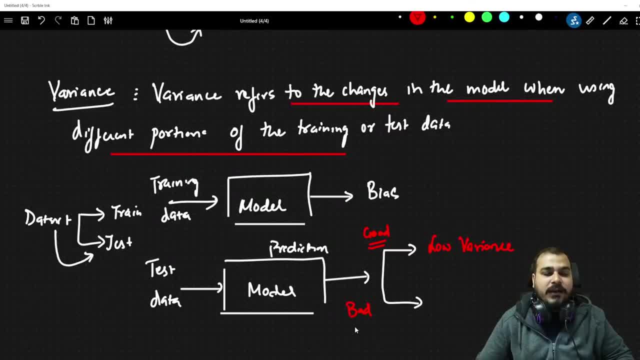 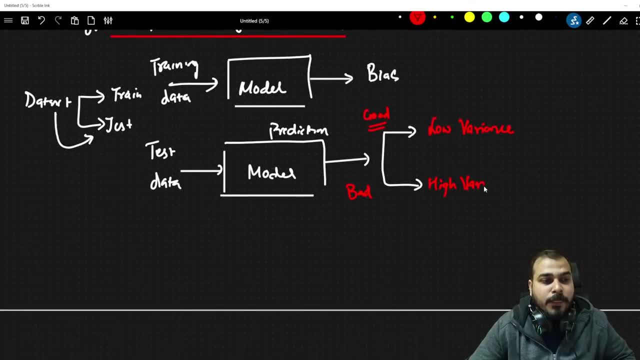 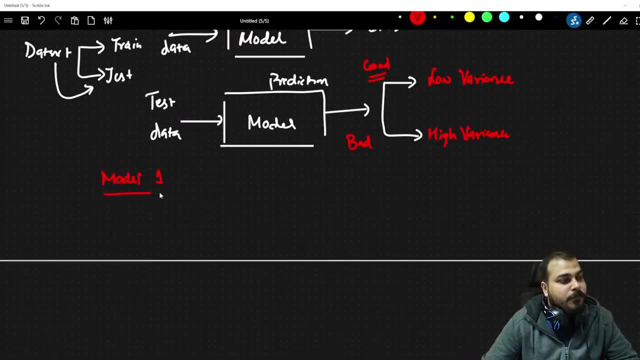 is also very good if i probably get a bad, if i probably get a bad accuracy at that time, i basically say it as high variance. so if i talk about three scenarios over here, let's say this is my model one and this is my model two and this is my model three. now, in this scenario, 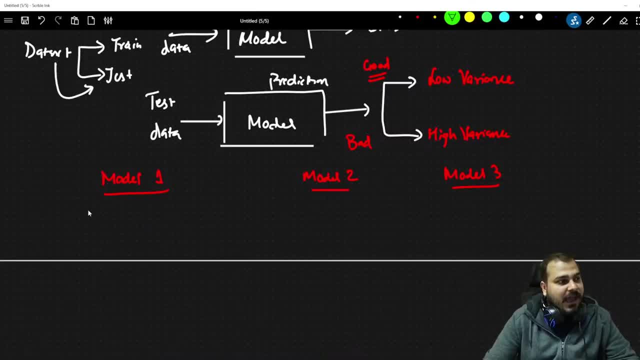 let's consider that my model one has the training accuracy of 90 and test accuracy of 75. similarly, i have here as my train accuracy of 60 percent and my test accuracy of 55 percent now. similarly, if i have my train accuracy of 90 percent and my test accuracy of 92 percent, now tell me what, what things you will be getting. 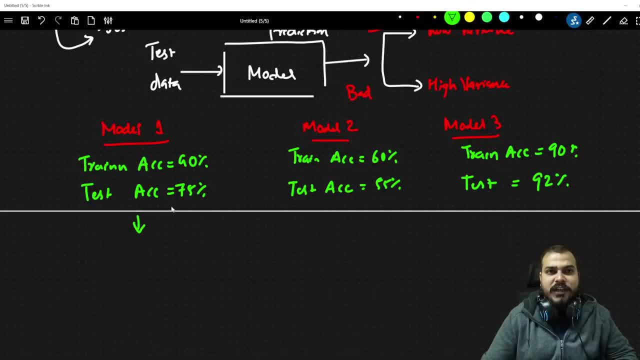 you Here. obviously you can directly say that: fine, your training accuracy is better. now you are talking about bias, so this basically indicates that this has low bias and since your test accuracy is bad because it is when compared to the training accuracy, it 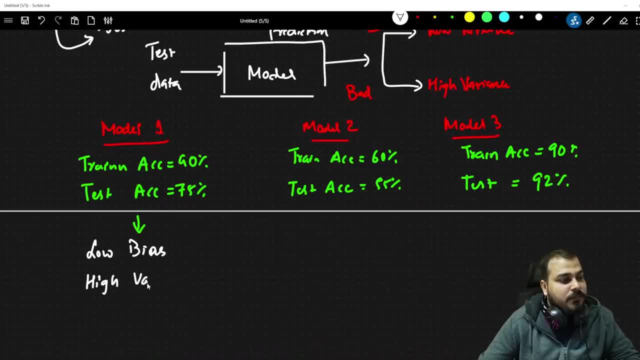 is less so. here you are basically going to say high variance. Understand, with respect to the definition, similarly over here, what you will say: High bias, high variance, because obviously it is not performing well. This is the another scenario. last, the last scenario is that this is the scenario that 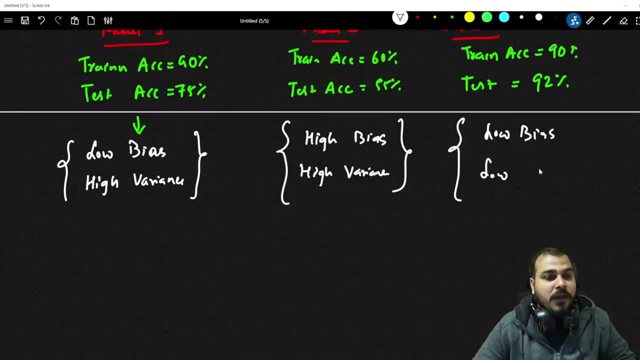 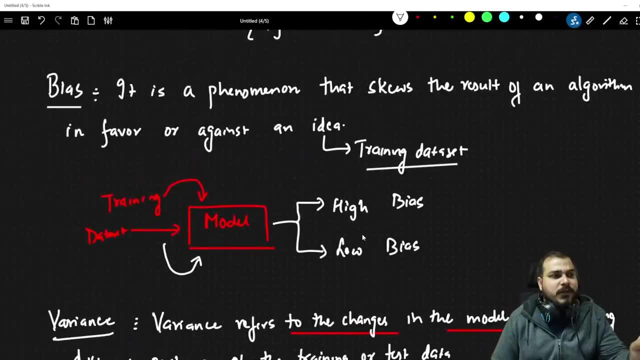 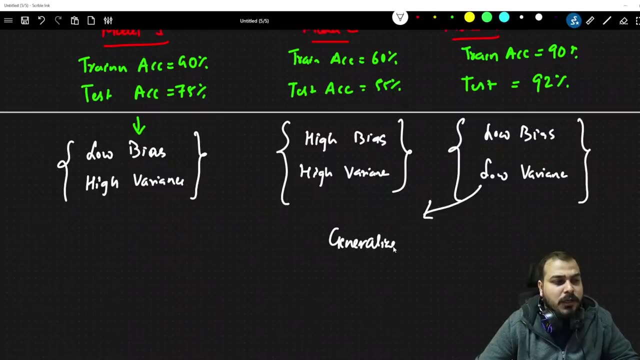 we want because it is low bias and low variance. ok, Many, many people have basically asked me the definition with respect to bias and variance and here I have actually discussed and this indicates this gives me a generalized model and this is what is our aim when we are working as a data scientist. 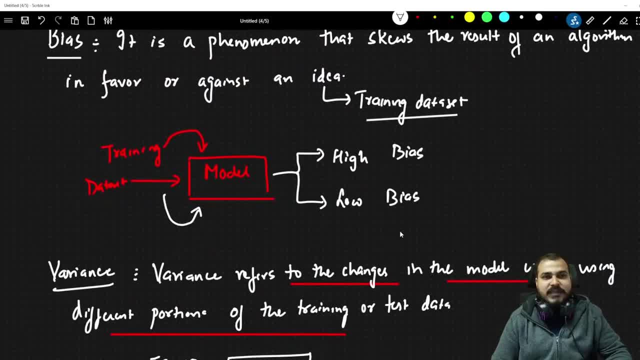 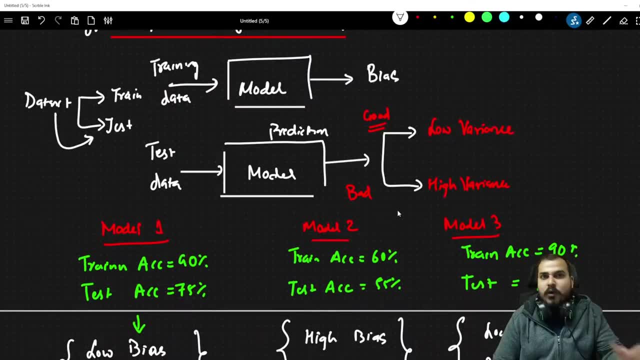 So I hope you have understood the basic difference between variance, bias and variance, and I was able to give you lot of examples, lot of understanding with respect to this, so I hope you have actually got this particular understanding of this two terms which we 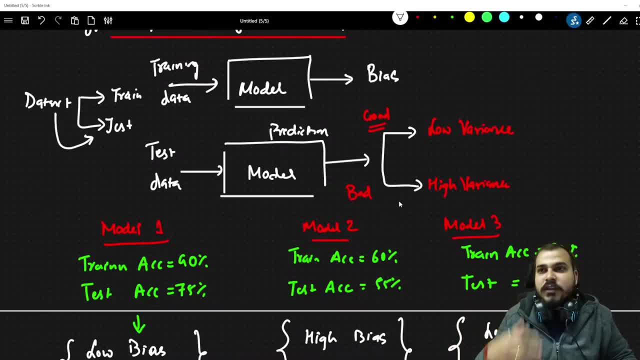 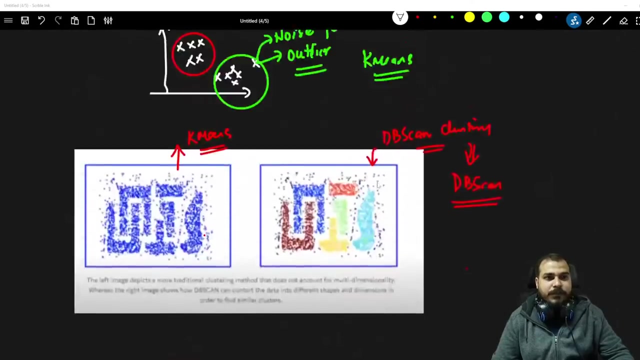 specifically talk about high bias, low bias, high variance, low variance, right? So this was it from my side, guys, Ok, And I hope you have understood this. So I hope you have understood. just give me a statement, something. so till when I can? avail tech neuron lifetime subscription. guys, get it within March. after that the price of the tech neuron is going to increase, Increase to 20,000, ok, And you will not be getting for lifetime their time. yearly for 3 years subscription.